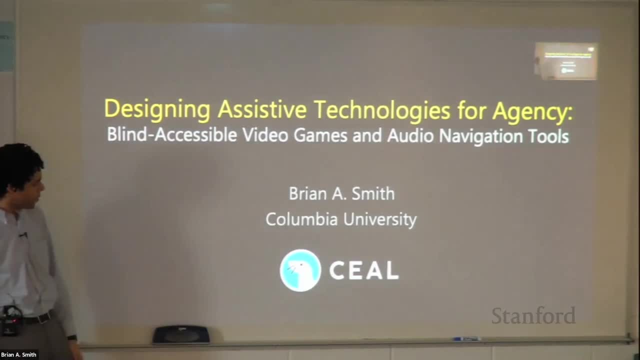 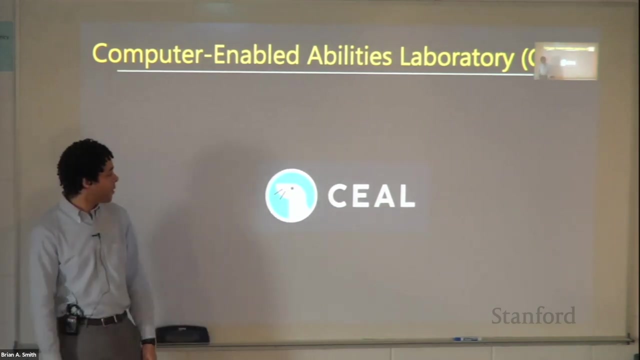 impairments. So my lab- Michael mentioned this already, but my lab- is the computer-enabled abilities lab. Let me just get my clicker on focus here. Here we go, Computer-enabled abilities lab, or SEAL for short, And we are looking to. you know the type of work that we do is we make it so that computers can grant. 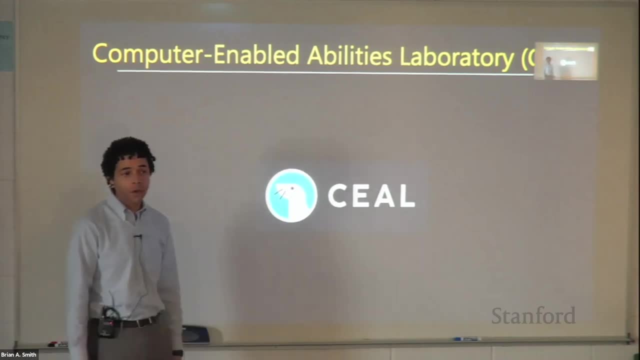 people, abilities, the ability to better experience the world, And so there are four threads of, I guess, skills that we employ in our research. One is accessibility, of course. Second is machine learning. We like to think about like, what does it mean, Like, how can you model experiences? so 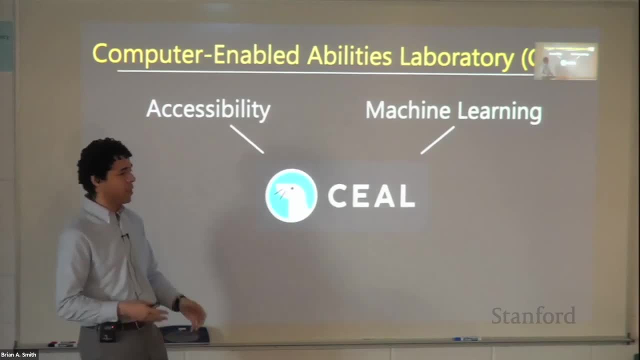 that you know that you know you can say definitively that one person is having an equivalent experience. We look at inputs, for example, controller inputs, VR, AR inputs, and how we can actually model those probabilistically. We look at games. We wear a game design hat quite often. 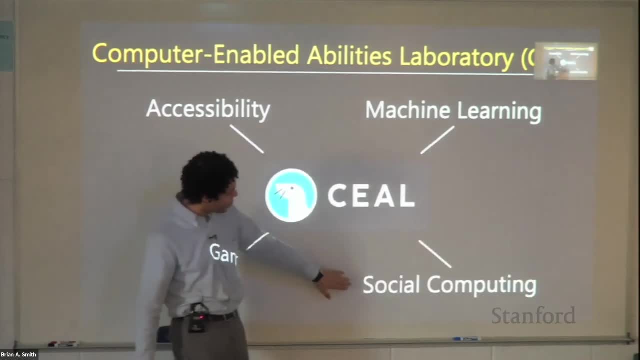 in our approaches, as you'll see here in this talk, And we do social computing work Quite often. if you ask people, you know visually impaired users, people with disabilities, you know just people in general. what do you like most value in life? They'll often 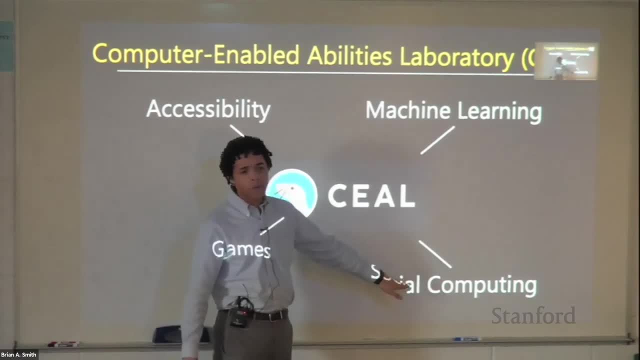 say, like other people, And so social computing is tremendously important. if you think about making technology grant people abilities- A lot of the work that I do at SNAP- I'm a research scientist there- SNAP, which makes Snapchat, is involved in social computing as well, And so 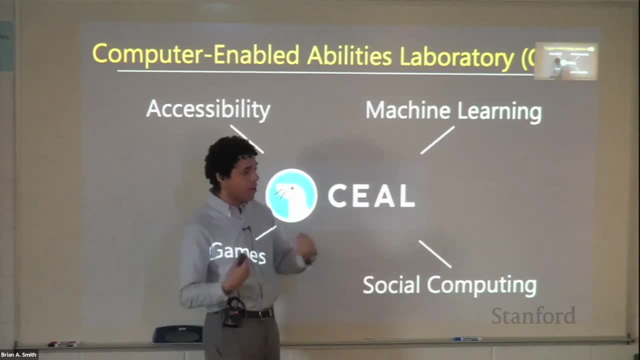 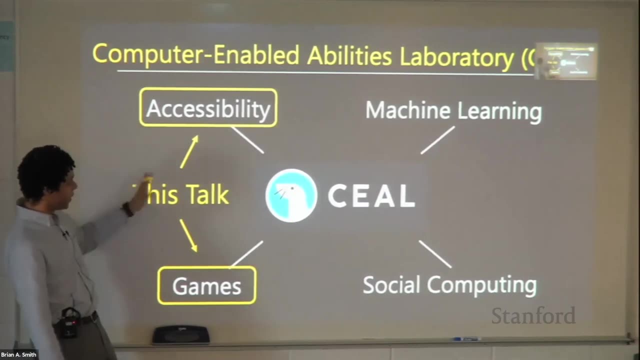 you'll see later. we're talking- you know we'll be talking- about maps and sharing maps. Social computing will come in. So this talk itself is really going to be focusing on the accessibility angle and the games and how and the mix between the two. 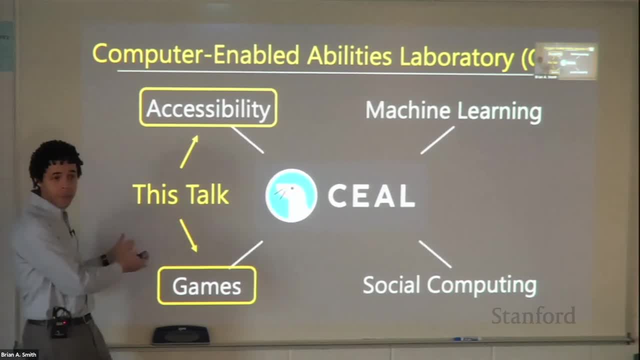 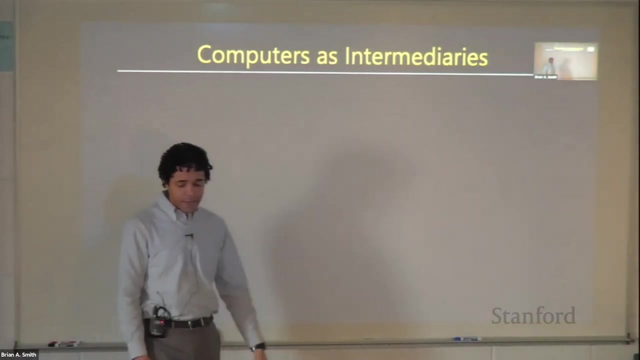 As I mentioned before, we're going to be looking at digital spaces first, and how we can make digital spaces equivalently accessible, And then that those principles will inform our treatment of physical spaces, the real world. Okay, So we also tend to, you know, in the 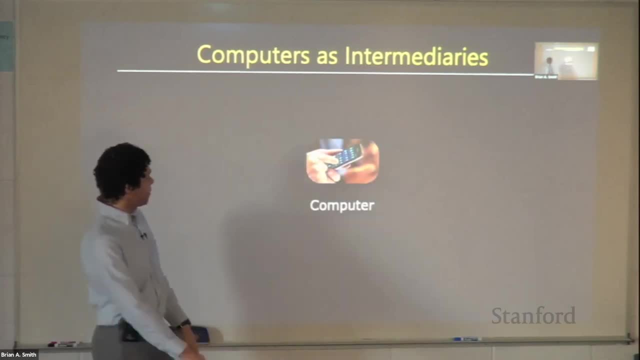 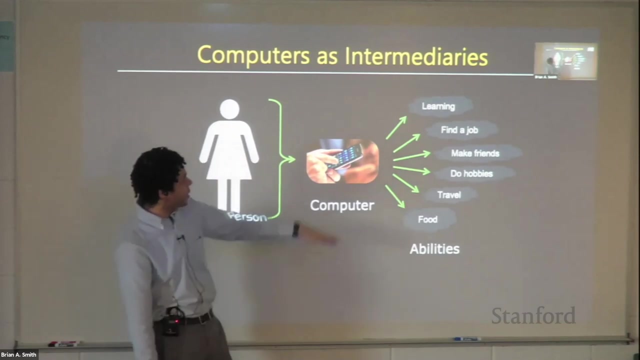 lab view computers as being intermediaries, You know. so here's a computer, for example, people's smartphones, And they act as intermediaries between people and all of the experiences they want to have, everything they want to get out of their lives right. So, whether that's learning, finding jobs, 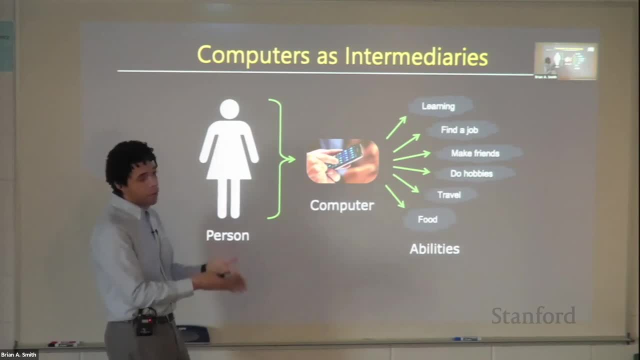 making friends, food, all of this stuff. People funnel their attention through computing devices in order to unlock these experiences in real life, And so that powers us, you know, thinking that computers have the power to grant people abilities, but it's a double-edged. 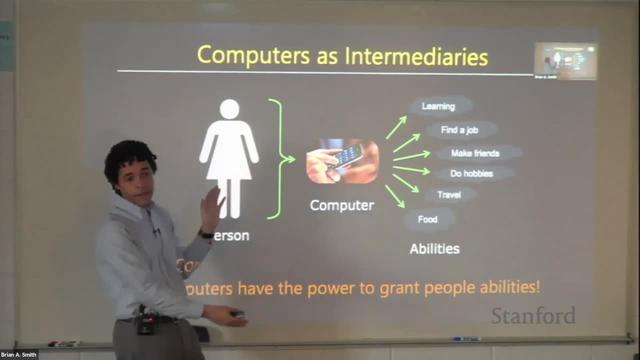 sword. Yes, computers can grant people abilities that they otherwise wouldn't have, and that's how a lot of accessibility researchers view assistive technology. but computers can also act as gatekeepers. right, They can hold the keys, hold back the keys to other aspects of the world. 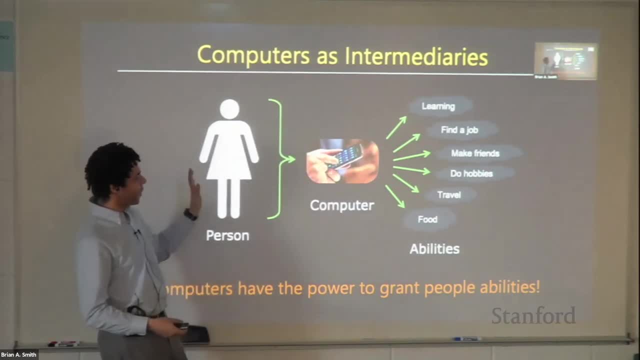 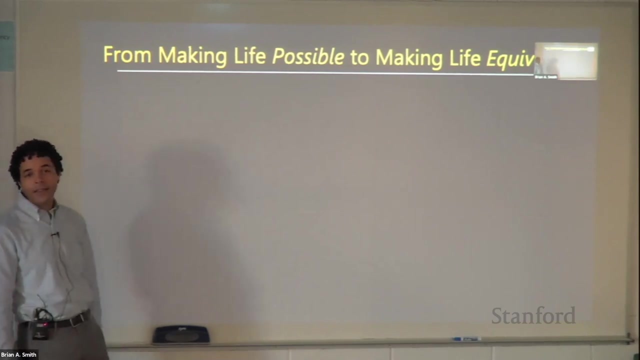 based on their representation of that world, and so they can effectively block people from participating in things in an equivalent manner. so that we'll be looking into that as well. Okay, and so our mantra is: from making life possible to making life equivalent. Let me show. 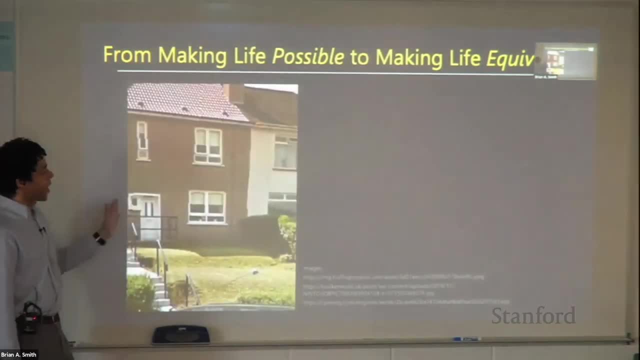 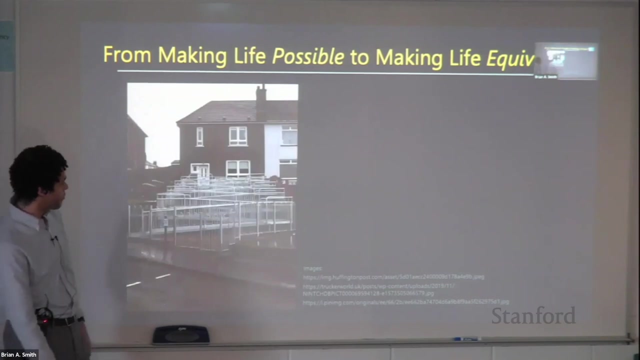 you an example of what I mean in the physical world. So this is a house in Scotland and one of the children needed a wheelchair, and so this family petitioned the town to install a ramp for that child. The town finally did and they installed this. This is the ramp right here. 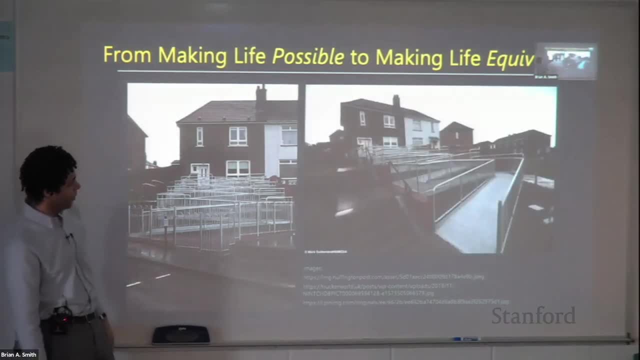 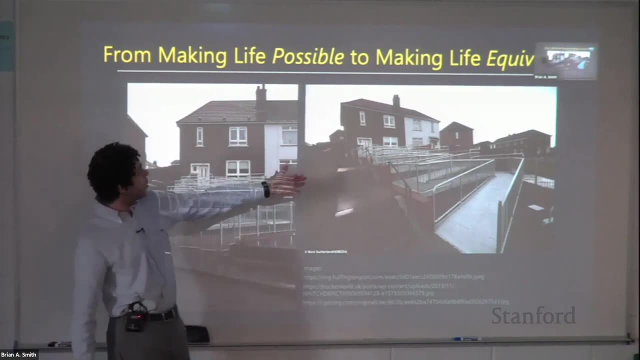 and you know. so I'm going to show you another angle from the corner here, So you can see the stairs. and then there's this ramp on the side. While this ramp clearly makes it possible to enter and exit that building, you know, going up that ramp is certainly not an equivalent experience to just. 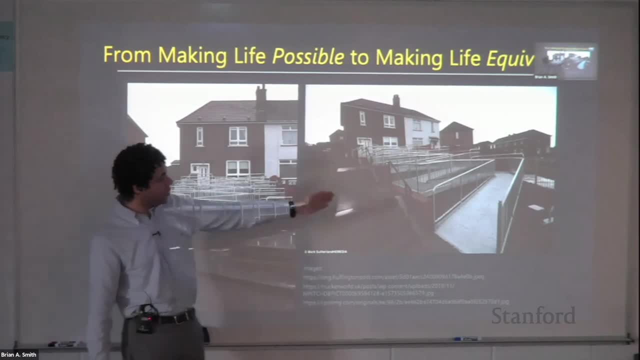 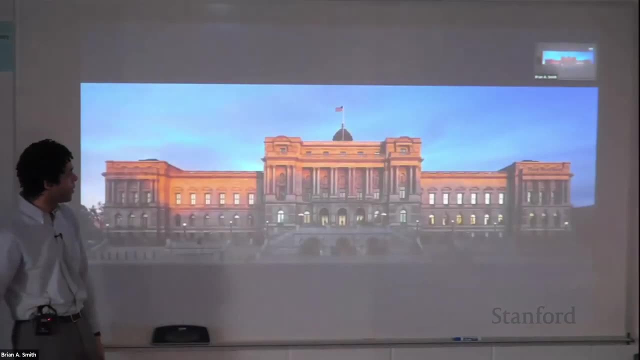 walking straight up those stairs. The only people that would ever use that ramp are people who have to, and that's a problem. So I'll show you another example, physical world. There's a Evans 가지고 where I came from, and we went to this building to get some car insurance. 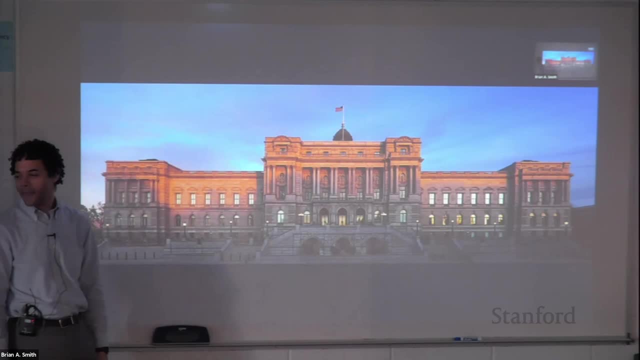 ASHRAE GASH fun. Does anyone here know what this building is? Can give a hint? Does anyone been to this building? It's in Washington DC. Does that help? So this building is the library of Congress, the world's largest library, And the normal route you know to enter this building. if you don't need, 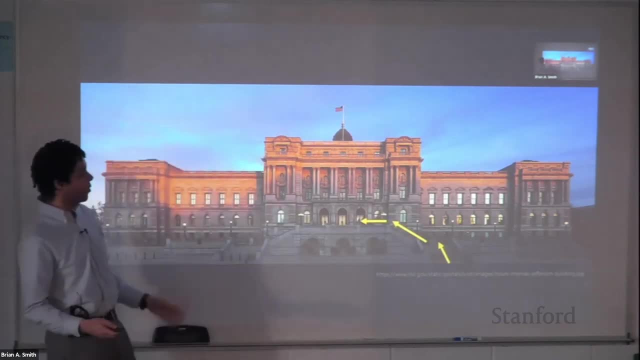 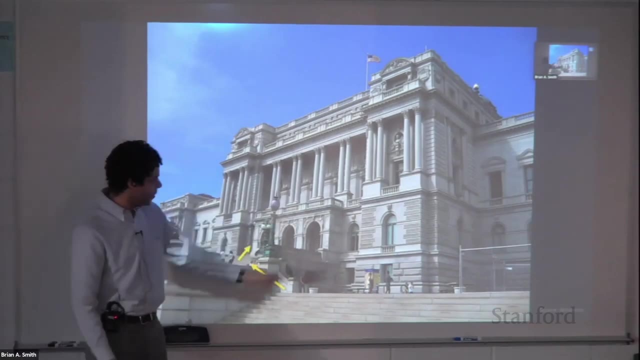 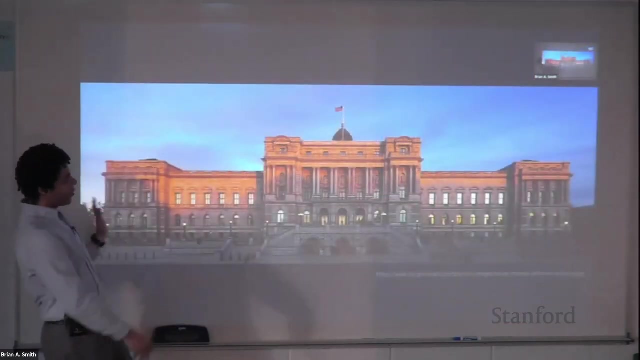 up these stairs, right over here, through the arches, into this grand lobby. here's another view, here's the stairs. you go up the stairs, you enter under the arches. absolutely amazing lobby, absolutely beautiful. but if you need a wheelchair, then your entrance is not shown anywhere in this, in this. 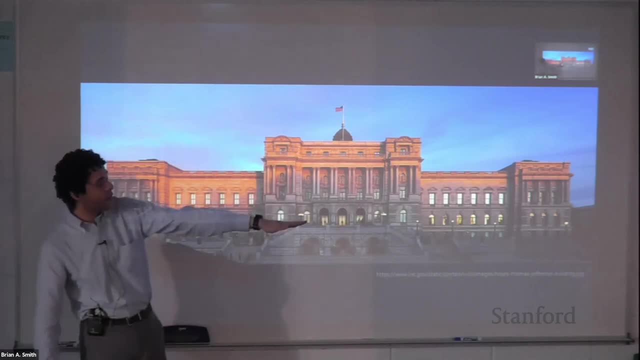 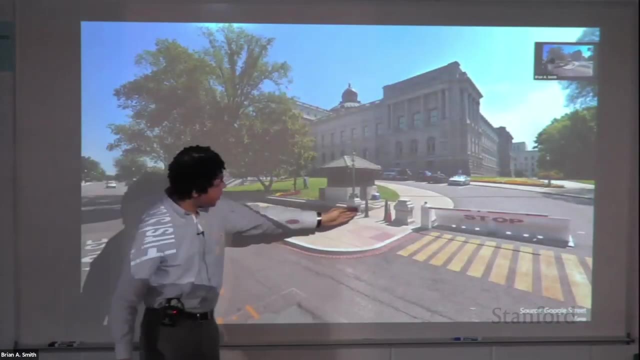 image. actually, you have to go all the way to the end of the block on your right- there's this corner here. this is a google maps view- and then you have to enter right here next to the guard booth, make sure that the guard sees that, yes, you're in a wheelchair, and then you can proceed along. 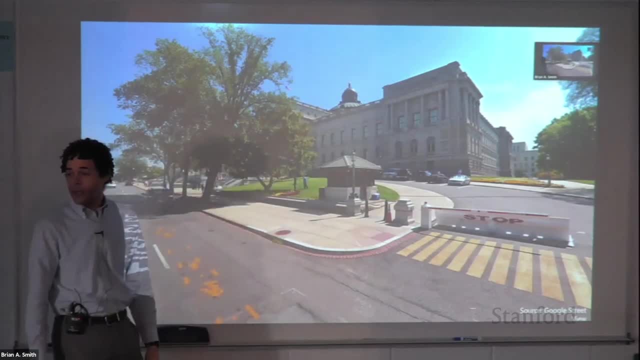 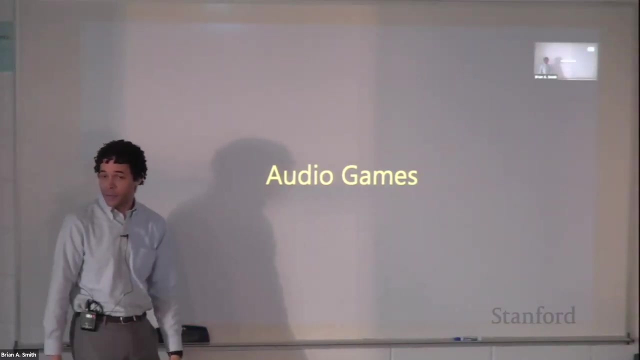 the sidewalk into a lower level of the library of congress, so again, entering is possible, but it's definitely not an equivalent experience. so i just showed two examples from the physical world. this is super, super common in the digital world as well, and so i'm going to be focusing. 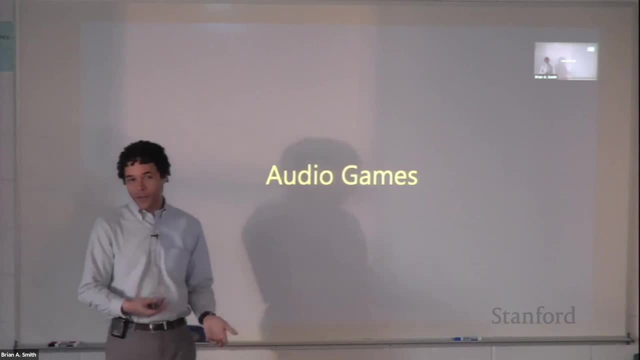 on games, specifically video games, an entire new, like genre of games has opened up, called audio games. and what audio games are are audio representations of video games. that it's like a, a whole class of games that's made to simulate what the video version of the audio games would. 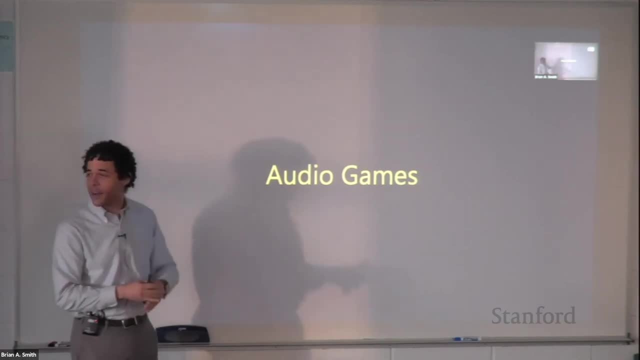 otherwise be. interestingly, you might see this glare. there's a building in new jersey across the river that's perfectly reflecting the sun. right now i can roll down the window, or it'll probably end in just a few minutes, so anyway. so this is audio games. let me show you an example. 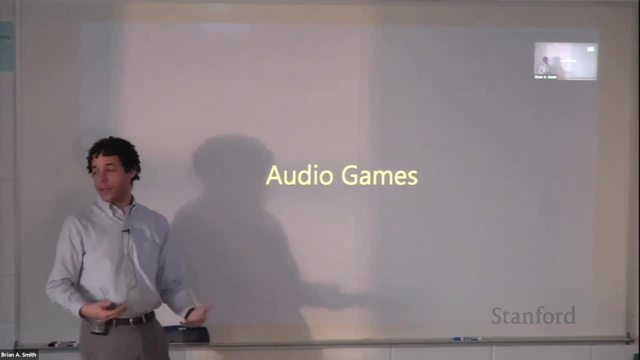 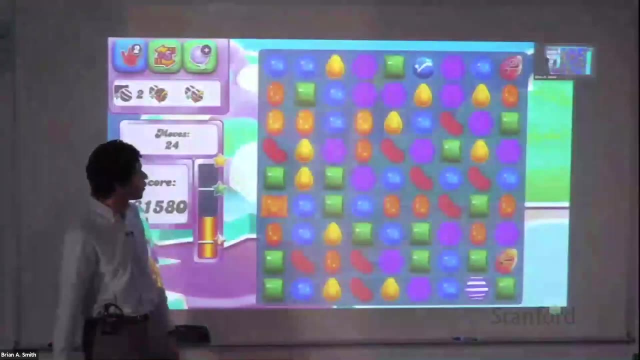 of of some of these audio games. they do not offer the same experience that their respective video game counterparts do. let me show you an example. so this is color crush. most of you have seen it and essentially, uh, you, you know, you just have to. it's a touch screen. 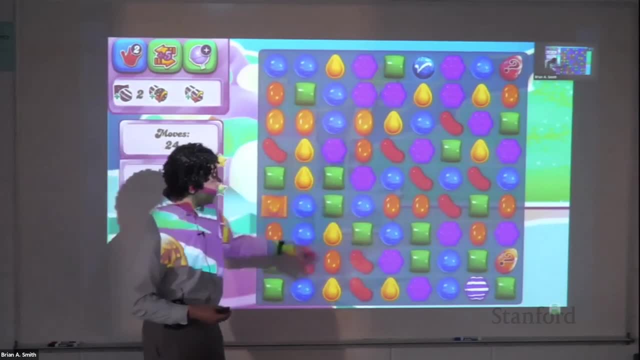 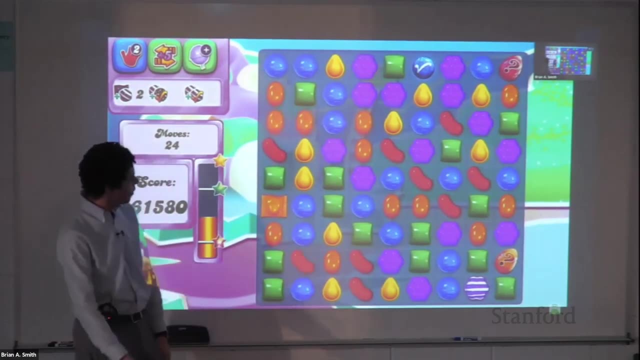 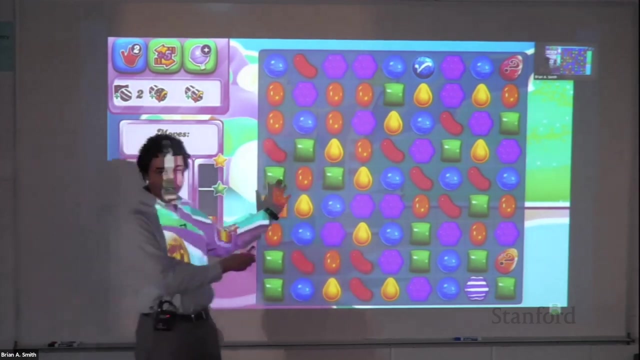 game. you swap, uh, you know these, uh, these candies, uh get three of a kind and then you um and you clear them. so i'll just show some video color crush. so there's some color crush action. everyone's seen color crush, um, so, uh, an audio game version of color crush has come out, um, by. 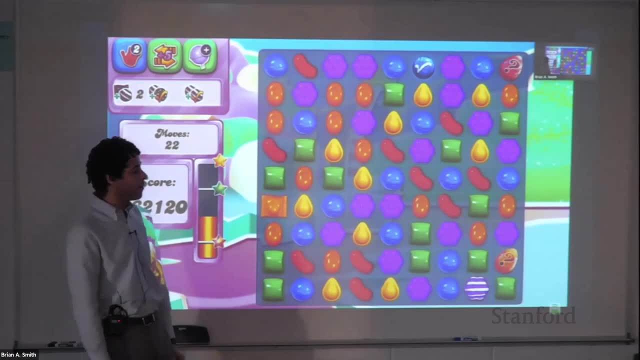 a hobbyist, you know which is great, it's better than nothing. um, you know, i i admire that a lot, but let me show you blindfold color crush. um, that's what it's called, uh, which is, uh, the, the audio, the audio game equivalent of color crush, just so you can see if you happen to be blind or visually. 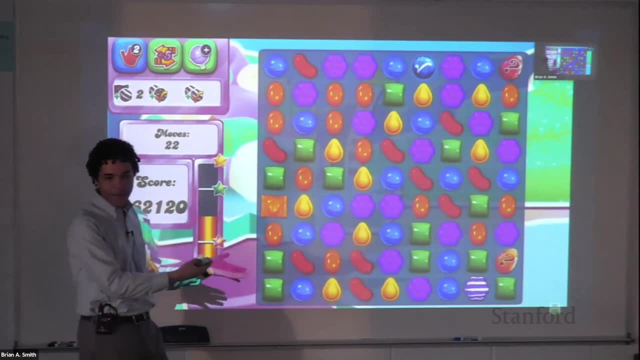 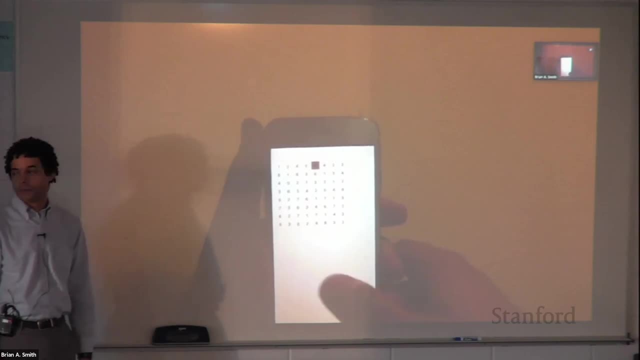 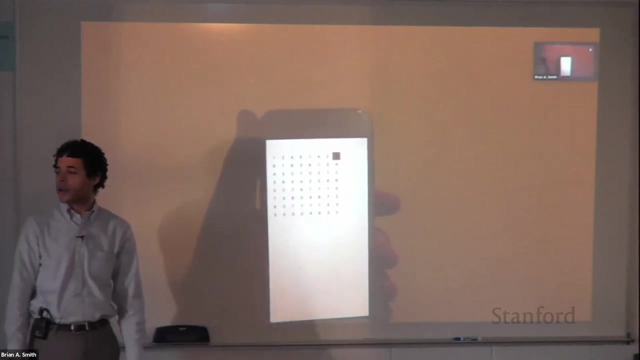 impaired. you don't get to play this. you're going to play this other game, so here it is: blue green, yellow, red, green, blue white, green, white, blue, white. so could you hear that audio, by the way, sort of okay, um, so the sounds, um, uh, essentially was. 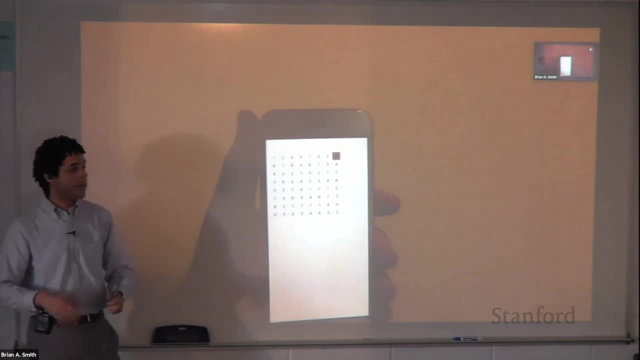 just announcing colors, as the person swiped um, uh, in in this, right. so it's saying blue, green, yellow, blue, white, right, this is blindfold color crush, um, and then i think a a two-finger swipe swaps, that's, and so this is just a ui view, but the player is blind, so they won't. they won't be. 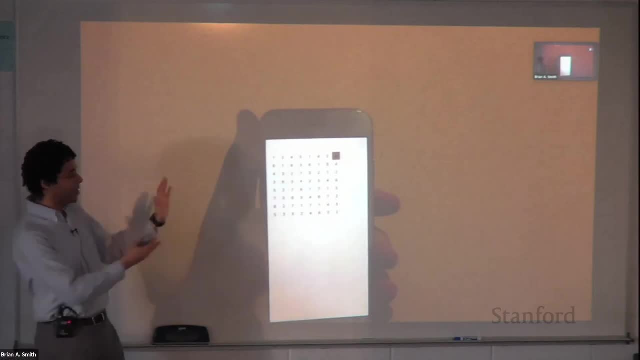 seeing this. clearly, this is not the same experience as playing uh, color crush, right? um, clearly not the same. uh, it's right like. uh, you know, color crush is a very zen-like um experience. um, there's a lot of submission in game design terms. this is all wrote like memorization- very, very different type. 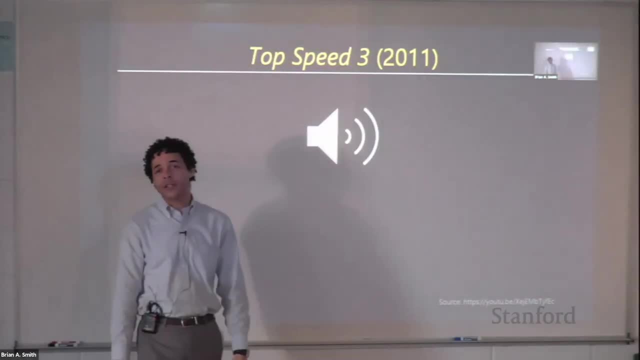 of game. so let me show you another example, right? so actually you know. one point from that, from that example is that merely providing all of the visual information and conveying that in this audio game clearly doesn't do it. you can't just make sure that the player has. 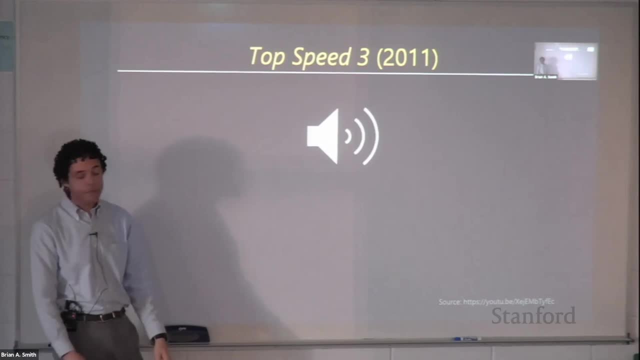 all of the audio information. that doesn't quite cut it. so here's another example, which is a game called top speed 3.. this is a very successful and great, actual, actually racing game- audio racing game that's designed to give people who are blind the ability to play some kind of. 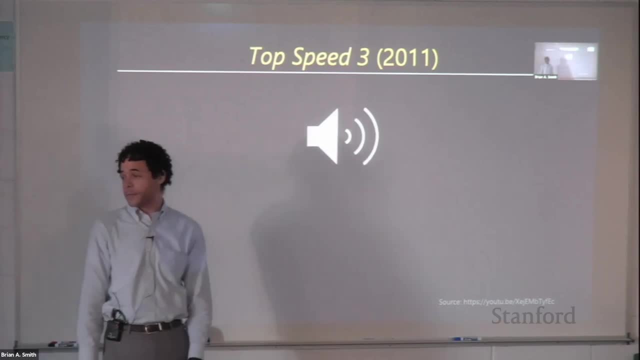 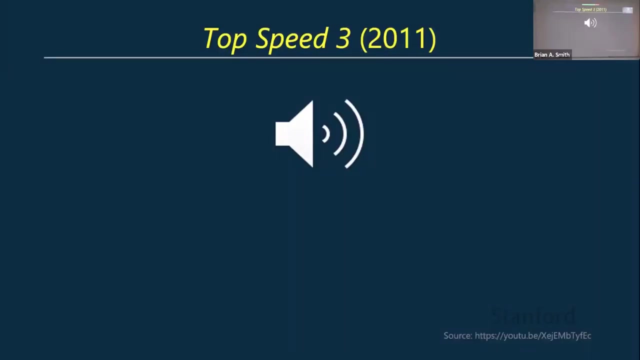 racing game. so let me just show you some gameplay from top top speed. three by show, i mean sound, remember, there are no graphics. let me, uh, have you listen to a clip of that and i it's important that you hear this, so let me just see. okay, so here's the game. 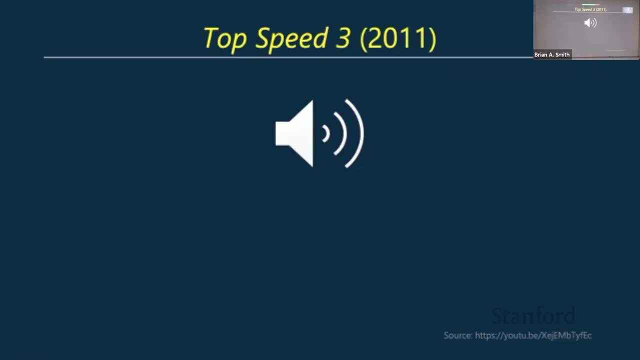 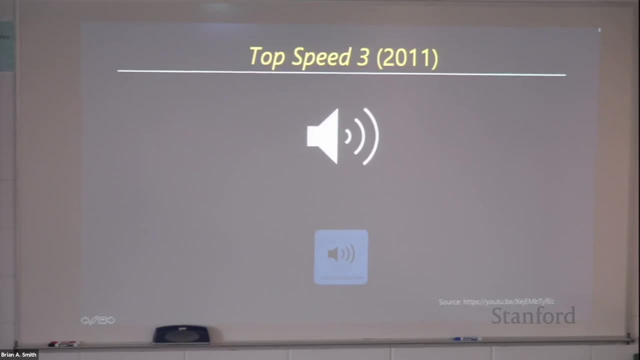 what? all right, so i think this is the best that we're going to be able to do in terms of the sound, okay, yeah, there are no visuals, it's all. it's all sounds, unfortunately, um, okay, so, yeah. so so what you heard- i'll just explain, um, as as the game was playing- was: the game was announcing left right. 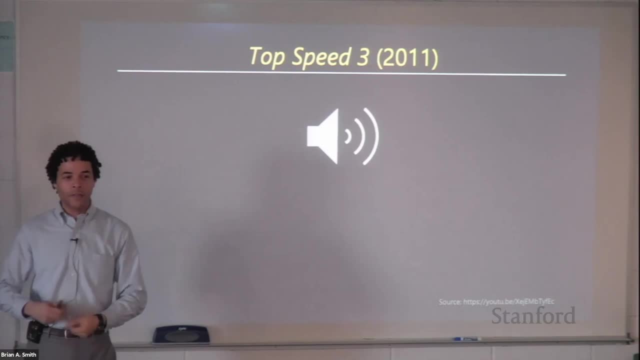 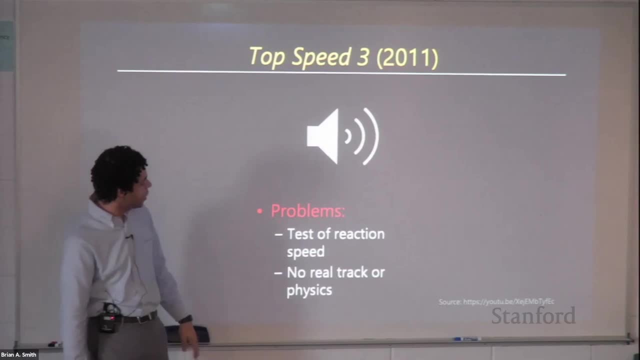 really feel like racing. right. there's several problems here. one is that it's just a test of reaction speed, naturally, um. the second is that there's no real track- uh, no actual track simulated in the game, or vehicle physics. it's a very simplified version of a racing game. it's a very 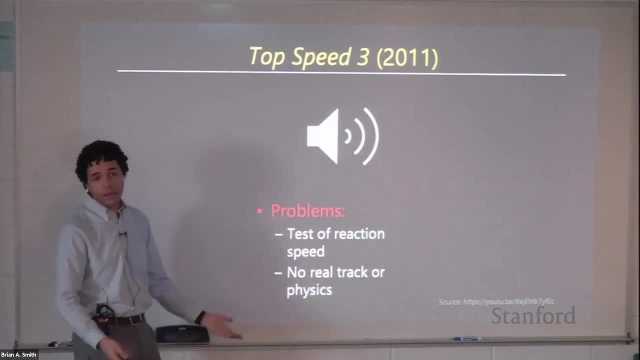 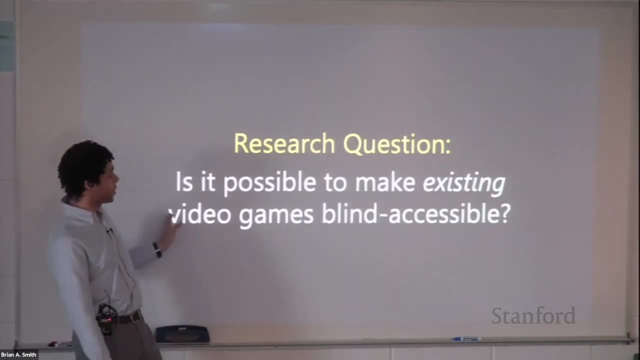 simple racing game, um, and so this you're going to see this time and time again with audio games, and so i'd like to ask the following research question, which is: is it possible to make existing video games blind accessible, rather than creating this new class of, you know, separate and not quite? 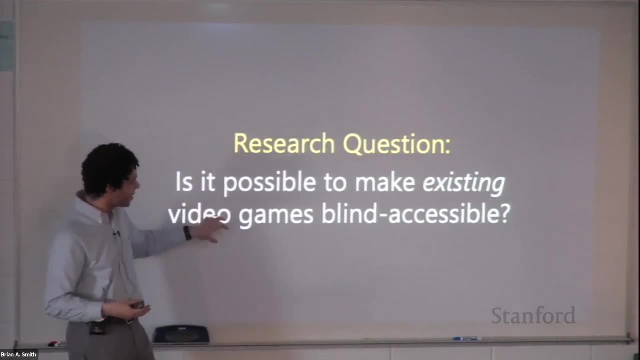 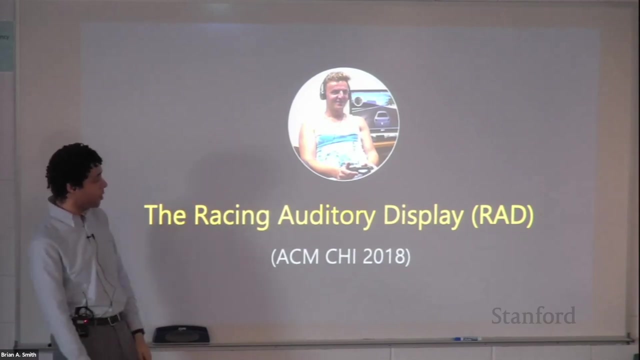 equal games, audio games. can we make existing video games playable by both people who are sighted and people who are blind, who want to play that same game? so, just to you know, move towards this answer. i'm going to present a project of mine called the racing auditory display, or the rad for short. and what this? uh, what this project was was? it was an. 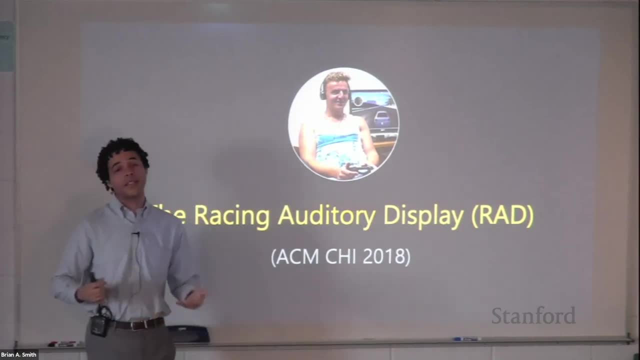 audio system designed to be used for a standard pair of headphones that makes it possible for people who are blind to play the same types of racing games as sighted players can, with the same speed and sense of control that sighted players have. um and so, so i'll go into the design of the 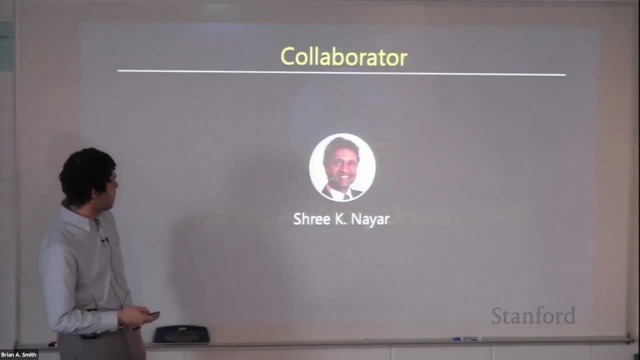 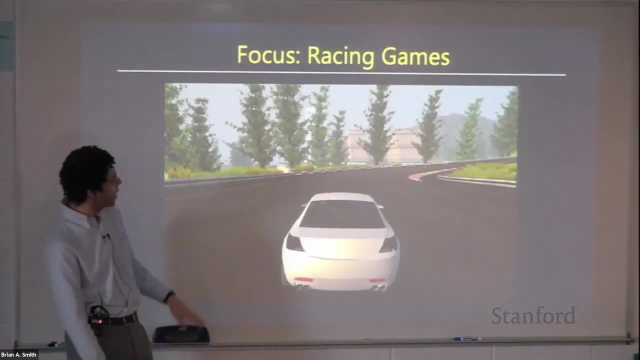 system and some of the insights that we got from it. um, i collaborated on this with my former phd advisor, uh sri nair, at columbia, and but before i do that, let me just, uh, you know, i showed blindfold color crush. i showed top speed three. why racing games in particular? um, we're interested in finding. 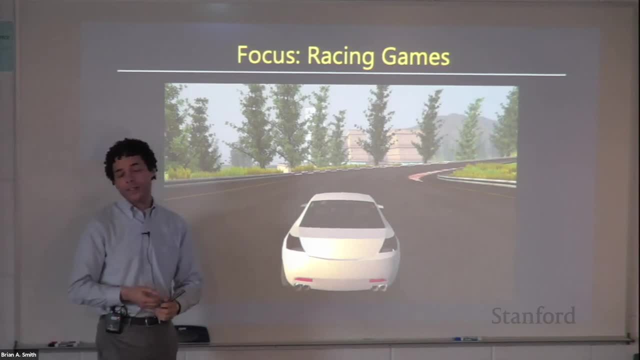 general principles or or methods for uh strategies for making uh games in general blind, accessible, right, but we started with racing, racing games, and there are two reasons why. number one in a racing game- they're only you know- it's both easier and harder. they're easier and harder one. it's easier because uh. 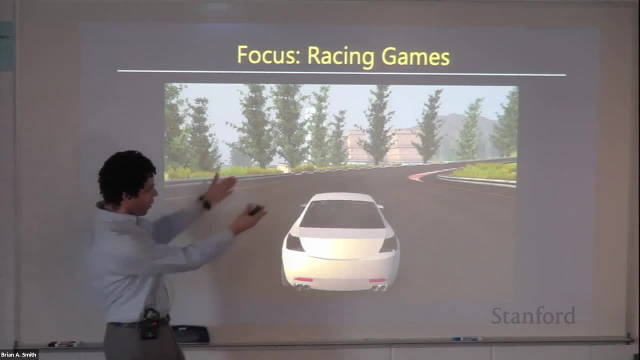 racing games only have a certain, like a small amount of information, um that the player needs to know and be aware of at any given time. so it's, it's an easier test. you know, test ground, test bed for that purpose, um. but then, two, it's harder because racing games move. it's really 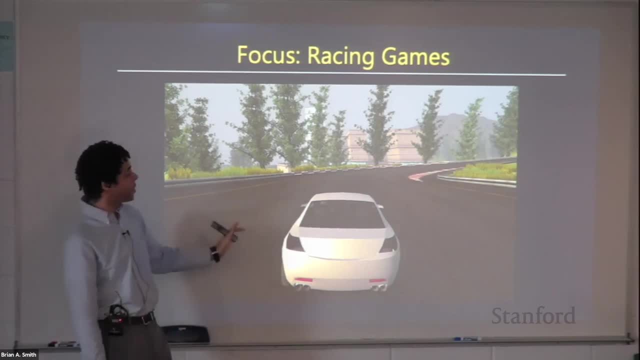 important to communicate that information in real time. the player doesn't get to just like: pause, think about things, make another move. you want to keep it moving so that it feels like racing. you don't even want to slow the game down because racing is all about speed. so how do you communicate all the information that needs to be communicated in real time was a 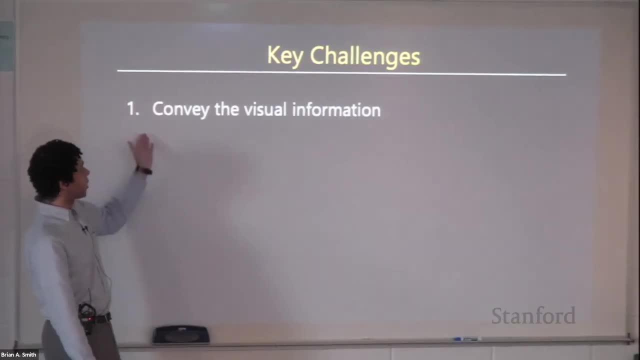 real challenge. so, speaking of challenges, right um conveying the visual information. that's challenge number one. how do you convey that using, uh, sound or you know, not visuals? um two, we do that while serving the game's tempo. it has to be moving at the same speed to still feel like racing. 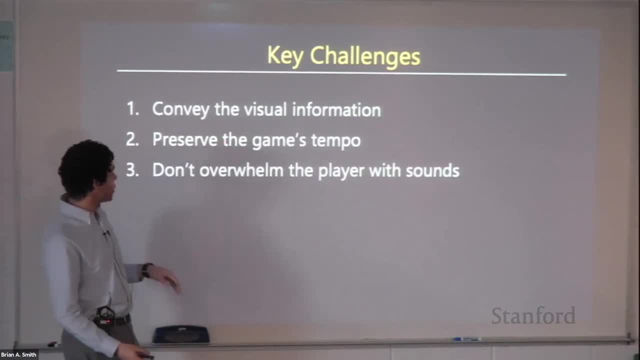 three: even though you're trying to convey a lot of visual information, how do you do that without overwhelming the player with sounds? and four, last challenge is we wanted to use standard hardware. no fancy, you know body worn stuff, just a regular pair of headphones and maybe the 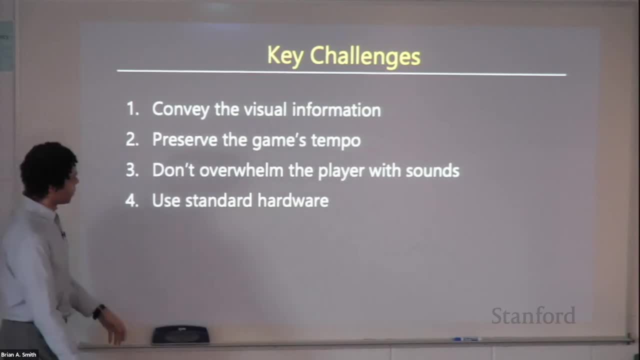 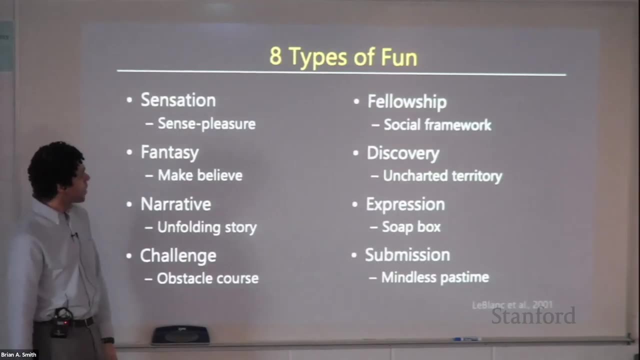 rumble motors within a standard video game controller, so that this like solution could be generalized to and deployed on consoles and pcs. um, so the reason why we thought that, uh, you know, that that problem of blind accessible games could be tackled is, um, is kind of from wearing our game designers hat. 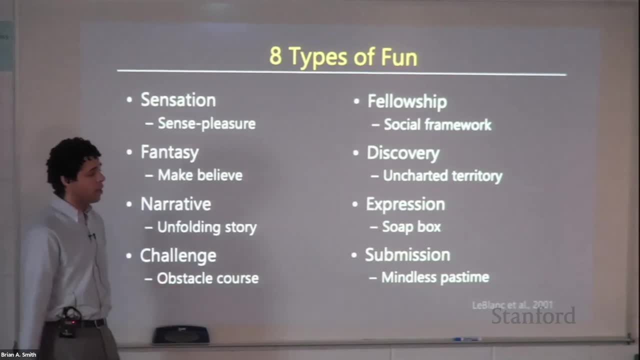 so in game design it's, um, you know, pretty widely known and this is spoken about at game developers conference all the time, um that, um so so a lot of folks, including mark leblanc here, that who i cite the question: what do players get out of video games? what aspects of games are fulfilling for? 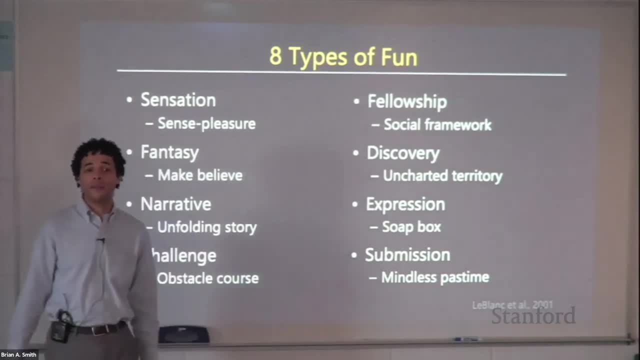 players. in what ways are people fulfilled by games that they play? so that's what this quote, this thing is here, which is like eight types of fun. um, what kinds of fun? if you were to split up that term and not make it overloaded, what would that look like in terms of what players are getting out of? 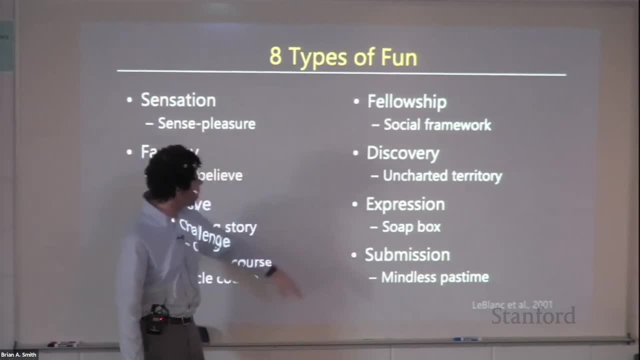 games, and so that includes things such as discovery submission- so can't candy crush, you know- and color submission- uh, challenge fantasy, etc. these are like this is breaking down in terms of what players get out of games. if you look at these, only one of them is heavily dependent on visuals. 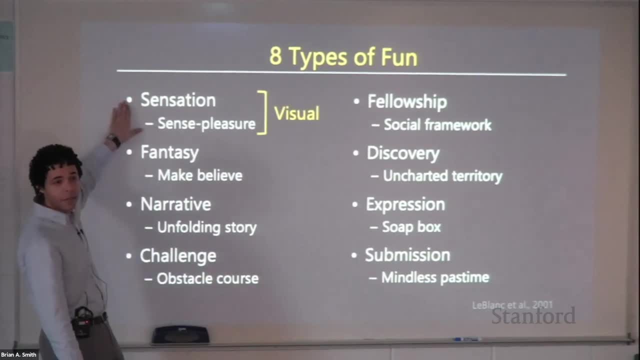 and that's sensation. uh, games as sense pleasure, uh, where, like just pretty graphics are really amazing environments um themselves can be fun to, to explore and to see, right, or like you know, oh, wow, this game did you feel like the, the, you know hd haptics, etc. hd rumble in that game, that's. 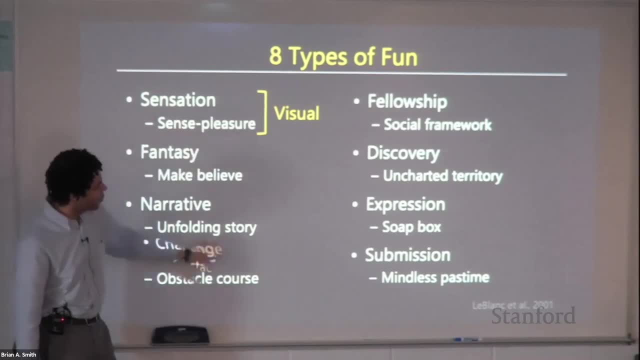 sensation. only one is visual. the rest, um, visuals aren't really necessary to any of these things, and that's why that was the. the key insight here, like this, is why it should be possible to make video games, um, you know, except for sensation, perhaps, uh, blind- accessible. okay, so ultimately, 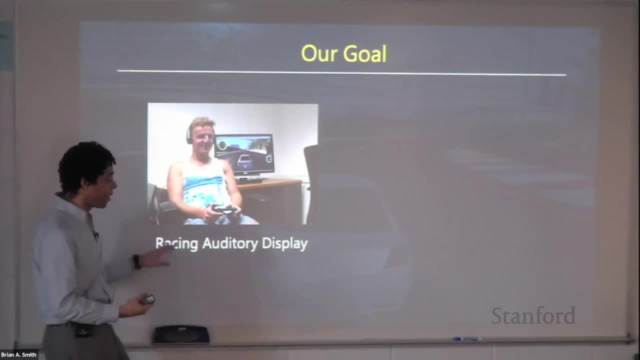 we wanted to create a real racing auditory display, a rad, some kind of audio system that really feels like racing, so players get that same experience of racing, as opposed to one of those top speed type systems which are just announcing turns. one of these basic auditory displays- um, there's an obvious 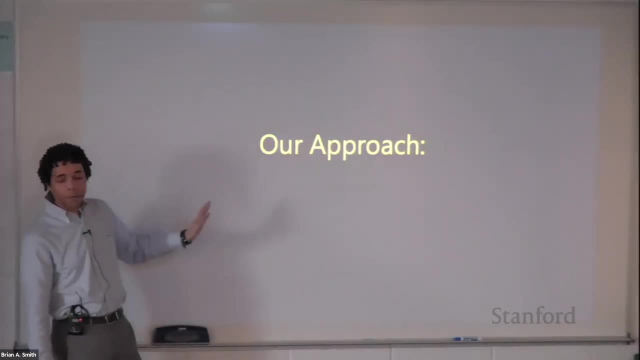 analogy which you can guess. so our approach um to to making this happen, um is to, as i said, with the library of congress example, you know. so that's that's where this comes back. um is to replicate the experience and not just the visual information. more specifically, uh, experiences are based on meaningful choices that people make. 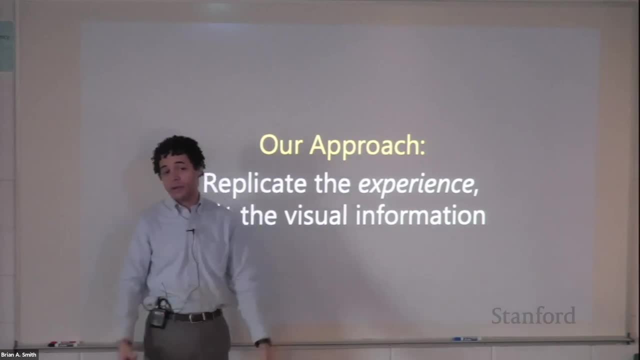 and this is also pretty common knowledge in in game design, right. uh, players make meaningful choices from moment to moment, and that constitutes their experience in the game and their feeling of agency when playing the game. and so, by replicating the meaningful choices from moment to moment, that 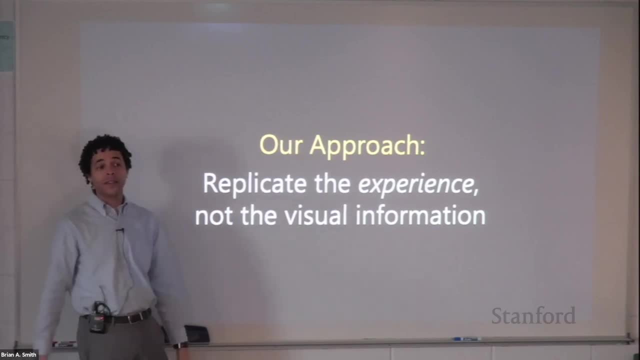 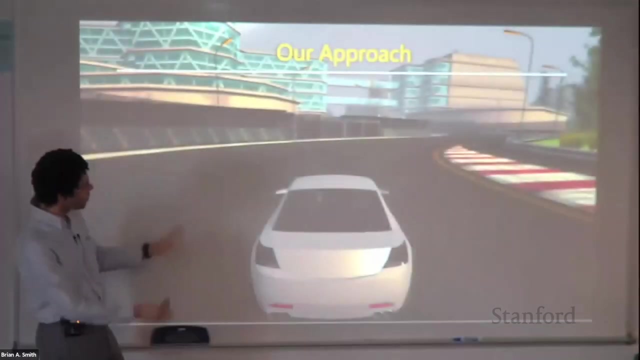 players are making. uh, in terms of the audio cues, so that you can design the audio cues such that they give players the same input information to make those same decisions. uh, that's when you. that's the secret sauce. so let me just be a little more um specific here. so, in terms of racing game, our 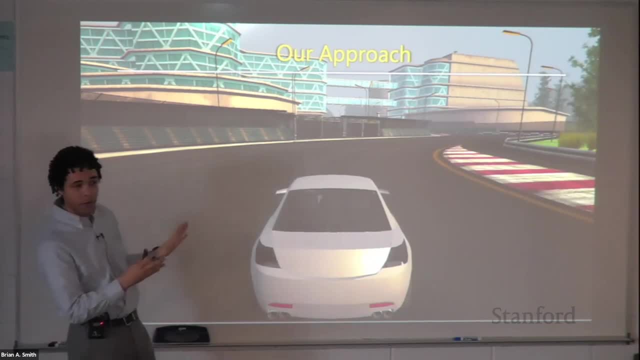 actual approach to solving this problem and making it blind, accessible, making it really feel like racing is to race a whole bunch of laps around the track ourselves, and then we're going to be able to go back and watch the replays frame by frame and then almost go. you know, go back and watch the replays. 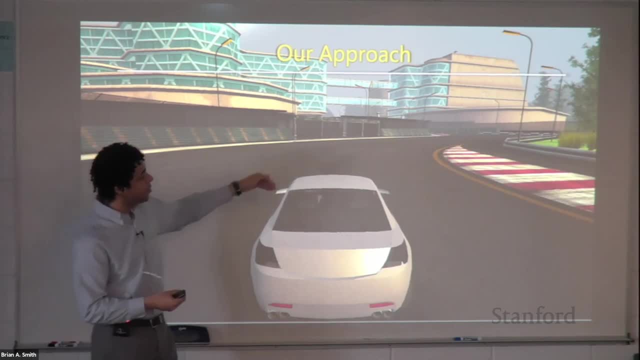 frame by frame, and really analyze from moment to moment: what are we making our? what pieces of information are we making our steering decisions based off of? um, what is it that we're just that's making us decide to turn a little bit left, turn right, you know, at from moment to moment, that is. 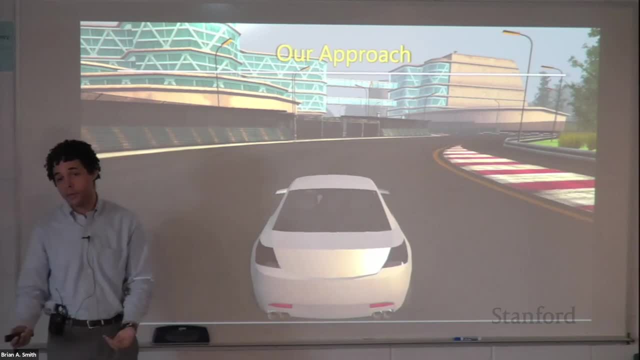 the information that's needed to make those meaningful choices from moment to moment. so it's not important to replicate all of the visual information here, only the information necessary to preserve those meaningful choices. that gameplay, that's the idea and so it turns out with. with a standard racing game there are two main uh choices that a player 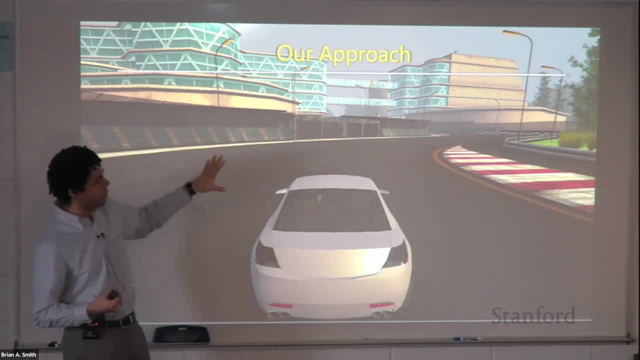 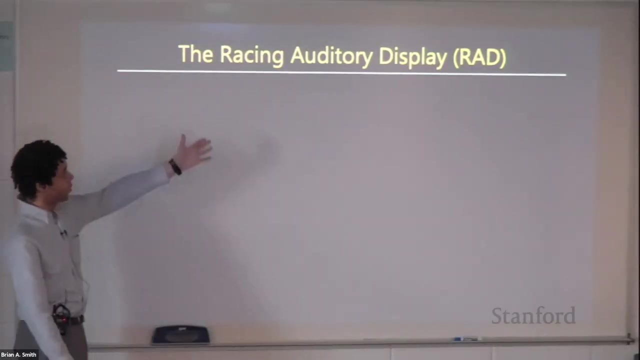 needs to make, or two rather, pieces of information that players make their the base their steering decisions on. number one is how the race car is situated on the track. number two is the nature of upcoming terms, and so, with the rad, we designed two audio cues to convey those two separate things. so um, the rad comprises: 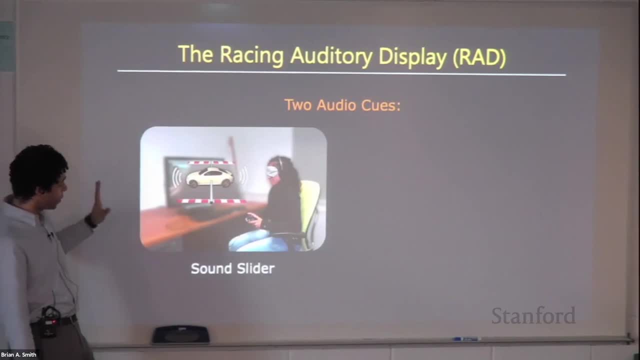 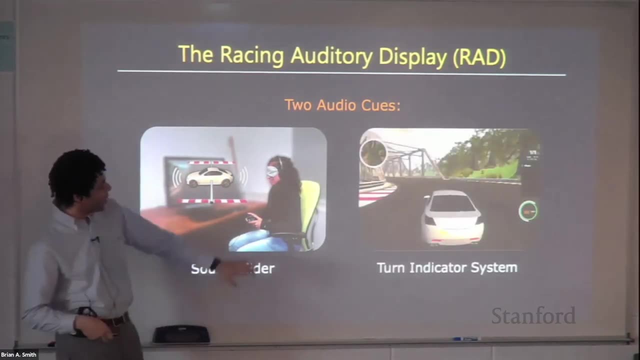 two audio cues. one is what, uh, you know, we call the sound slider, which, um, uh, communicates the car's positioning on the track. i'll explain how that works. and then the second is the turn indicator system and that, uh, that communicates the nature of upcoming turns. so let me talk. i'll talk mostly. 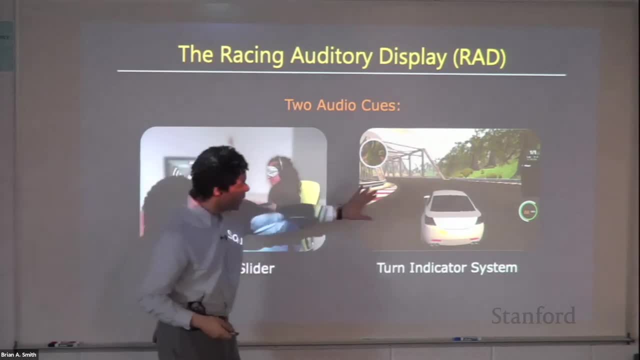 about the sound slider. it's a little bit more complicated, but it's a little bit more complicated, so let me talk. i'll talk mostly about the sound slider. it's a little bit more complicated, but it's a little more involved. spend more time here. and then the turn indicator system. 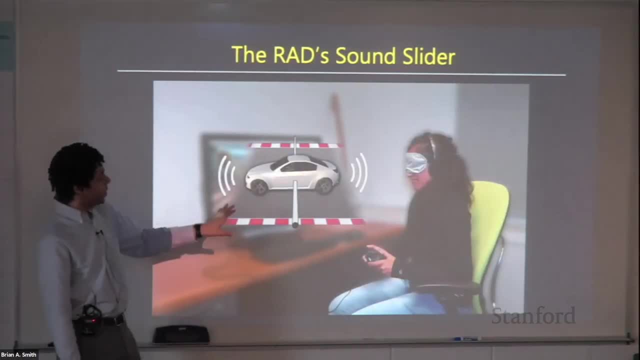 okay, so the sound slider. the way that i like to explain this to uh, to players is like follows: imagine that you're sitting directly behind the car that you're controlling, so that you hear the sound of the car's engine right in front of your face as you steer left and right. you're controlling that car. that engine sound directly. 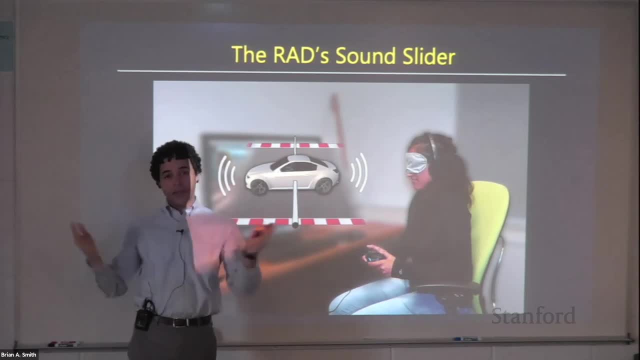 so it's going to slide laterally in front of you in the soundscape in 3d space, um, in in front of your face. that's the sound slider. that's essentially the concept. but it raises a really interesting sort of research question. if you, if you peek behind the curtain here, 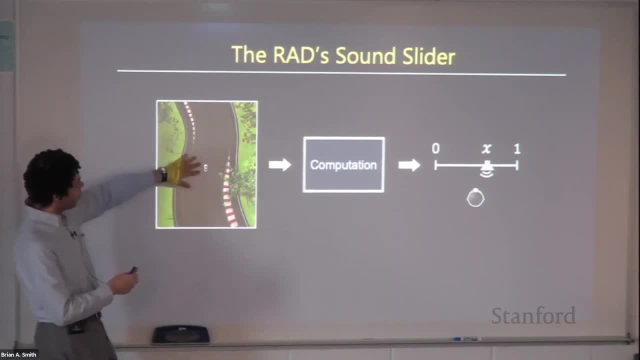 you'll find that we have this situation where, right, the whole point is to communicate the cars. uh, you know how the car is situated on the racetrack. the car could be pointed any given way, it could be oriented any or, you know, placed any way. the track could be doing a. 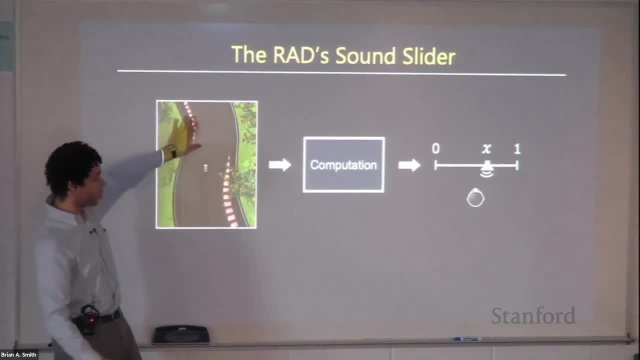 whole variety of things. there's a lot of rich information about how the car is situated here, and we somehow want to use computation to distill that information down to some value of x between zero and one. somehow it's almost a dimensionality reduction that we're trying to perform. so then the 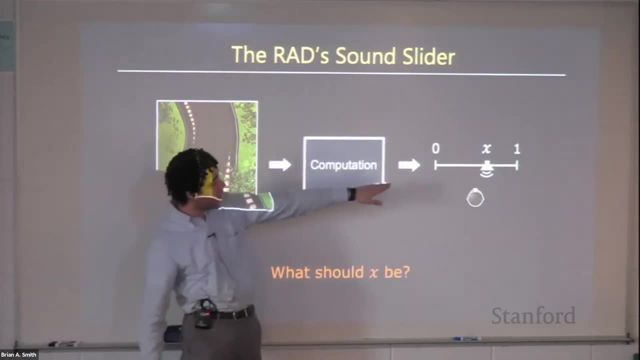 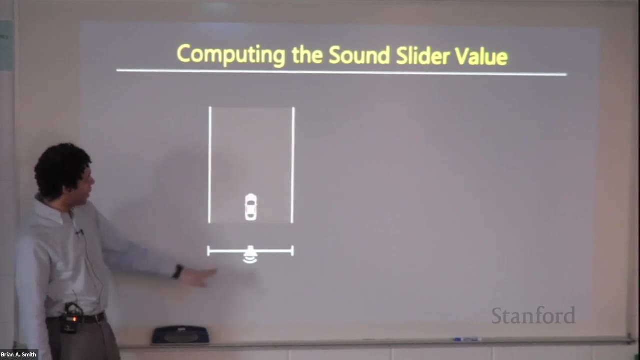 question here for the sound slider is like: what should the value of x be? so one naive approach first take is: why doesn't, why not use x to communicate the car's lateral position on the track? the car is over? here the slider might move, you know, to match wherever the car is laterally. 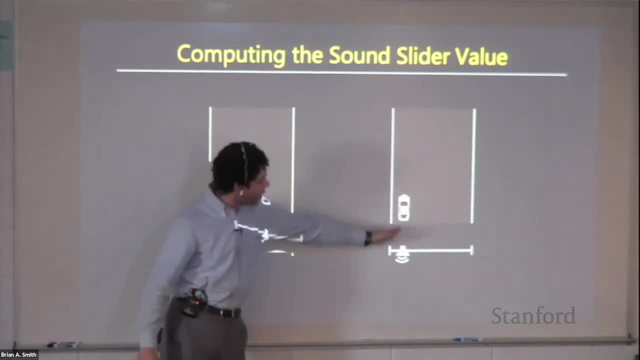 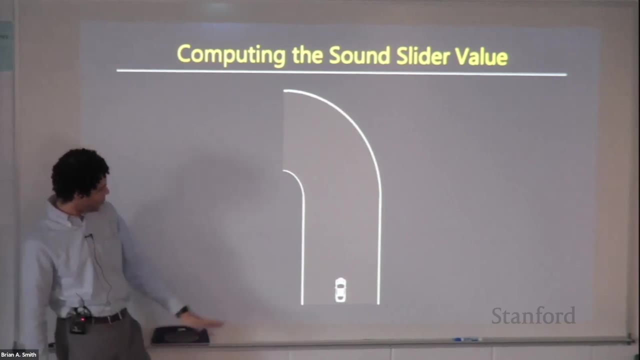 so if it's in the middle, be in the middle. if it's kind of on the left edge, be on the left. it's one idea. that idea falls apart a little bit in this situation, where you have a straightaway followed by a sharp turn. essentially the slider will stay in the middle and then it'll very quickly veer to. 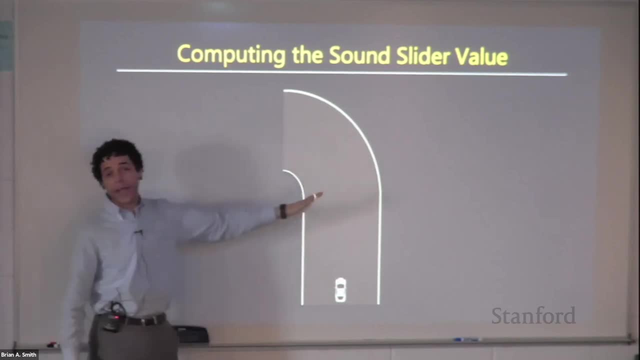 the right. uh, so fast, like too fast for the player to even react to it. um, so there's a problem with that, and so what that means is that these two situations, um, you know, the car being right here at the, at the straightaway, versus the car being centered laterally but right at the- 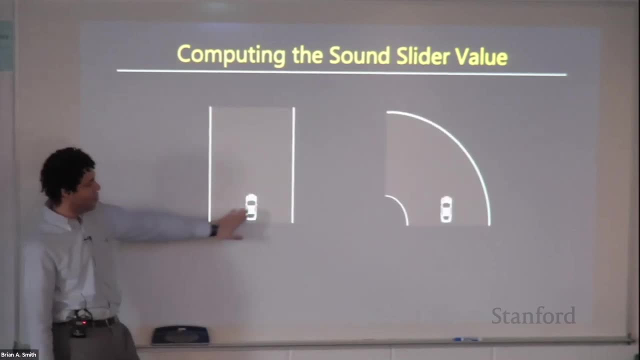 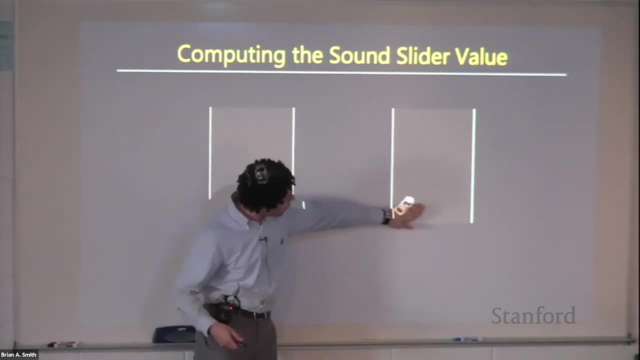 precipice of the turn. um, they're actually very different beasts, and so the sound slider should actually communicate these two things differently. same as these two situations: even though these cars are both laterally towards the left, if, as once you point the car towards one edge, you have a very different right, you're in a very different situation, and so maybe the 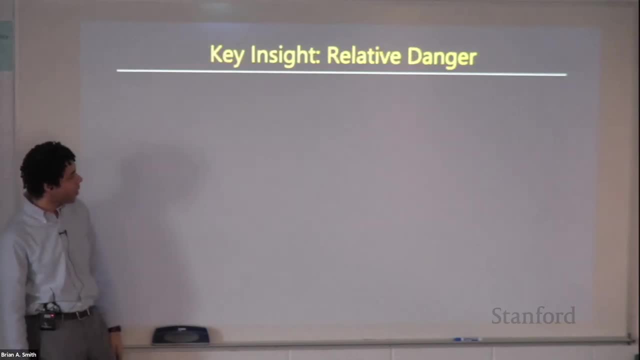 sound slider should reflect that. ultimately, it's about the relative risk of hitting either edge of the track. that's the key insight. it's the relative danger here. so, for example, right in this car or in this scenario, what we end up doing is calculate the risk of the car hitting the left or right edge based on the lengths of these. 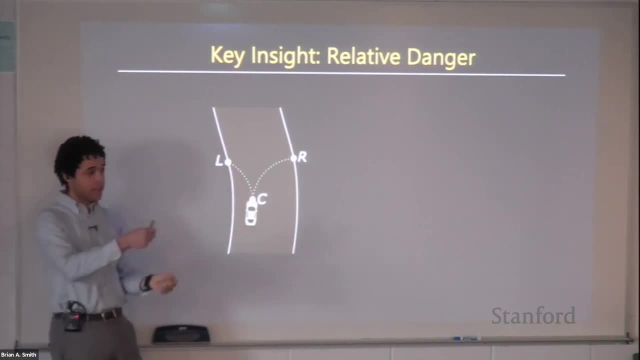 trajectories. if the car was just, if the player was to steer left, how long would it take to hit the left edge? and likewise for hitting the right edge, that will represent the car's relative risk of hitting either edge of the track at that point in time. so if we think about that, um, 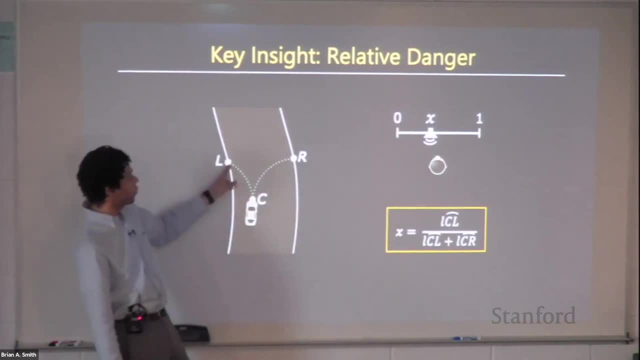 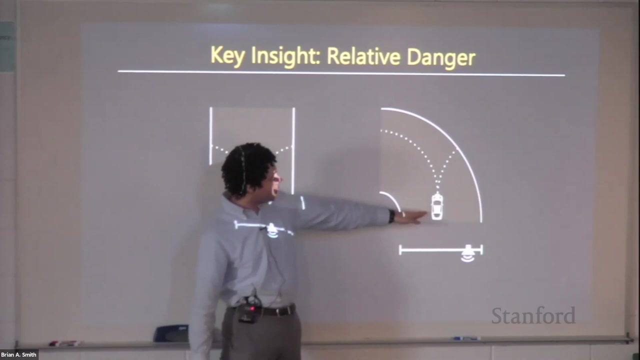 we can actually set x to this value, which is just the ratio between these arc lengths. it's pretty, pretty simple here, and so let's look at these scenarios again. this car that's right in the middle, the arcs have the same length, but this car that's on the right right, the left arc is going to swoop. 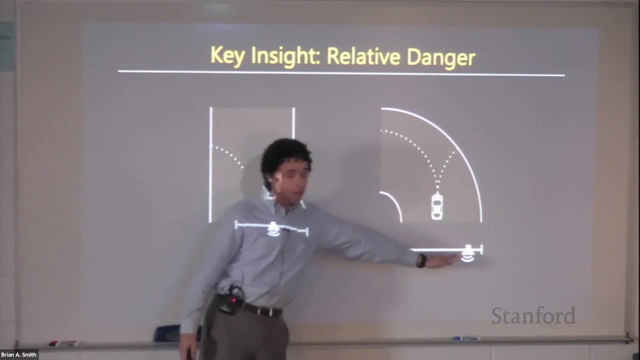 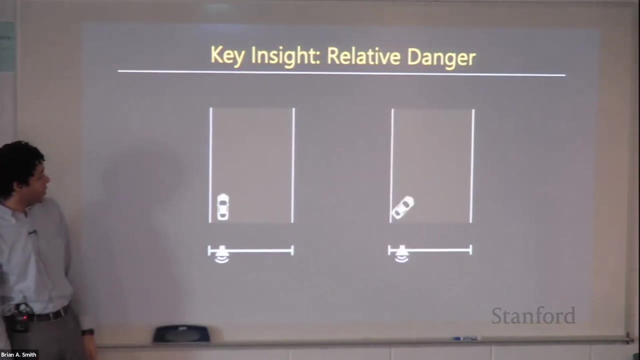 around the turn. it's much longer than the right arc, and so the it should be communicated very differently. the car is at great risk of hitting the right edge. same with this scenario. so the left arc is shorter in this case, but the left arc is a lot longer in this case, and so we'll be. 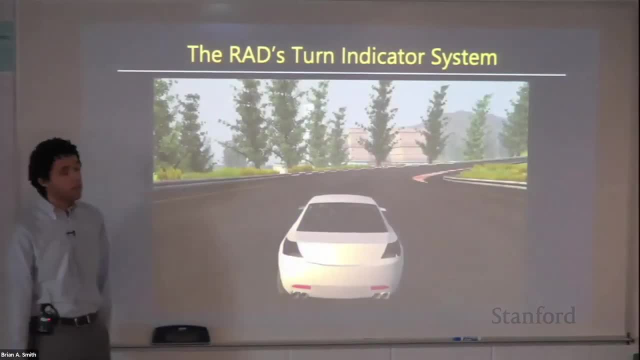 communicating that risk very differently. so that's the sound slider. it's like communicating the positioning of the car on the racetrack in terms of its relative risk of hitting either side, but that will be complemented by the turn indicator system, that other piece of information. 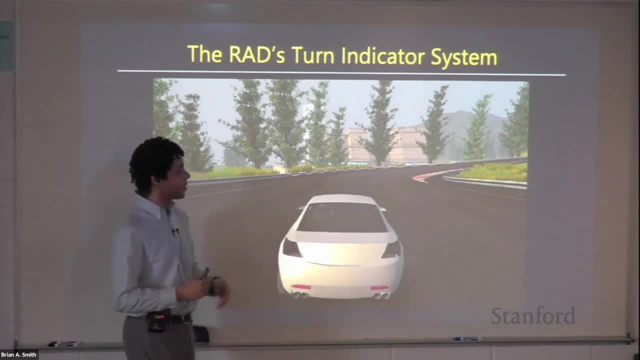 which is the nature of upcoming turns. so the way that the turn indicator system works, um is is is as follows: so communicates the direction, the sharpness, the length and the timing of upcoming turns. the way that it works as a player is approaching a turn, they'll hear an announcer announce the. 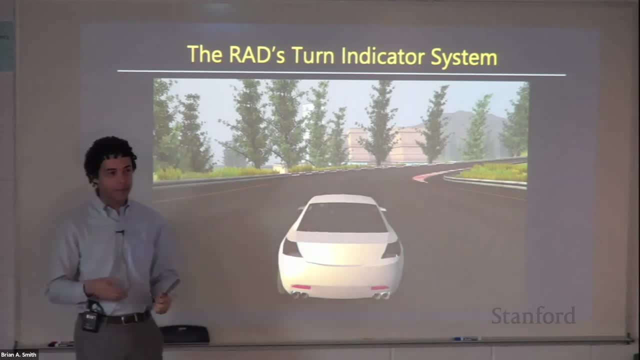 number. so, for example, they might say eight for turn eight, just to help the player with memory remember the turns. and then at the same time they'll hear a series of four beeps from either from either ear. it'll sound like coming from one side or the other. 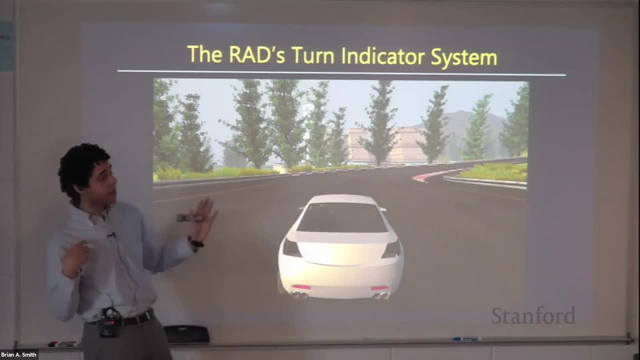 the other. if it's a right turn, it'll come from the right side. if it's a left turn, it'll come from the left side. the the pitch of the beeps indicates the sharpness of the turn and we, you know, we have three different turn sharpnesses. the reason there are four beeps is that they establish a rhythm. 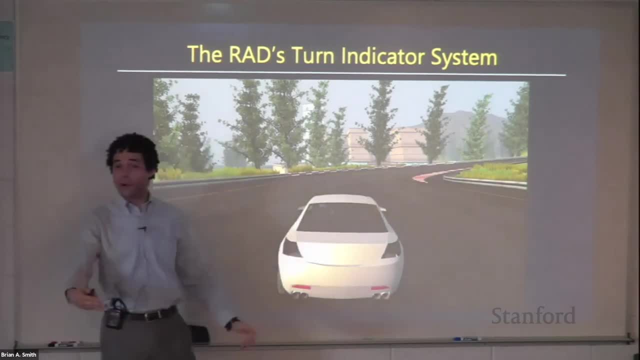 so that the turn itself will always start on the fourth beep. so as the player approaches the turn, they know exactly when the turn is going to start, they know the timing. and then that last beep that they hear as soon as they approach the turn. and then that last beep, that's when they'll surprise the. 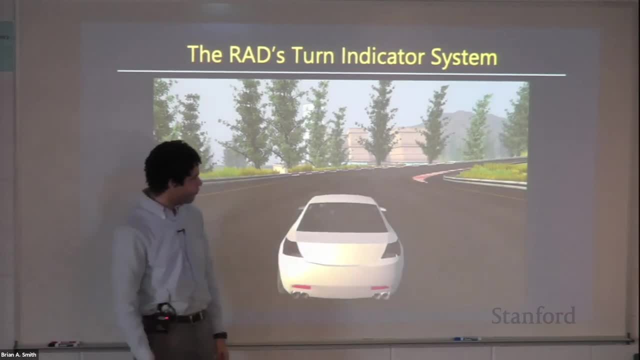 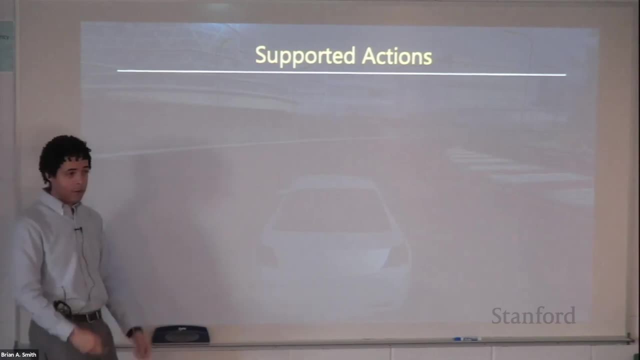 previous turn. they'll say, oh, the second arm is up. okay, that's what you had in the middle. there's, that's what you had in the middle, and they'll take a look at the turn and they'll do their turn. they'll use that and they'll take a look and say, oh, it seems like that's what it really does. 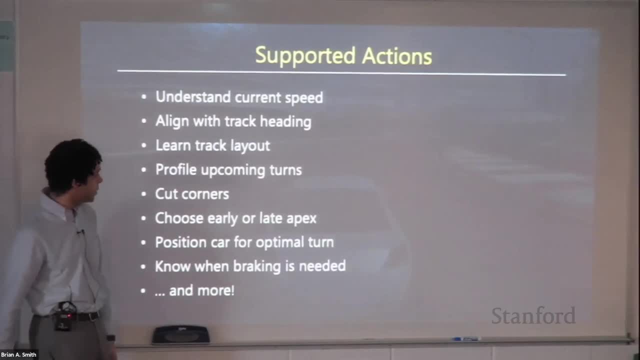 so they start with a nice sound and then, after a while, the sound, the turn indicator system continues sounding as long as the player is is in the turn. so so that's how the the sounds, the turn indicator system works, and so together the sound slider and choosing an early or a late apex. 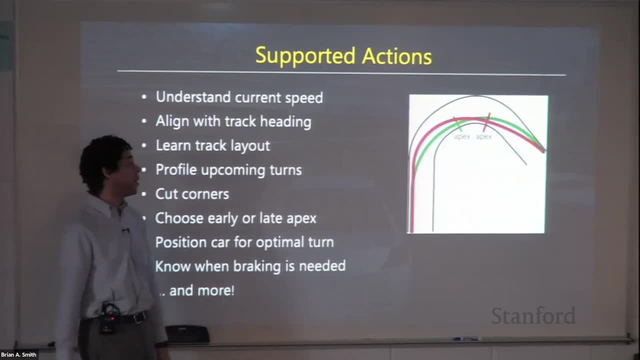 you can do all of these things with just those two audio cues. And in fact we had people who have been blind their entire lives. try out the RAD And by the third lap they were able to actually do a lot of these advanced stuff like cut corners and things. 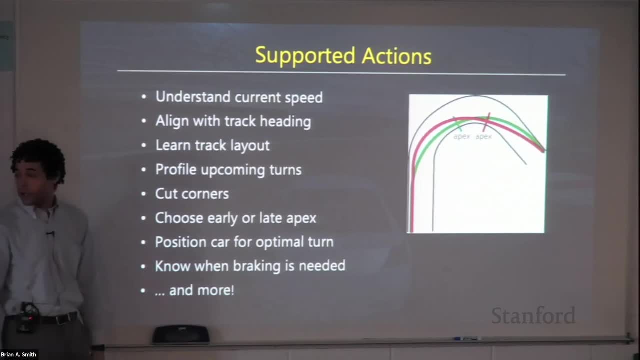 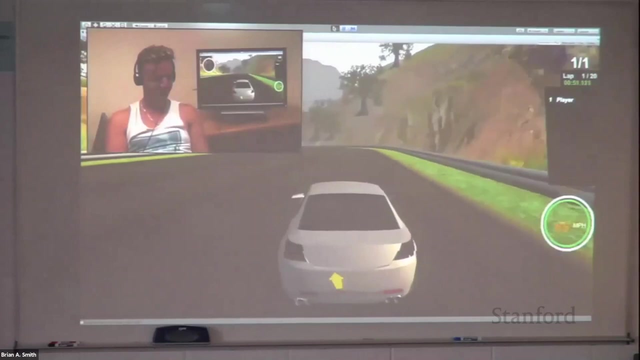 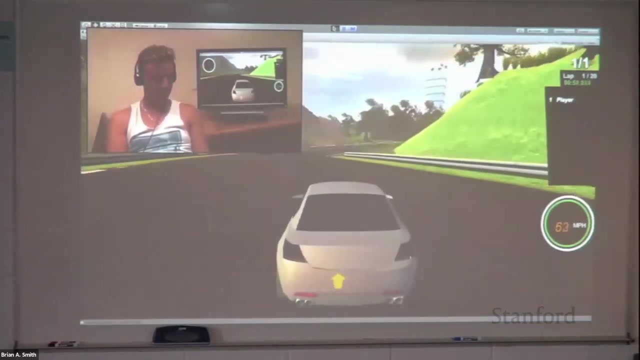 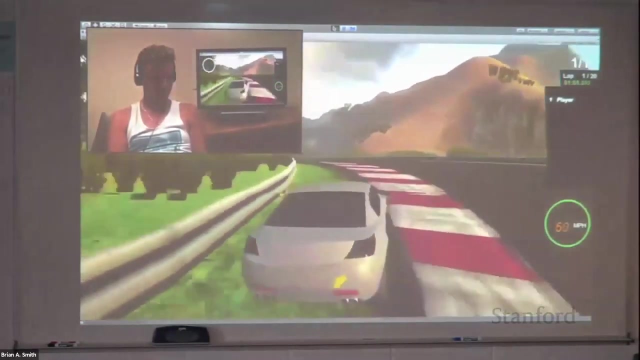 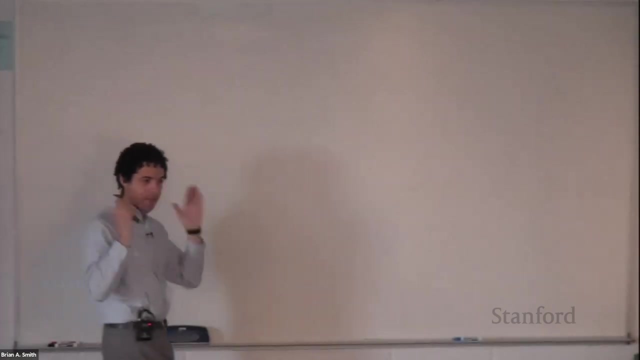 like that. So I think next up I'm going to show a quick video of the RAD in action. I'm going to move and try to move my personal lapel mic closer to the sound source so you can hear it. So you weren't hearing stereo, but it's stereo. 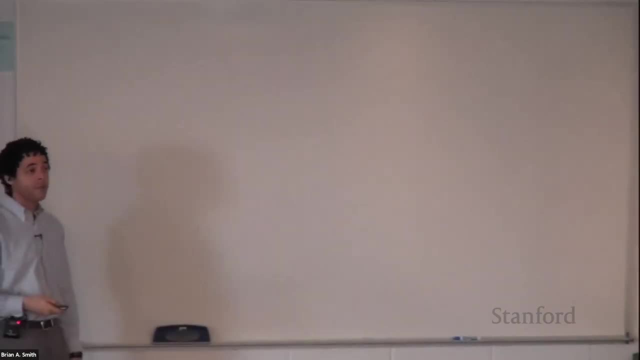 Sound is spatialized. And then I'll play a short clip from that player describing his experience playing a racing game- a real racing game- for the first time. So that particular player has been blind from birth, Sorry. before that, a couple of data points. 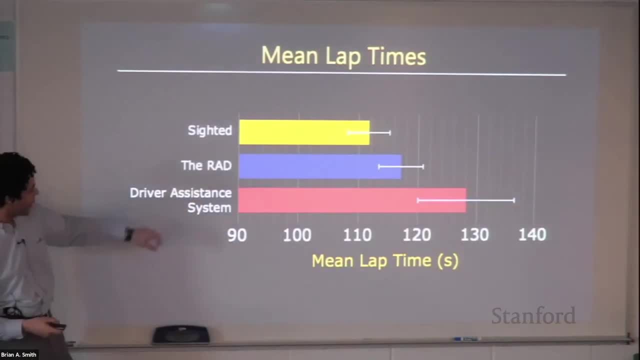 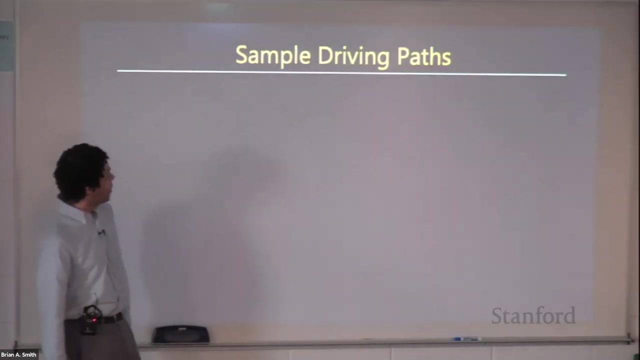 That's coming after the data. In terms of lap times, we actually found that the RAD, RAD, RAD Offered Players were able to drive laps in a comparable amount of time as sighted casual players In shorter times than a system that just called out. 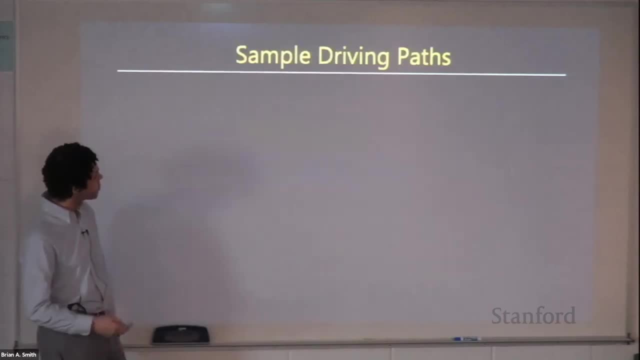 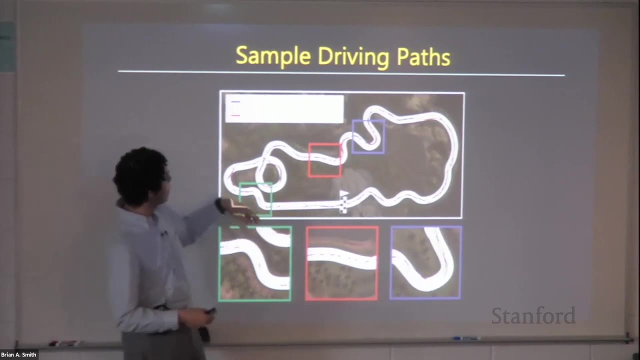 turn left, turn right, left right. That's what the red thing is. And then this one chart. before I show that other video, here are some actual driving paths. So the RAD is in blue And then the turn left, right. 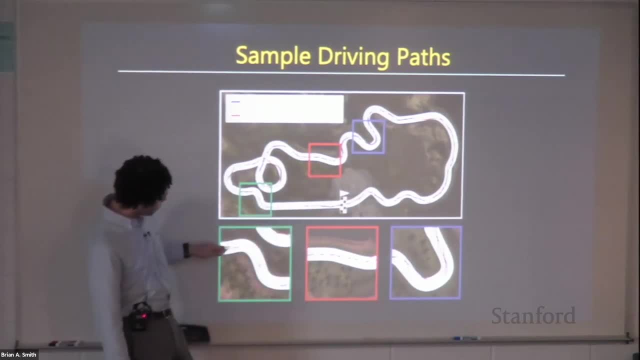 Left kind of system is in red, as you see, And you can see that the RAD allows the player to actually make some advanced racing maneuvers right. So obviously they're going straighter along this straightaway, But then they can thread the needle in this S turn. 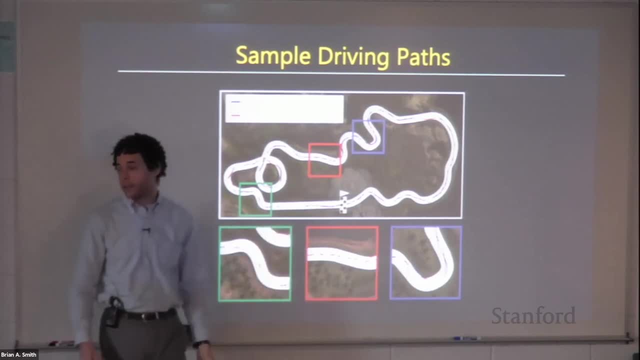 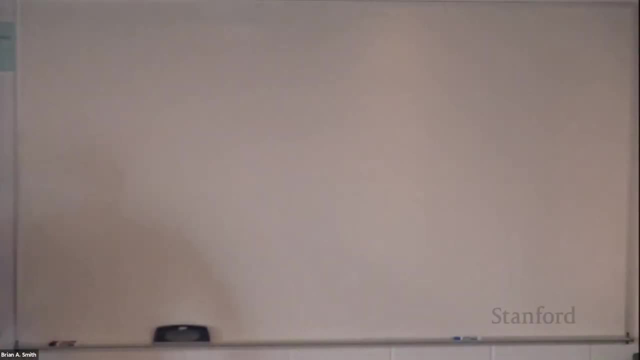 for example- And this was after just using the RAD for a few laps- They're able to form that intuition of what's going on with the track. OK, so here's the video. It was interesting to me. It was interesting to me. 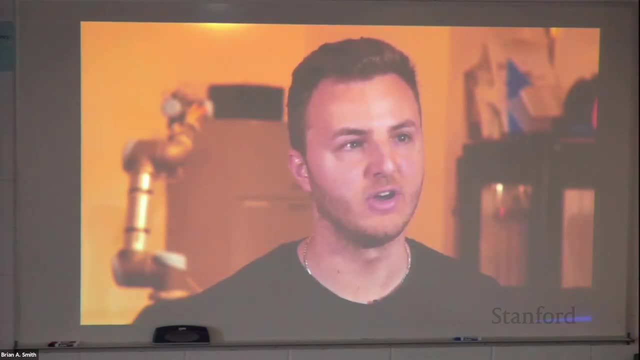 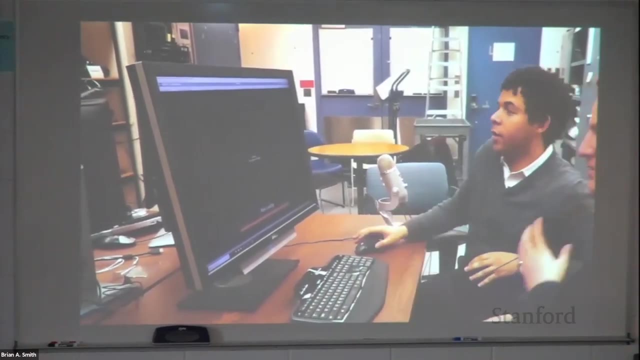 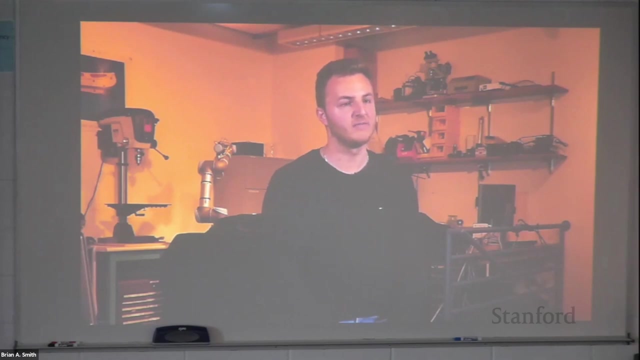 It was interesting to me. I tried the RAD because of the new experience that it gave to me, as a visually impaired person, in relation to playing racing games, This feeling of- I guess you can say- the feeling of adventure that it gave the sense of control. 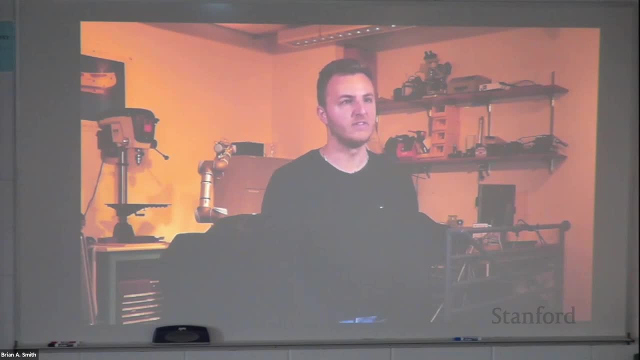 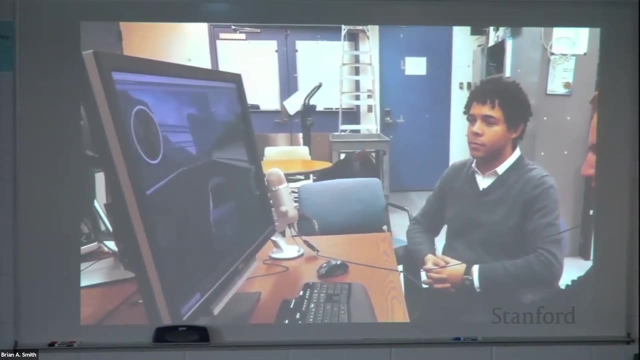 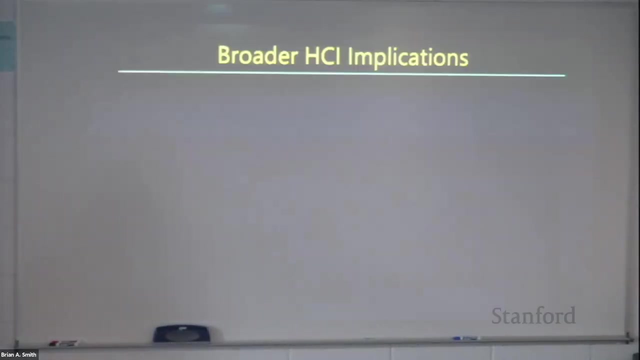 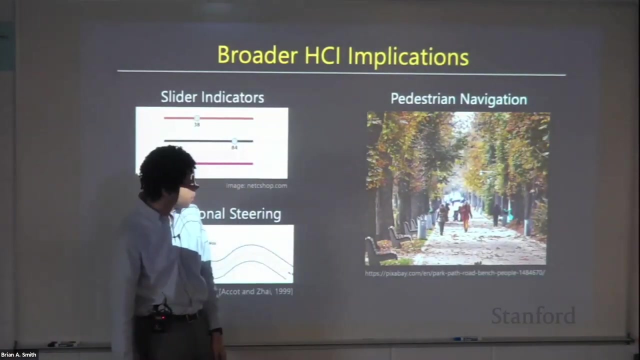 that it gave me as a player was totally different than what you would usually get from other audio racing games that were just designed for the visually impaired community. So the sound slider and the turn indicator system have some implications beyond games to HCI in general. So, for example, like in a pedestrian navigation system, 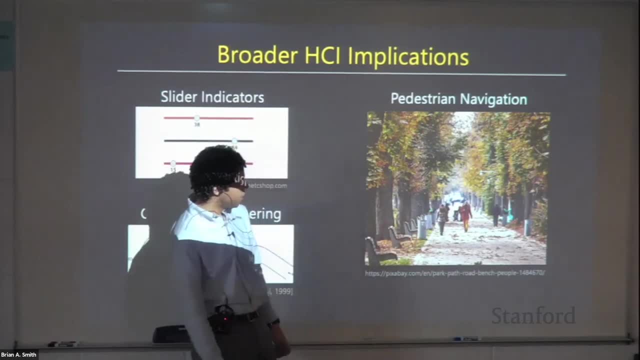 they can actually be used to help people who are blind, walk along a path and not only just follow a straight line along the path, But understand, Understand the path's width and maybe keep to the right side of that path. The way that sound sliders are defined. 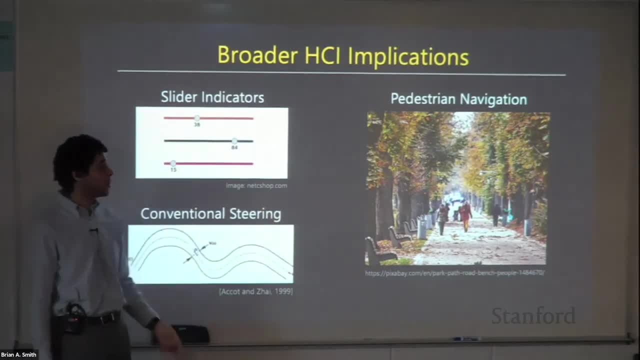 they're essentially these line segments in 3D space in the soundscape. They could be used as slider displays in general in general purpose UIs And then they can be used for any kinds of steering tasks in the classical sense to help some kind of user. 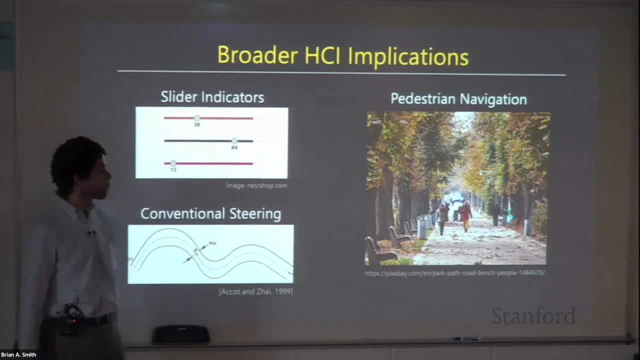 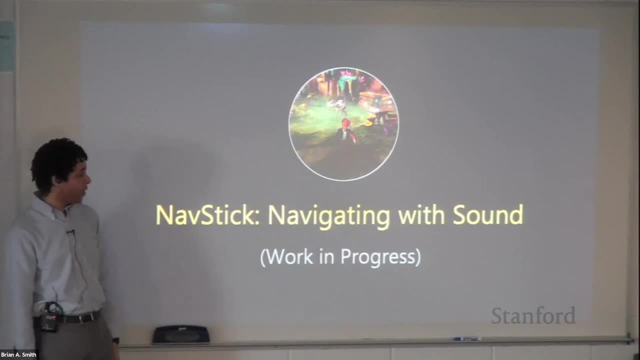 make a motion through some type of path or tunnel. Cool, So that work. the racing auditory display showed us that, in order to enable meaningful experiences, it's important to preserve meaningful choices right And so, rather like in order to enable equivalent experiences. 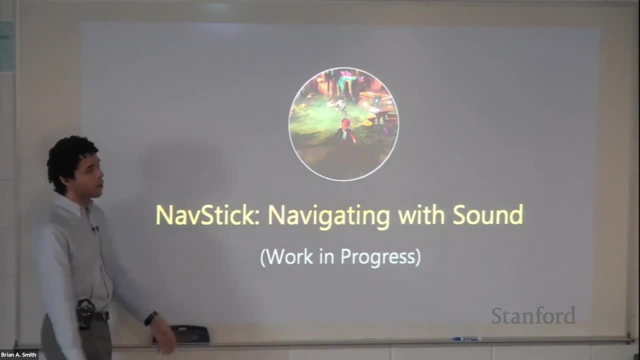 it's important to preserve meaningful choices, But the RAD only scratched the surface. Racing games is just one game genre. There are a lot of other genres, such as platformers, platforming games, action games, adventure games, RPGs, first person shooters, et cetera. 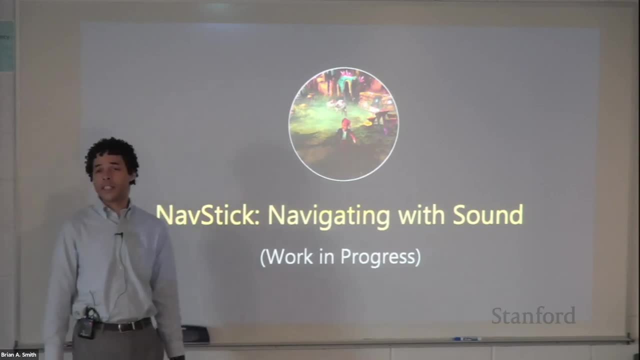 And then also the RAD sort of revealed the prospect of, with the pedestrian navigation stuff, promoting real world navigation as well and helping people better understand the real world as they're navigating as well, And so this is work that's still in progress, that we are doing in order to investigate. 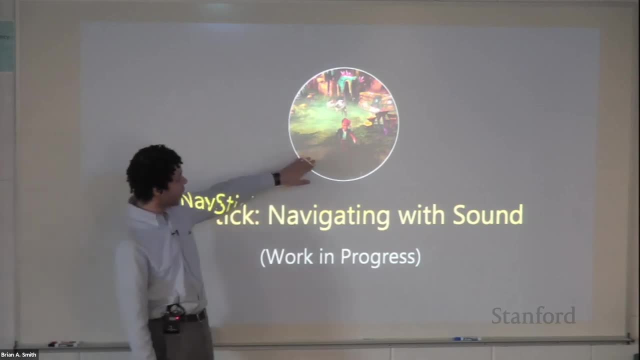 both of those realms, New genres. There's a lot of work to be done in order to make sure that we're able to make the best use of games. So in this case, this is an adventure game, an action adventure game. And then how do we build tools, widgets? 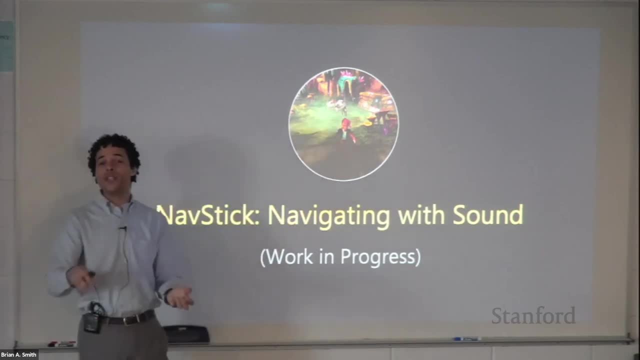 that can be used across games and maybe built into game engines to make these types of games playable. And then can those same widgets also give people more fulfilling experiences navigating in the real world, so they're not just following orders. So that's this project. 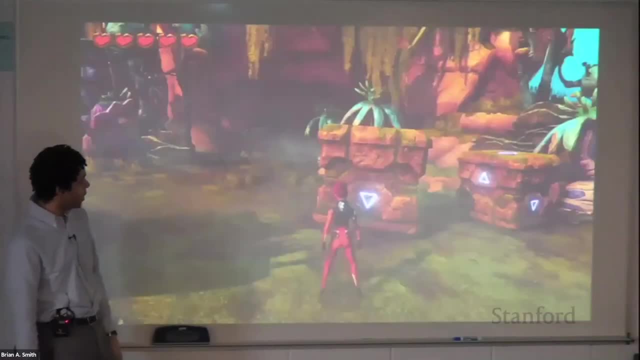 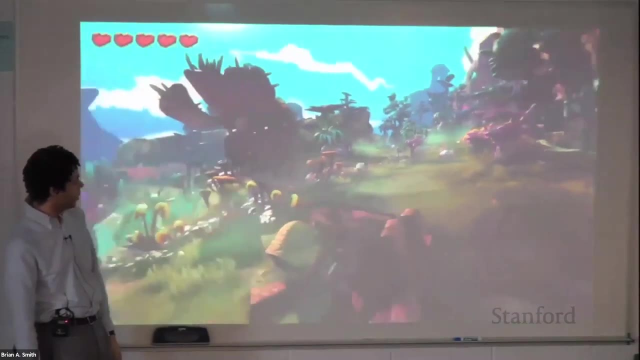 There's no sound here, but just to illustrate this action adventure game: you can move around, You can break crates- Every great game has to have crates- some enemies You can melee. You can also fire projectiles, that kind of thing. 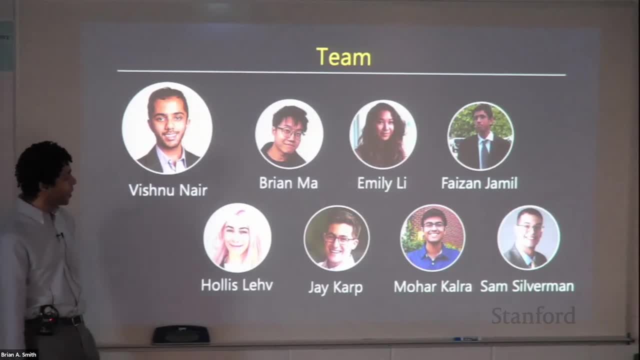 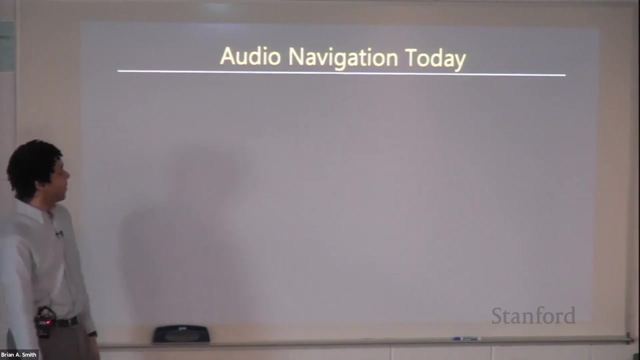 So this project is led by Vishnu Nair, my first PhD student- He's a second year now- And then as well, a team of undergraduate and master's students at Columbia. So let me start by talking about audio navigation today in the real world. 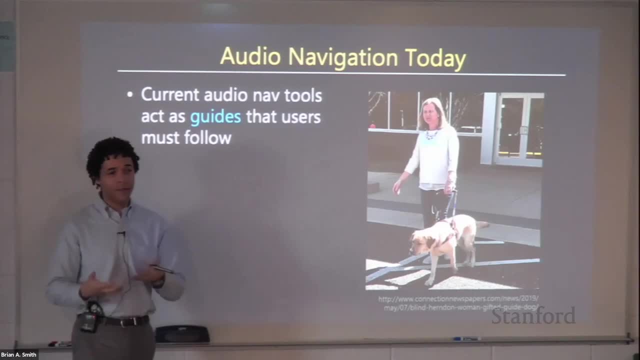 And it actually works the same way in existing adventure games and first-person shooters. Generally, these audio navigation tools act as guides that users must follow, So the prevailing analogy is that of a guide dog, where there's some kind of sound or some kind of tool. 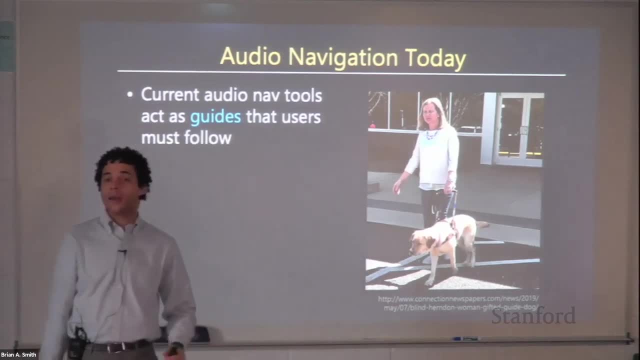 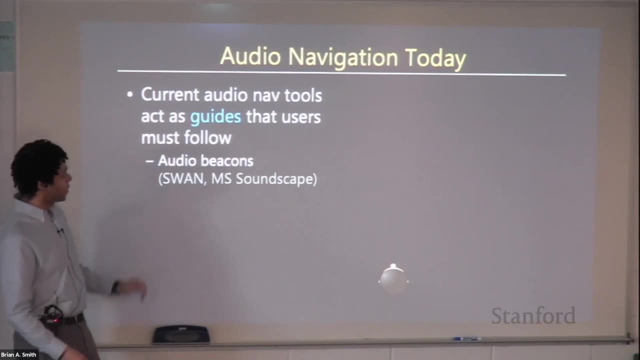 that tells the user which way to go And they just follow it wherever they're going. That's the analogy, And so a few common approaches. One is this concept of audio beacons. It's present in this system called SWAN, from Georgia Tech, Microsoft Soundscape. 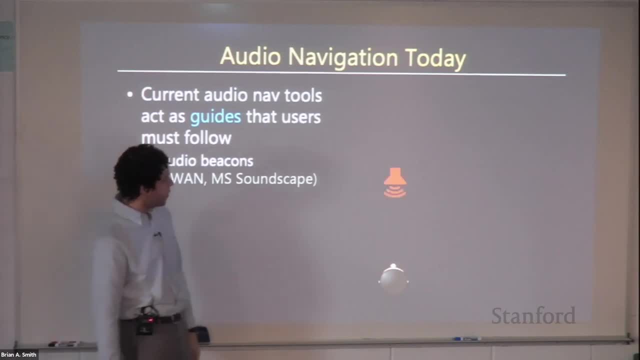 which is a really, really cool free mobile app, And the way that it works is that, essentially, the user hears this audio beacon, a siren call using spatialized sound from some point in space. They rotate themselves to center, They enter the sound and walk towards it. 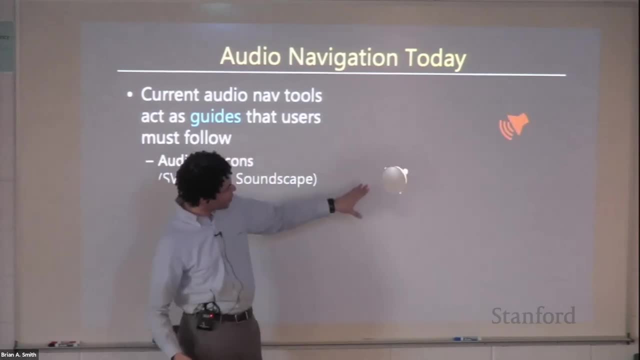 Once they do that, another sound will appear. They turn, they rotate and walk towards that one, And then they're just guided along a poly line some route to their destination. So that's audio beacons. So this is how people who are blind 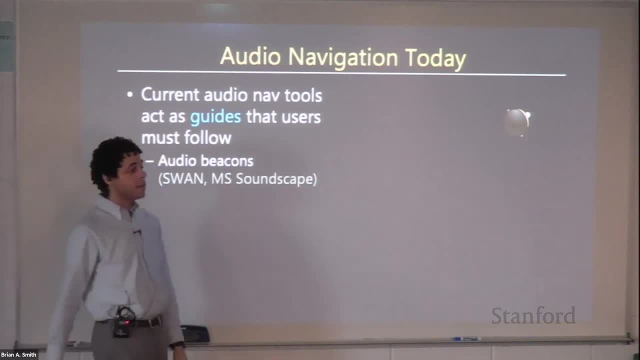 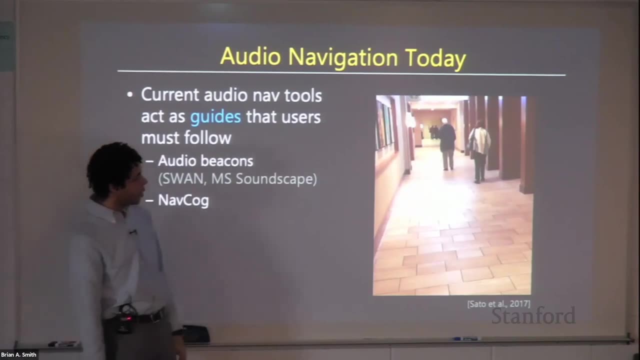 if they want to use an audio system such as Microsoft Soundscape to navigate to some place, that's how they do it. Another approach is NavCog. NavCog came out of Carnegie Mellon and IBM, And so, rather than using audio beacons, 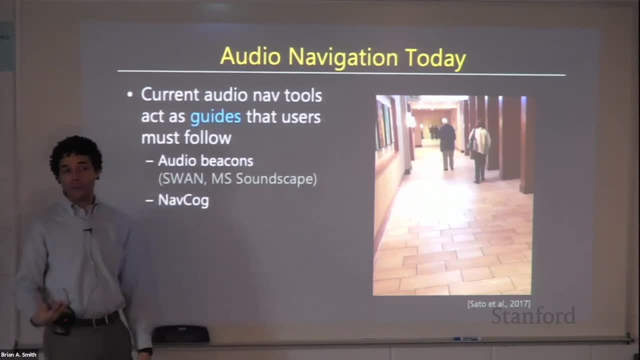 they're using the NavCog employees spoken prompts which tells the player or the user: walk 50 meters, turn left in 10 meters. OK, turn left now, keep turning, keep turning, OK, that kind of thing. So here I'm just going to play this short video. 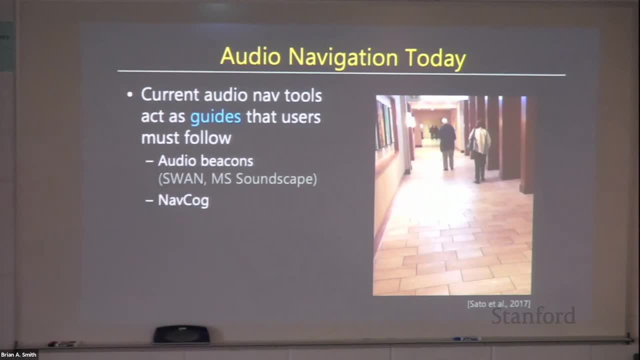 so you can hear what some of these prompts sound like. I'll step over here, Turn around. You might be going that way. Proceed 25 meters and turn right. OK, So that's NavCog spoken directions instead of beacons. 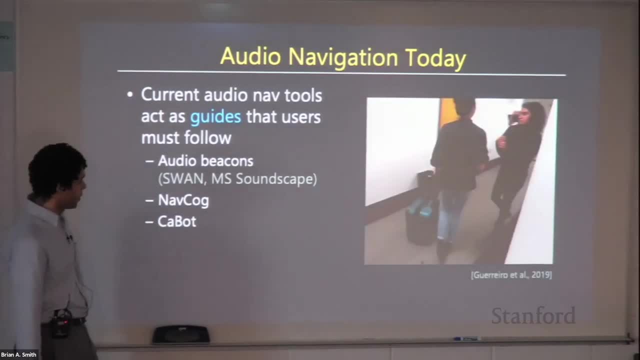 And then, third, we're seeing really interesting work. This is again from CMU called Cabot, And this really goes into this guide dog analogy. What we have here is a suitcase that can move itself along, and it has a depth camera attached to it. 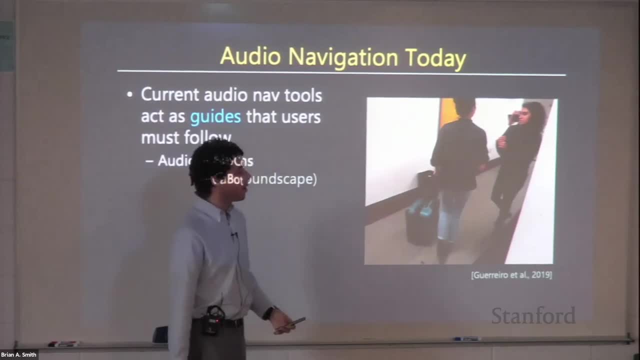 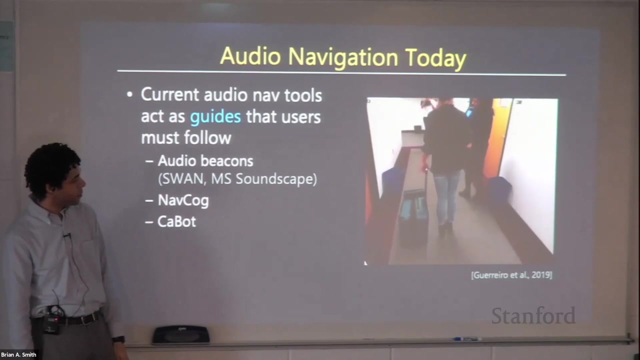 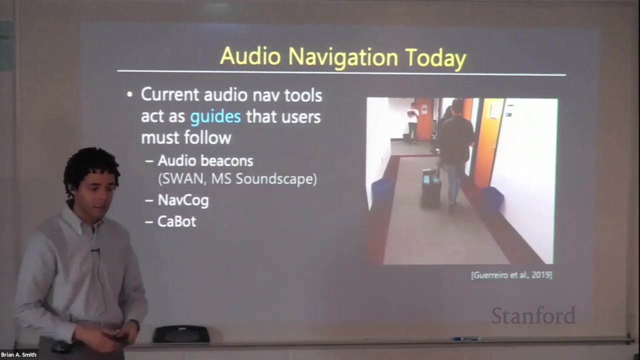 OK. So this suitcase will actually guide the user and the user simply just kind of follows the suitcase And it also checks for obstacles along the way. So here's a quick little video of Cabot. So it's kind of tugging the user along. 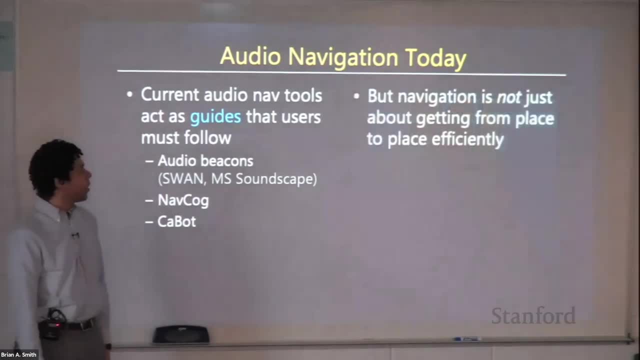 It's kind of dragging the user along, But our observation is that, OK Again, when we're thinking about equivalent experiences, people who are sighted do not. Navigation is not just about getting from point A to point B efficiently, right. 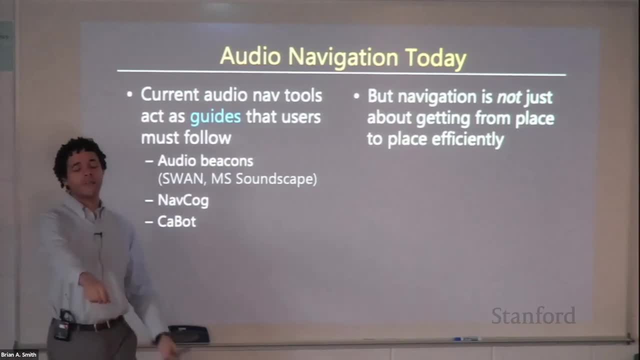 It's about a lot more. It's not just about closing your eyes and having someone take you there. OK, you have arrived. It's about a lot more than that. It's about surveying one's surroundings, kind of knowing where they are, enjoying the space itself. 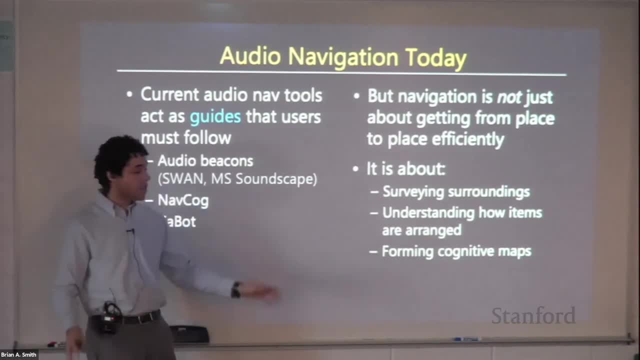 the journey along the way, understanding how items are arranged in a space, forming mental maps, cognitive maps of the space. right, It's about a lot more than search this idea of just going from point A to point B, And so, in short, navigation is about looking around. 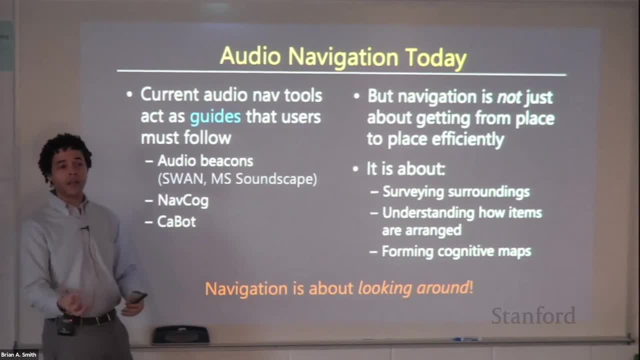 And so if there's one ability that can unlock agency in navigation, it's the ability to look around. If you can provide that, well then actually, users would be able to navigate themselves in a very fulfilling way, rather than just being guided, And so NavStick is an instrument for looking around. 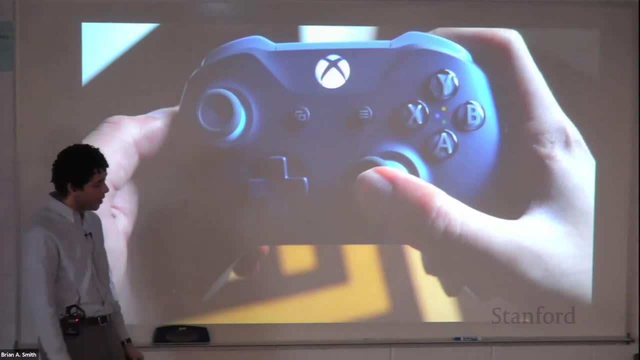 And the way that it works- and so far we've prototyped it for games- is it repurposes the right analog stick into an instrument for looking around. Essentially, the user will tilt the stick in order to look around in that direction with respect to them. 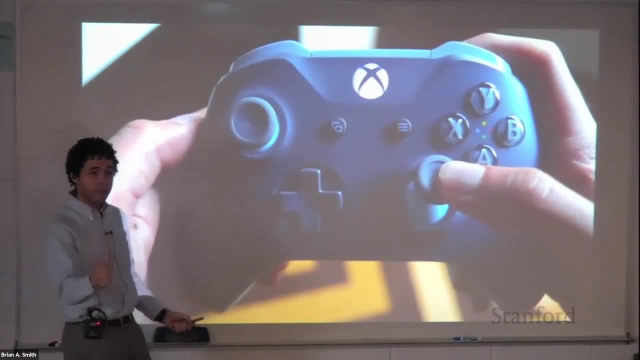 So if you tilt it to the right, you're checking out your 3 o'clock. If you tilt it forward, it's your 12 o'clock, So you can very, very quickly survey what's around you as you go in the game. 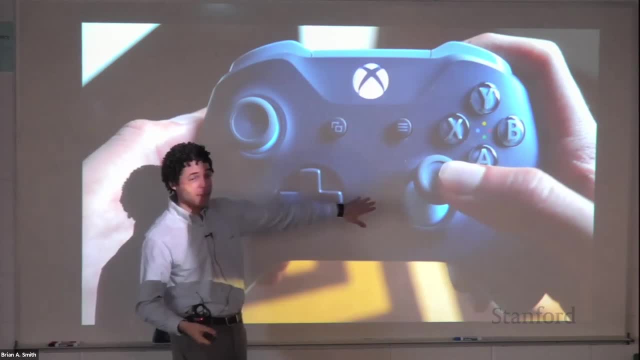 Most adventure games and first-person shooters reserve the right stick for camera controls. But if you're blind, you don't need the camera, So we can repurpose it into an instrument for looking around. It's a simple idea, but what's interesting about this idea? 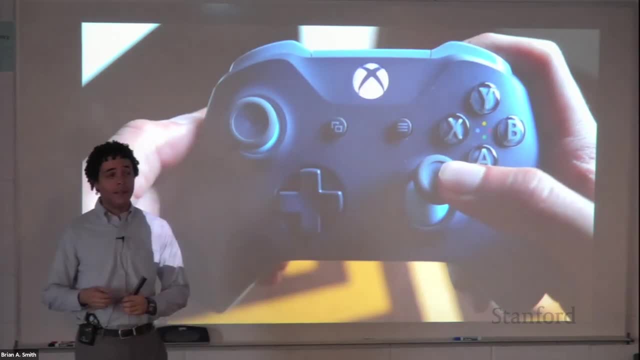 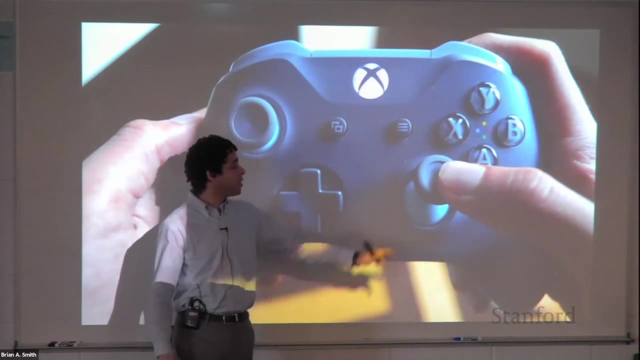 is that it enables on-demand and random access to directional information. It's on-demand. It's on-demand because users aren't just being spoken to the entire time, especially when they don't want to hear speech or hear that siren sound, The only time that they'll ever hear a sound. 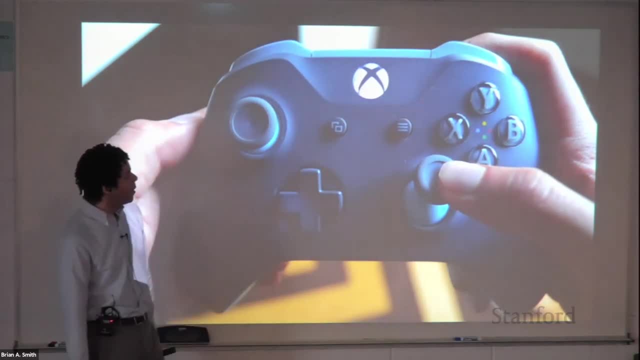 is when they tilt the stick. They get to control that And it's random access because they can probe any direction just by tilting the stick in that direction. There's constant time to look around regardless of direction. So here I'm going to show NavStick in a growth. 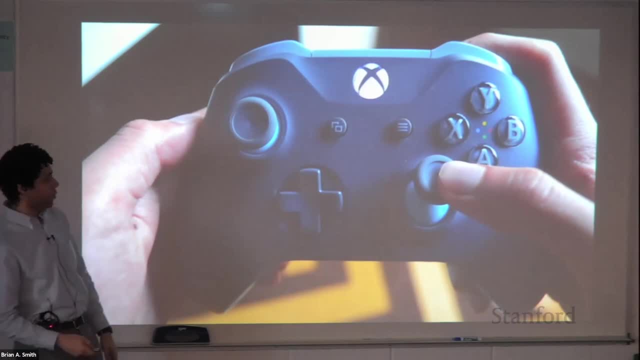 grocery store environment that we created. I'll explain why we created this grocery store in a minute. It's essentially to test NavStick, not only in that adventure game context, but also in the context of real-world navigation, thinking about environments in which people might want to find things. 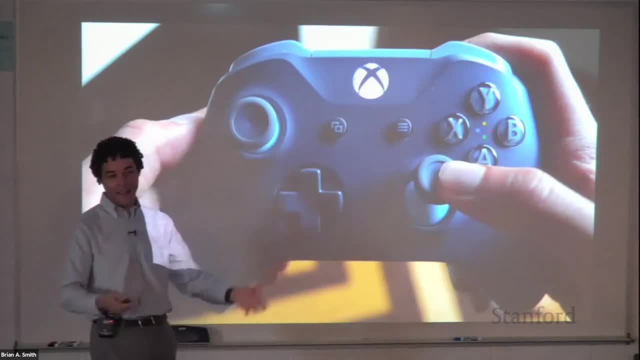 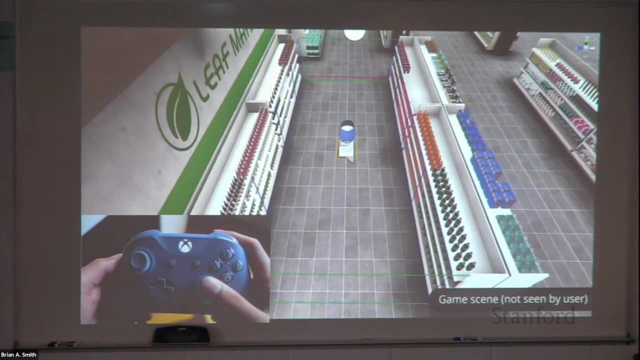 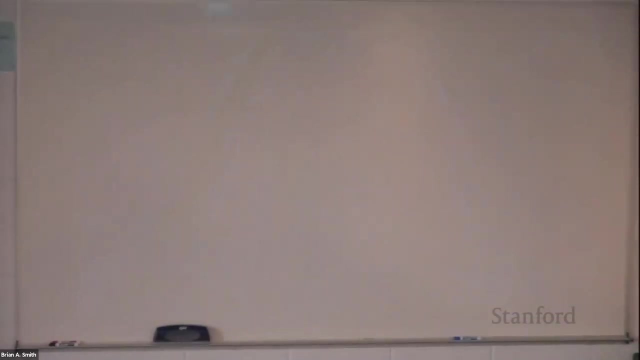 and explore and remember where things are and compare items. That's the grocery store. So here's NavStick in action. I'm going to move so you can actually hear. OK, So that was a quick one, And so we asked a few research questions. 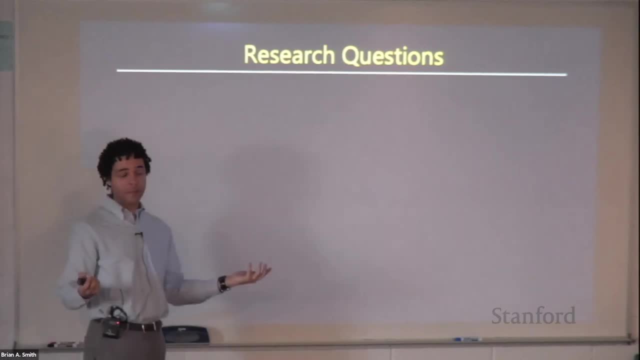 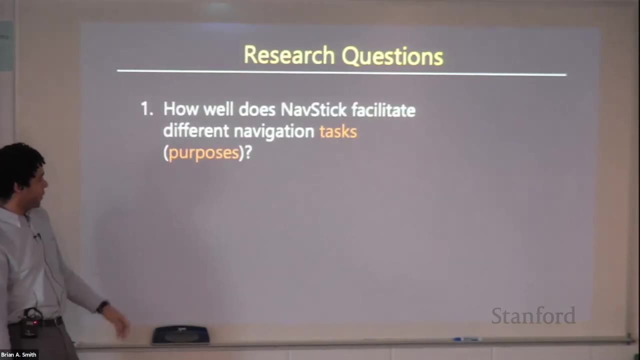 around NavStick, giving people this ability to look around in spaces which, surprisingly, isn't present right now. Number one: how well does NavStick facilitate different navigation tasks or purposes? So by navigation tasks I mean search, getting from point A to point B. But 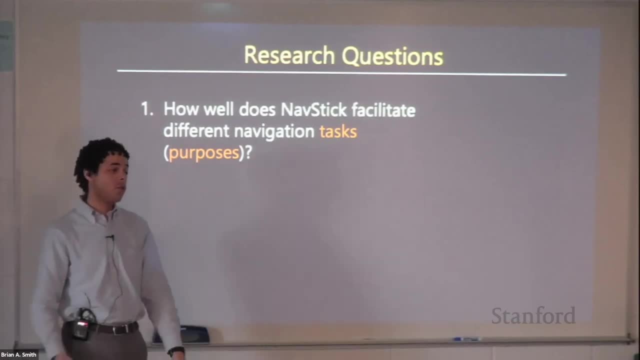 also exploration, forming cognitive maps, or comparison, comparing different pathways. we draw from, from psychology here, in terms of right, the purposes that you know, navigation being an overloaded term and there are actually many different purposes for navigation. so we want to, we want to understand how well nav stick. 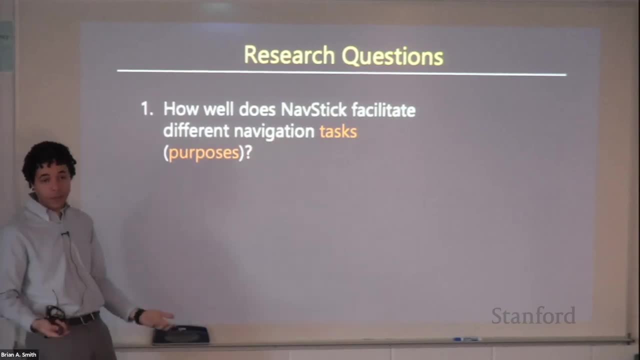 serves these different purposes. if it is going to become an instrument for navigation, a widget that we use across you eyes to, we want to understand how well does nav stick facilitate different navigation environments? so game environments, clutter, density, occlusion, that kind of thing. and then three: how? 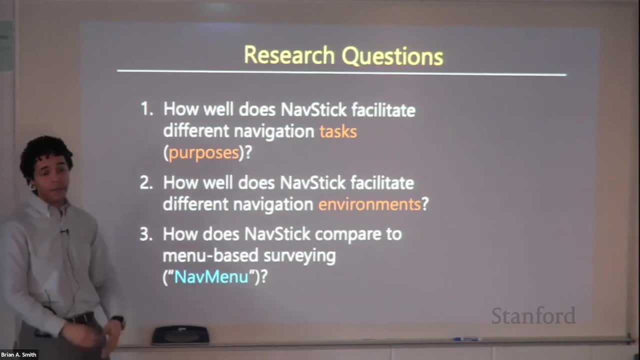 does nav stick compared to menu based, surveying this idea of just having a hierarchical menu of targets that people can select, grocery store items, for example. and you know, maybe it's alphabetized or sorted by distance, so I'll show just a. you know, maybe it's alphabetized or sorted by distance, so I'll show just a. 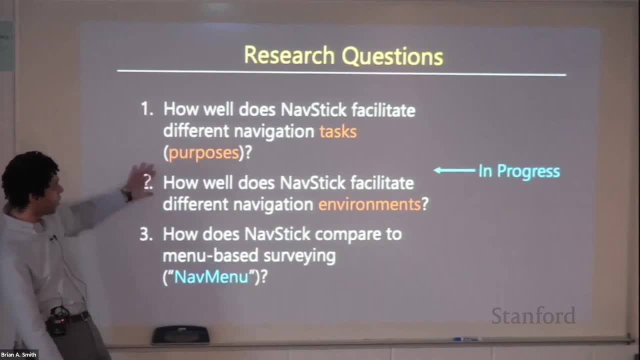 you know, maybe it's alphabetized or sorted by distance. so I'll show just a couple of results here. and number two, by the way: how well does nav stick facilitate in different environments? this is still in progress and we're testing this in that video, that adventure video game environment. so we 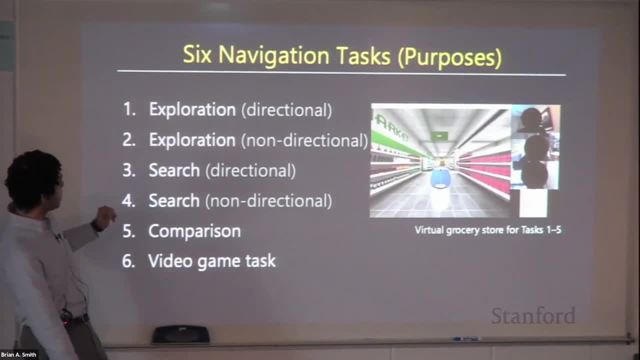 had six different navigation tasks. I won't go into this, but essentially we talked about exploration, search, comparison and even playing games where agency is more important in navigation. by directional I mean cases in which agency is more important in navigation. by directional I mean cases in which agency is more important in navigation. by directional I mean cases in which knowing the direction of something is. 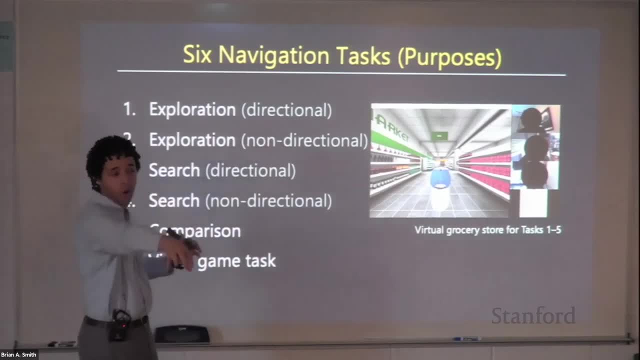 knowing the direction of something is. knowing the direction of something is important. so, for example, I want to important. so, for example, I want to important. so, for example, I want to remember that the milk is in this corner. remember that the milk is in this corner. remember that the milk is in this corner of the aisle as opposed to just in the. 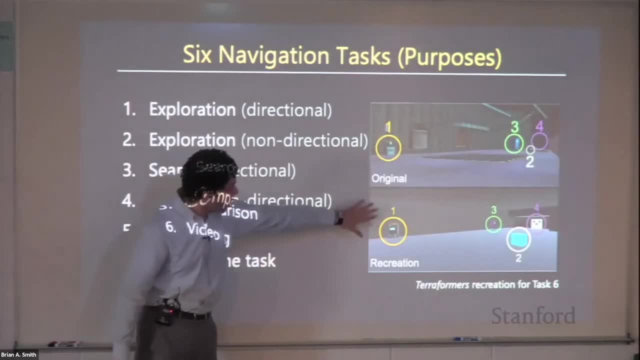 of the aisle, as opposed to just in the of the aisle, as opposed to just in the aisle period, and this is like this video aisle period and this is like this video aisle period and this is like this video game environment. another one: this is an game environment. another one: this is an. 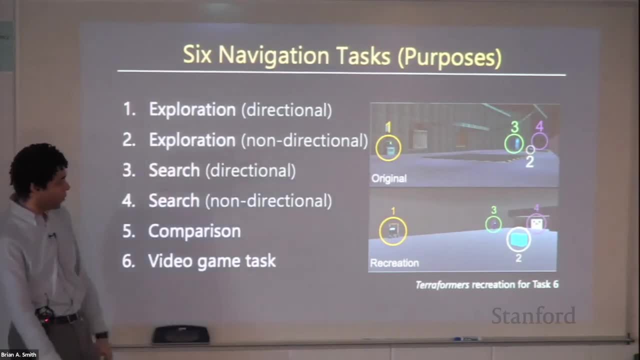 game environment. another one: this is an act. this is actually a first-person act. this is actually a first-person act. this is actually a first-person shooter that we recreated and we found shooter that we recreated and we found shooter that we recreated and we found that participants actually enjoy having 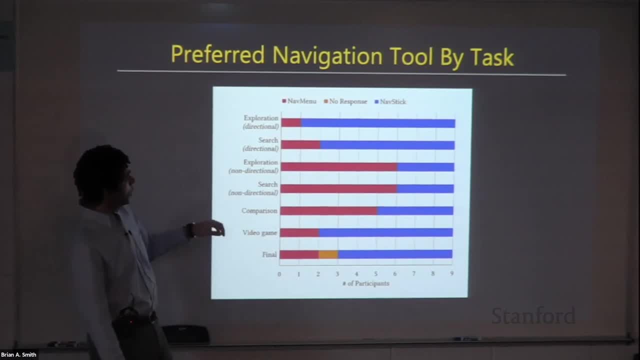 that participants actually enjoy having that participants actually enjoy having both a menu based navigation tool to both, a menu based navigation tool to both, a menu based navigation tool to get from point A to point B. and nav stick. get from point A to point B and nav stick. 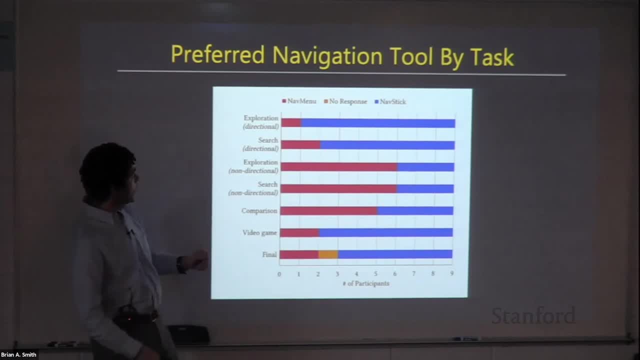 get from point A to point B and nav stick to explore and look around. and they make to explore and look around, and they make to explore and look around, and they make that choice based on whether they would that choice, based on whether they would that choice, based on whether they would like to navigate directionally, whether 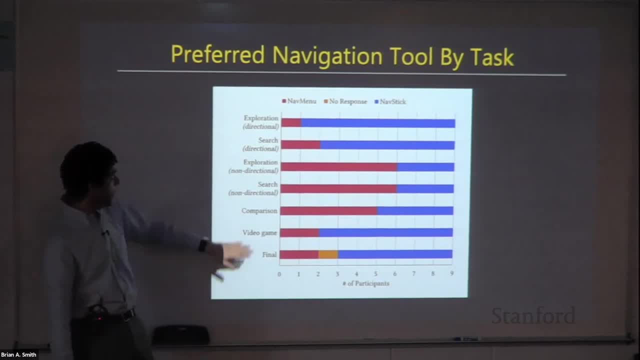 like to navigate directionally, whether like to navigate directionally, whether directions important and whether or not directions important, and whether or not directions important and whether or not they are, for example, playing a game. they are, for example, playing a game. they are, for example, playing a game and in the context of a game where people 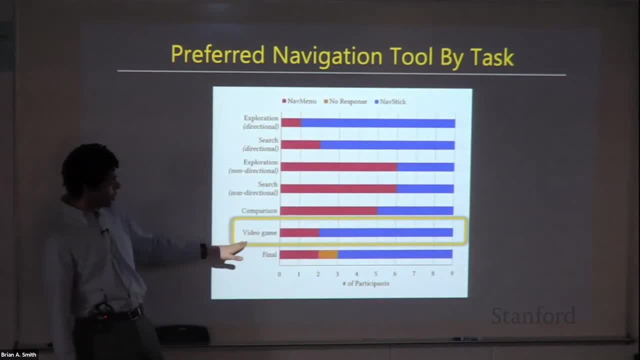 and in the context of a game where people and in the context of a game where people predominantly preferred nav stick, they predominantly preferred nav stick. they predominantly preferred nav stick. they preferred this, even though they also preferred this, even though they also preferred this, even though they also agreed that nav stick took a lot of extra. 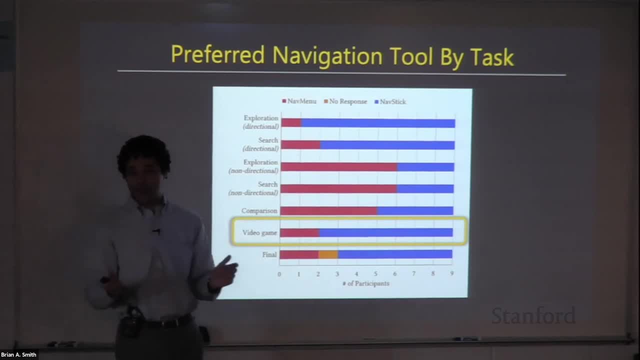 agreed that nav stick took a lot of extra. agreed that nav stick took a lot of extra effort for the game actually looking effort for the game actually looking effort for the game actually looking around and doing things themselves was around and doing things themselves was around and doing things themselves was the whole point of the game to them. they 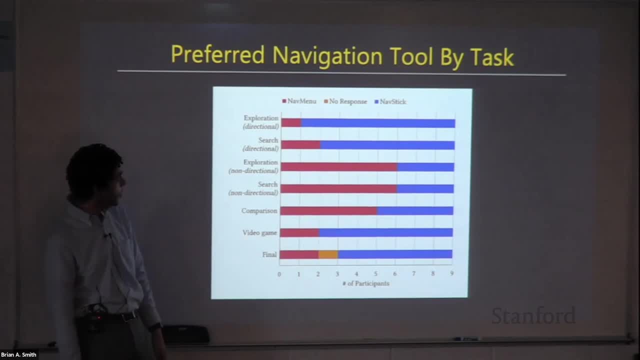 the whole point of the game to them. they the whole point of the game to them. they really enjoyed that a lot. so I'm going really enjoyed that a lot. so I'm going really enjoyed that a lot. so I'm going to show one more result about mental. 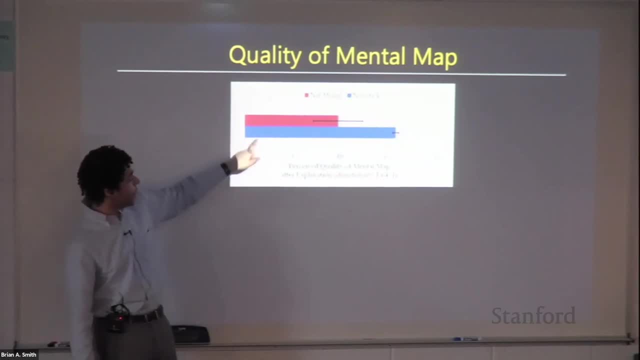 to show one more result about mental. to show one more result about mental maps. people actually felt that they were maps. people actually felt that they were maps. people actually felt that they were able to form better mental maps of their, able to form better mental maps of their. 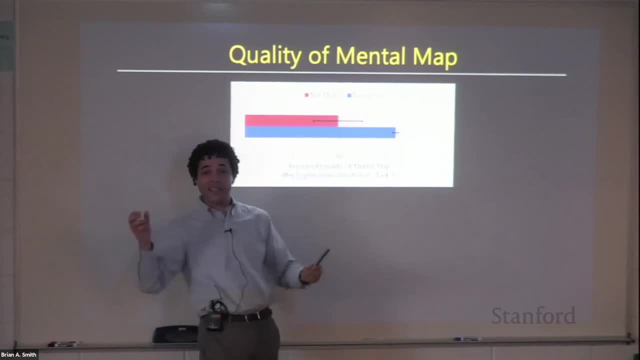 able to form better mental maps of their spaces with nav stick compared to using spaces with nav stick, compared to using spaces with nav stick, compared to using a menu and hearing where these things a menu and hearing where these things a menu and hearing where these things are from a menu. and they agreed very 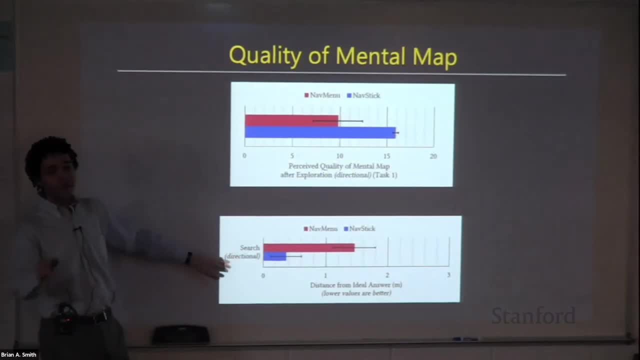 are from a menu and they agreed very are from a menu and they agreed very small confidence interval. and then we small confidence interval, and then we small confidence interval, and then we quiz them. we put them in random grocery, quiz them. we put them in random grocery, quiz them. we put them in random grocery store aisles and say you know? and said 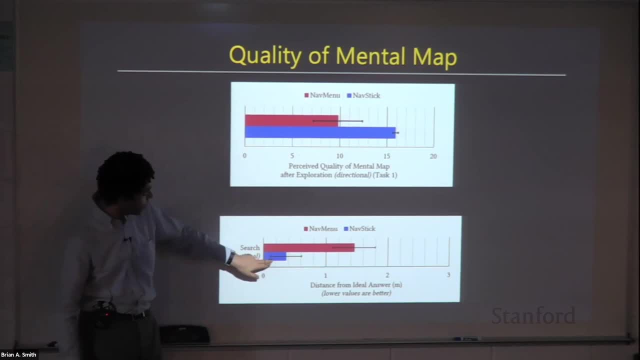 store aisles and say you know, and said store aisles and say you know, and said okay, so where's the peanut butter? and we okay, so where's the peanut butter? and we okay, so where's the peanut butter? and we found that people performed much better. 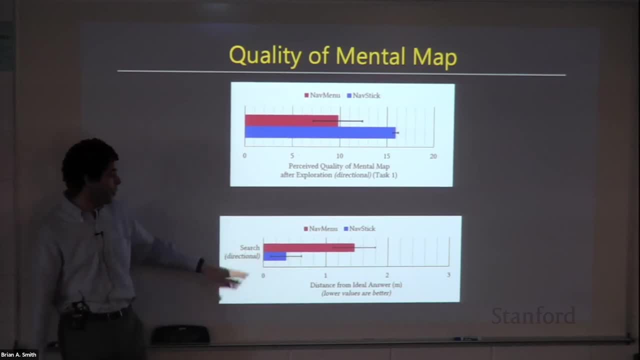 found that people performed much better. found that people performed much better when they were able to explore first. when they were able to explore first, when they were able to explore first with nav stick, then when they use the with nav stick, then when they use the with nav stick, then when they use the menu. okay, so let me go on into future. 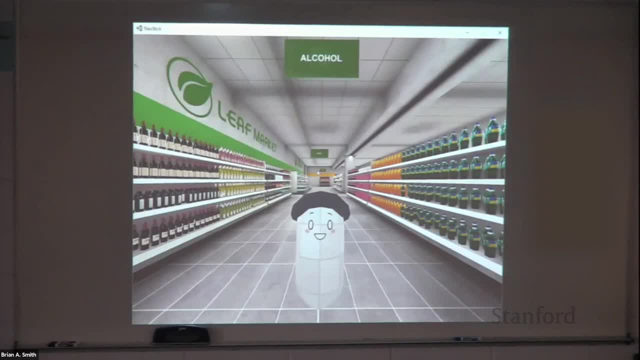 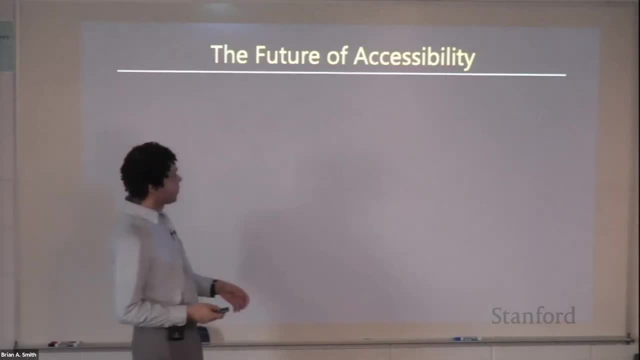 menu. okay, so let me go on into future menu. okay, so let me go on into future work. okay, so in the future, you know the work. okay, so in the future, you know the work. okay, so in the future, you know the way, that way, that way, that that you know we're thinking about the. 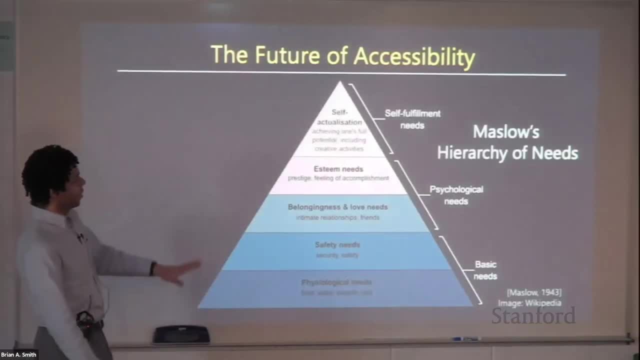 that you know we're thinking about the. that you know we're thinking about the next couple of years, and and next couple of years, and and next couple of years, and and accessibility at large. is is related to accessibility at large. is is related to accessibility at large. is is related to maslow's hierarchy of needs, right. so 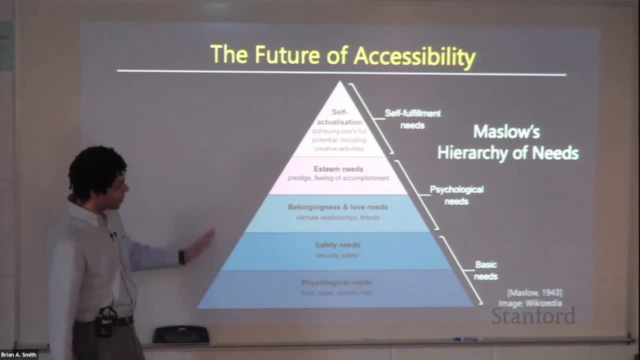 maslow's hierarchy of needs. right. so maslow's hierarchy of needs, right. so this is how i. this is how i. this is how i think about accessibility. maslow's think about accessibility. maslow's think about accessibility. maslow's hierarchy starts with basic needs. on: 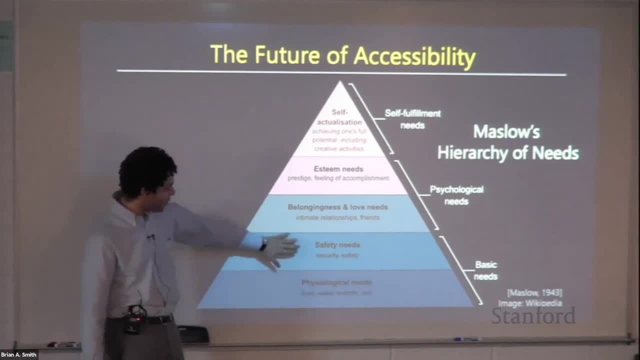 hierarchy starts with basic needs on. hierarchy starts with basic needs on the bottom, the bottom, the bottom, food, water, shelter, that kind of thing. food, water, shelter, that kind of thing. food, water, shelter, that kind of thing, safety needs, and then it moves on up: safety needs, and then it moves on up. 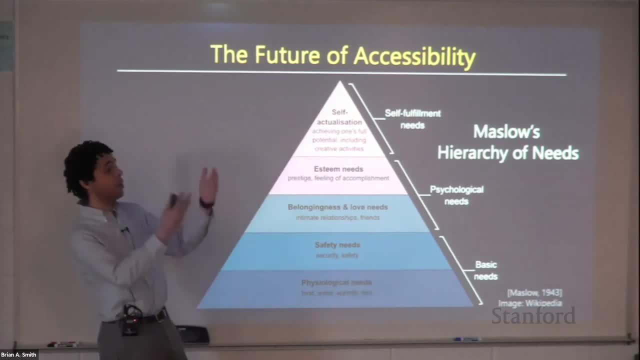 safety needs, and then it moves on up into self-fulfillment needs. achieving into self-fulfillment needs, achieving into self-fulfillment needs achieving one's full potential, including creative one's full potential, including creative one's full potential, including creative activities. 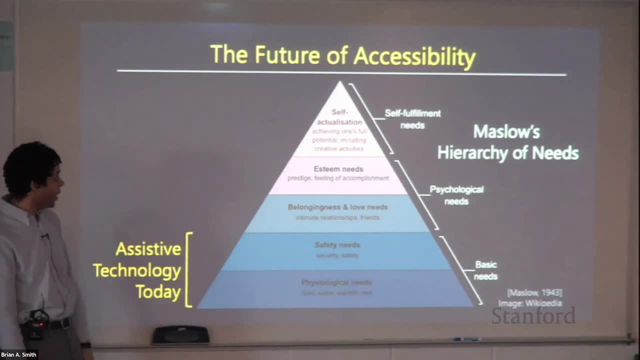 activities. activities right if you look at most. right if you look at most right if you look at most. accessibility research today. accessibility research today. accessibility research today. it's down here at the bottom of the. it's down here at the bottom of the. it's down here at the bottom of the pyramid. 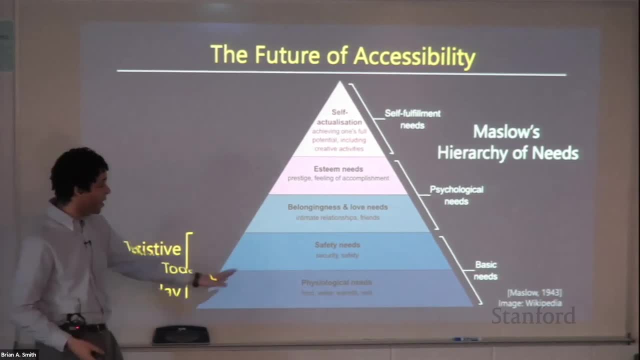 pyramid pyramid really focused on just providing basic, really focused on just providing basic, really focused on just providing basic access. making things access. making things access, making things possible. fulfilling basic needs right possible. fulfilling basic needs right possible. fulfilling basic needs right. you might think of it in terms of: 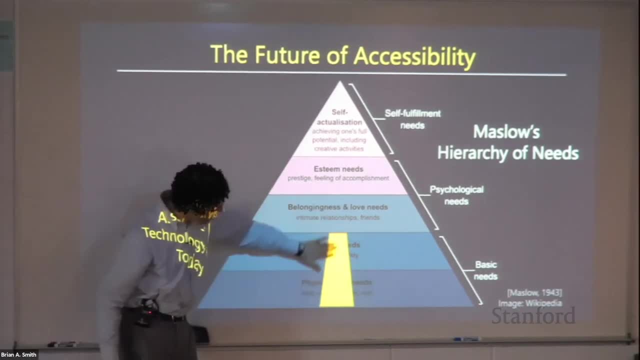 you might think of it in terms of. you might think of it in terms of actually this, this wedge where we're actually this, this wedge where we're actually this, this wedge where we're fulfilling these basic needs. fulfilling these basic needs, fulfilling these basic needs and a lot of accessibility. 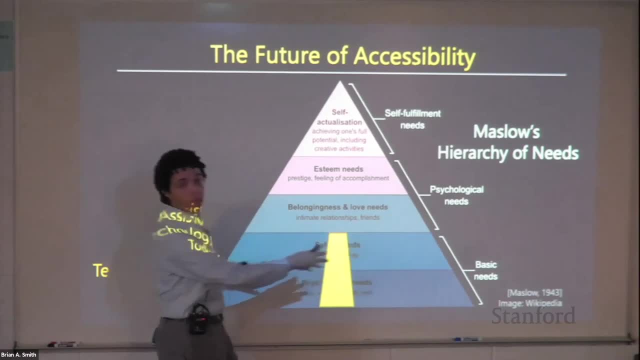 and a lot of accessibility and a lot of accessibility. work is trying to figure out other work is trying to figure out other work is trying to figure out other basic needs, basic needs, basic needs: that that that need to be fulfilled. that that that need to be fulfilled. 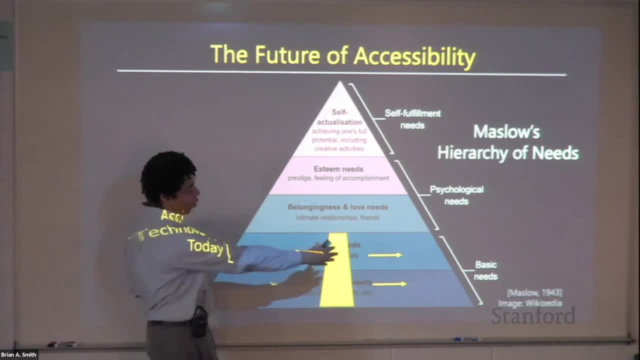 that that that need to be fulfilled. it's a continuing journey. it's a continuing journey. it's a continuing journey, so we're kind of just expanding outward. so we're kind of just expanding outward, so we're kind of just expanding outward in accessibility research, in accessibility research. 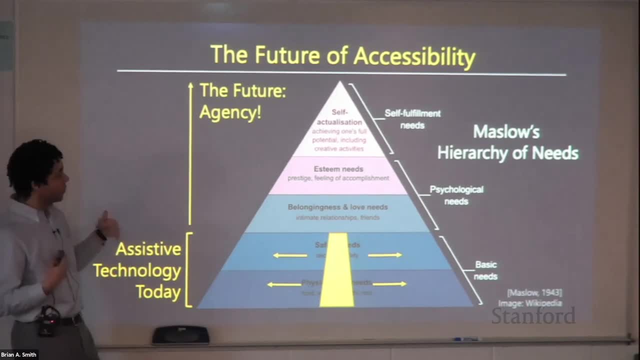 in accessibility research. but we at the lab like and this is, but we at the lab like and this is, but we at the lab like and this is, and this is also what i believe, uh think, and this is also what i believe, uh think, and this is also what i believe, uh think that the future is in. 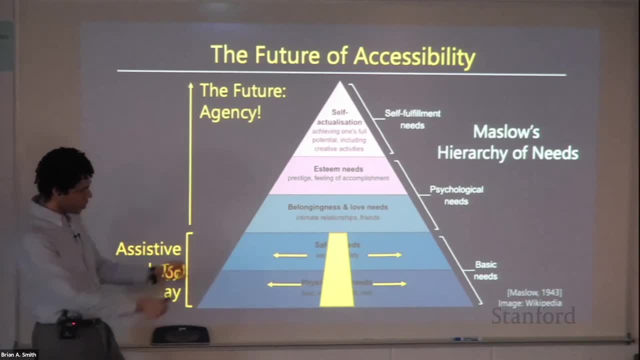 that the future is in, that the future is in agency right accessibility accessibility. agency right accessibility accessibility. agency right accessibility accessibility system shouldn't just be building system. shouldn't just be building system, shouldn't just be building outward and serving more basic needs of outward and serving more basic needs of. 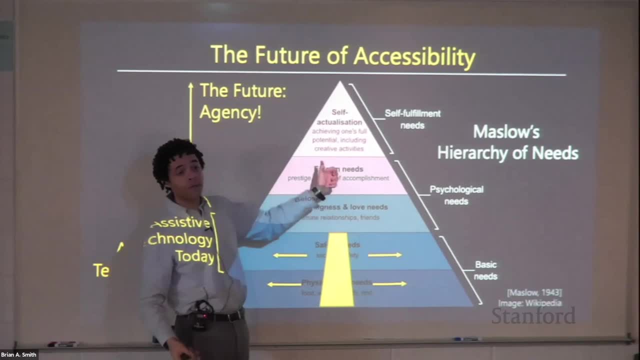 outward and serving more basic needs. of course that's super important, course, that's super important, course that's super important. but we need to be thinking about, but we need to be thinking about, but we need to be thinking about creating equivalent experiences as well, creating equivalent experiences as well. 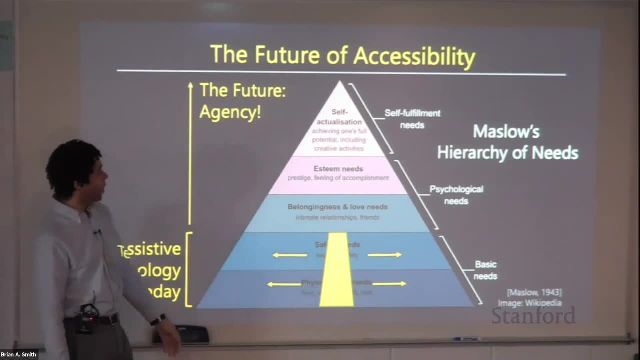 creating equivalent experiences as well, and not you know creating these glass and not you know creating these glass and not you know creating these glass. ceilings for users, ceilings for users, right. so the future is building up um in right. so the future is building up um in right. so the future is building up um in new york. we like to build up. 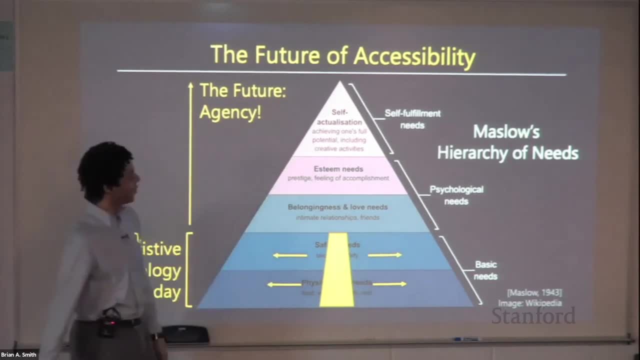 new york. we like to build up new york. we like to build up uh, and so i think uh, and so we're doing uh, and so i think uh, and so we're doing uh, and so i think uh, and so we're doing a lot of work. 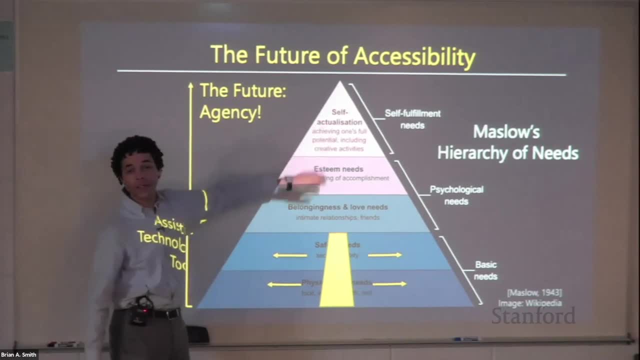 a lot of work, a lot of work, um in terms of uh helping people have, um in terms of uh helping people have, um in terms of uh helping people have these equivalent experiences, these equivalent experiences, these equivalent experiences, and the sense of agency and self-worth and the sense of agency and self-worth. 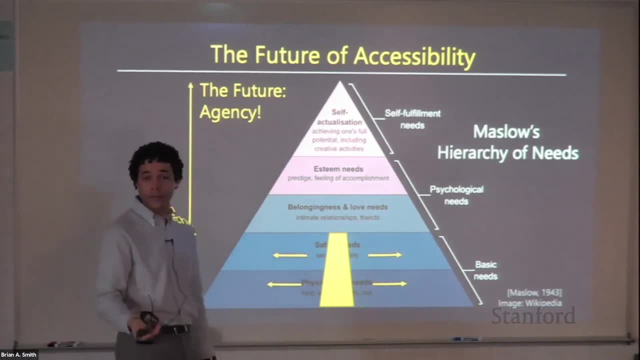 and the sense of agency and self-worth, and this feeling of yes, i did it. and this feeling of yes, i did it, and this feeling of yes, i did it instead of i'm just following the instead of i'm just following the instead of i'm just following the system's orders. 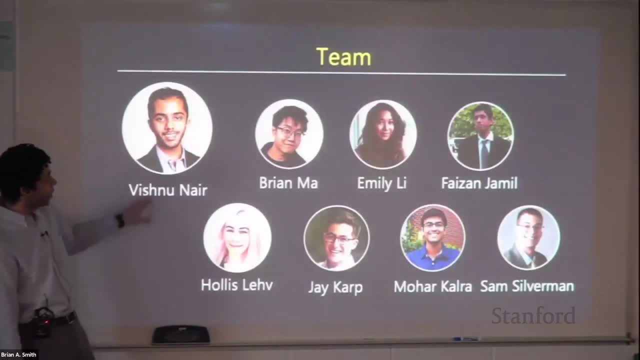 system's orders, system's orders, and so with navstick, um, you know this. and so with navstick, um, you know this. and so with navstick, um, you know, this is ongoing work. again i showed you the is ongoing work. again i showed you the is ongoing work. again i showed you the team. 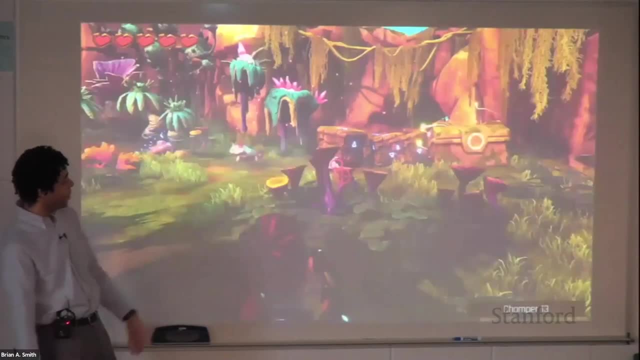 team, team. um we uh actually prototype navstick in um we uh actually prototype navstick in um we uh actually prototype navstick in this video game. this video game, this video game allowing users to you know shoot enemies. allowing users to you know shoot enemies. allowing users to you know shoot enemies, walk around. we're doing a whole bunch of. 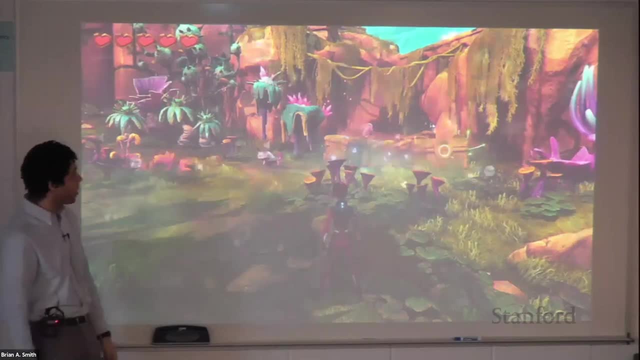 walk around. we're doing a whole bunch of walk around. we're doing a whole bunch of experiments there, experiments there, experiments there. we'll be releasing stuff. we want to. we'll be releasing stuff. we want to. we'll be releasing stuff. we want to make all this stuff open source. 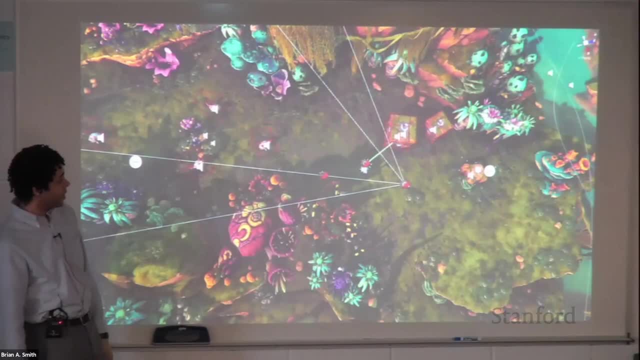 make all this stuff open source. make all this stuff open source. here's a top down view of the kinds of: here's a top down view of the kinds of: here's a top down view of the kinds of stuff we're doing with navstick. stuff we're doing with navstick. 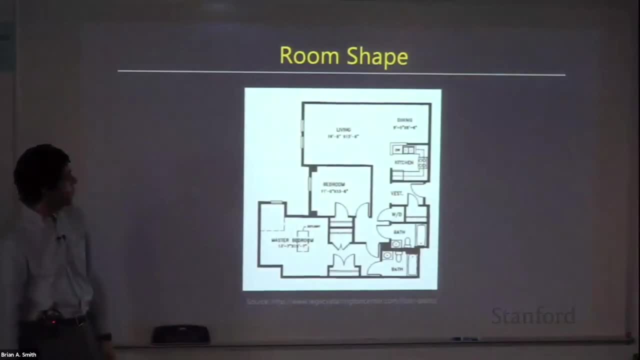 stuff we're doing with navstick and adventure games and moving on to and adventure games, and moving on to and adventure games and moving on to other genres of games, other genres of games, other genres of games. we're also thinking about how to very. we're also thinking about how to very. 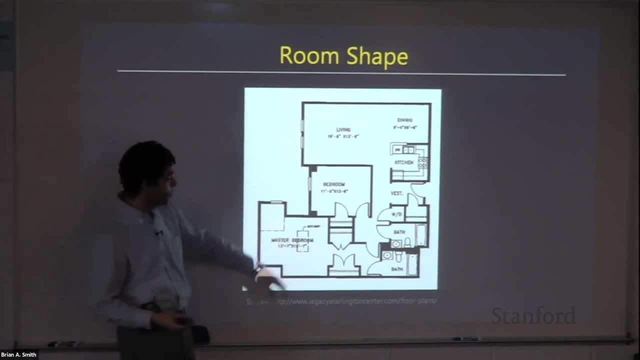 we're also thinking about how to very quickly communicate the shapes of rooms, quickly communicate the shapes of rooms, quickly communicate the shapes of rooms and layouts to people and layouts to people and layouts to people. using sound right, you walk into a room. using sound right, you walk into a room. 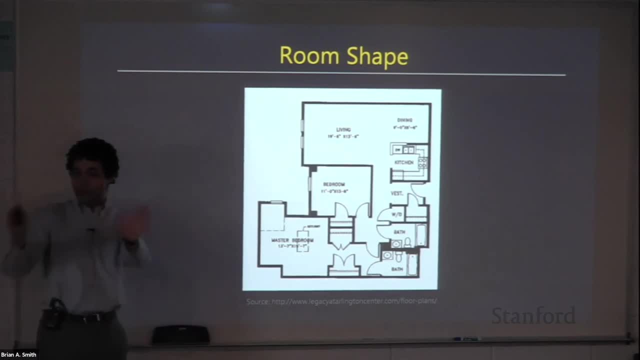 using sound. right, you walk into a room or a hallway, if you have sight, you can. or a hallway, if you have sight, you can. or a hallway, if you have sight, you can. very quickly perceive the general, this very quickly perceive the general, this very quickly perceive the general, this general sense of shape, how can we do? 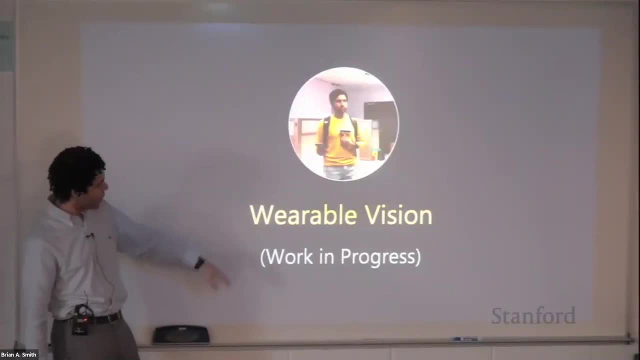 general sense of shape. how can we do general sense of shape? how can we do that without sight, that without sight, that without sight? and then my other phd student, garov, and then my other phd student, garov, and then my other phd student, garov, jane, is leading a project which we're. 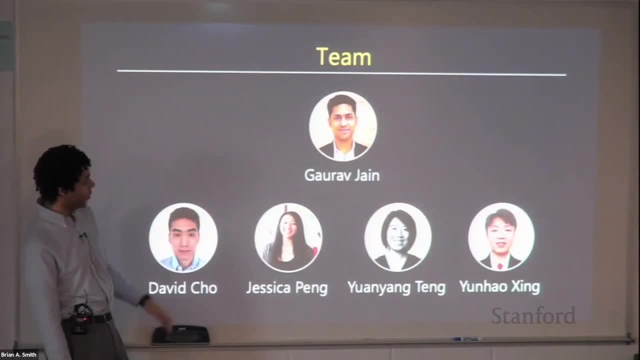 jane is leading a project which we're jane is leading a project which we're called calling wearable vision. he has a called calling wearable vision. he has a called calling wearable vision. he has a computer vision background, working with computer vision background, working with computer vision background, working with several- uh, you know, really talented. 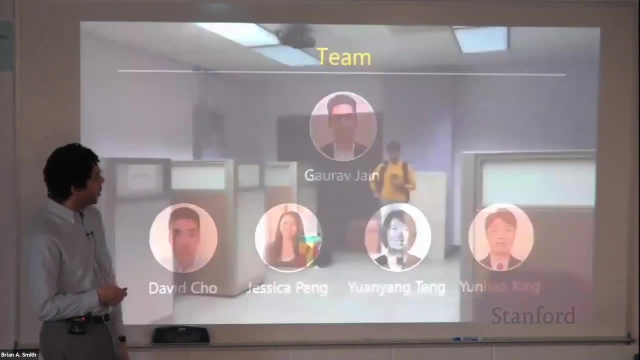 several- uh you know- really talented, several- uh you know really talented- undergrads and master students. undergrads and master students, undergrads and master students: um, in which uh a user can actually um, in which uh a user can actually um, in which uh a user can actually create their own maps by wearing a. 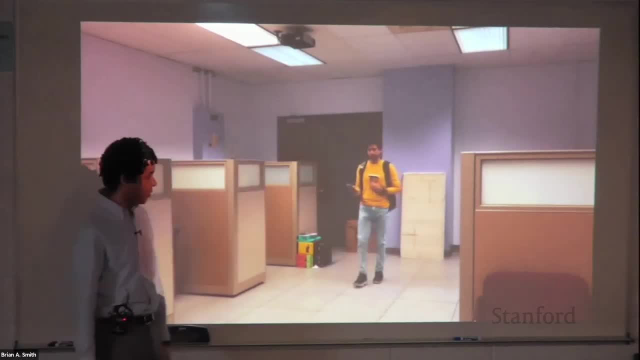 create their own maps by wearing a. create their own maps by wearing a little camera harness- little camera harness, little camera harness. so garov is a first year phd student. so garov is a first year phd student. so garov is a first year phd student. so this is still pretty early work. but 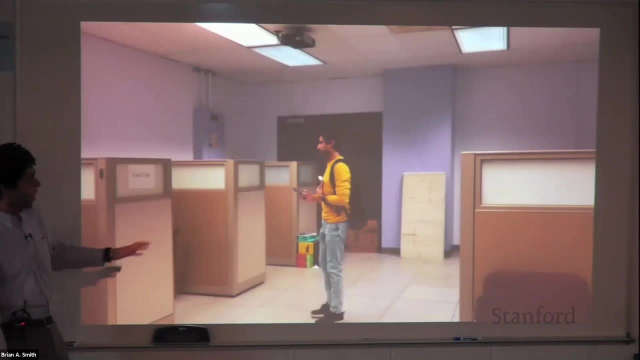 so this is still pretty early work. but so this is still pretty early work, but essentially we're um, essentially we're um, essentially we're um using slam, and uh, the idea is like: how do using slam? and uh, the idea is like, how do using slam? and uh, the idea is like: how do we? 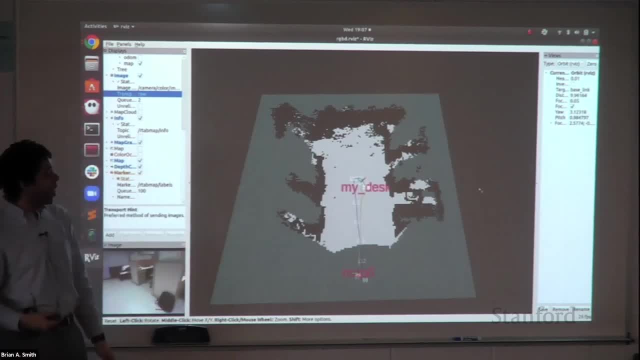 we. we give blind users um the power to take. give blind users um the power to take. give blind users um the power to take navigation and like map making into navigation and like map making into navigation and like map making into their own hands, rather than relying on. 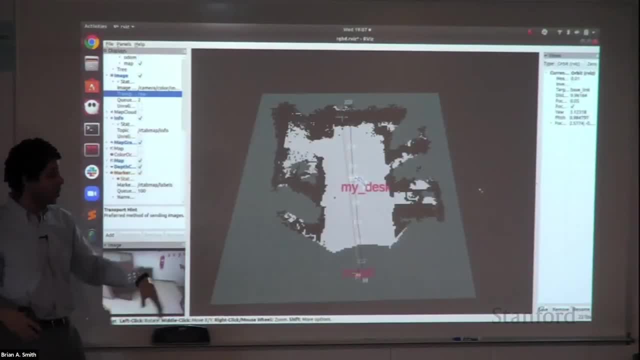 their own hands rather than relying on their own hands, rather than relying on building owners, building owners, building owners- to install maps and bluetooth hardware, to install maps and bluetooth hardware, to install maps and bluetooth hardware, and all of that themselves, and all of that themselves and all of that themselves? how can blind users take map making and 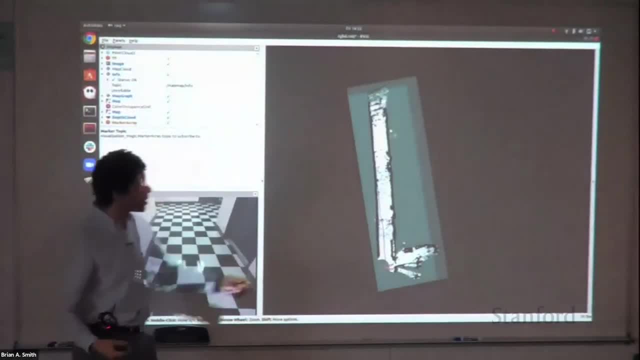 how can blind users take map making and how can blind users take map making and localization into their own hands? localization into their own hands. localization into their own hands by creating their own spots, um, and by creating their own spots um, and by creating their own spots um, and and making slam work for humans and not. 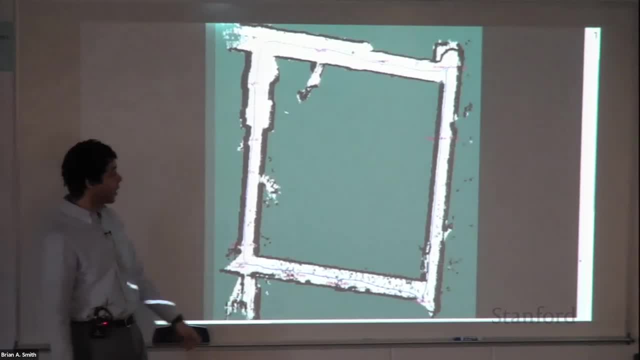 and making slam work for humans and not and making slam work for humans and not just robots at factories- right, there are just robots at factories, right. there are just robots at factories, right. there are a lot of human factors and ui issues, a lot of human factors and ui issues. 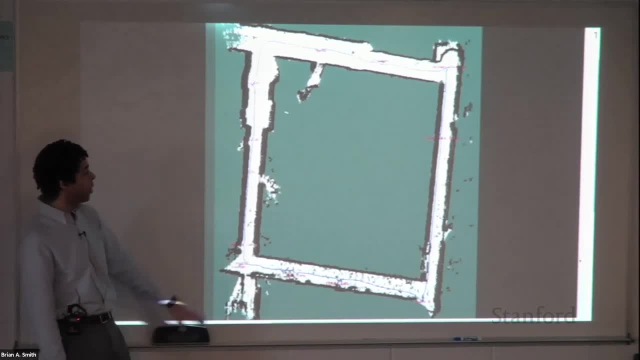 a lot of human factors and ui issues, especially if the user is blind. how do, especially if the user is blind, how do, especially if the user is blind, how do they actually control? they actually control, they actually control. how do, how do you build this kind of? how do, how do you build this kind of? 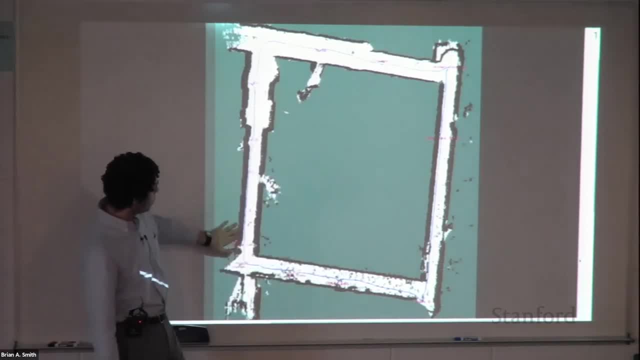 how do, how do you build this kind of system? so this is uh um system. so this is uh um system. so this is uh um, uh my, you know this is part of a floor. uh, you know this is part of a floor. uh, you know this is part of a floor. um near my office, um gaurav, i think. just 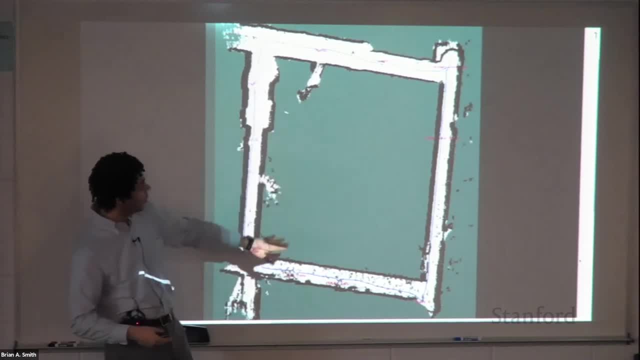 um near my office um gaurav. i think just um near my office um gaurav. i think just did one loop and formed this map. did one loop and formed this map. did one loop and formed this map and created these little spots along the. and created these little spots along the. 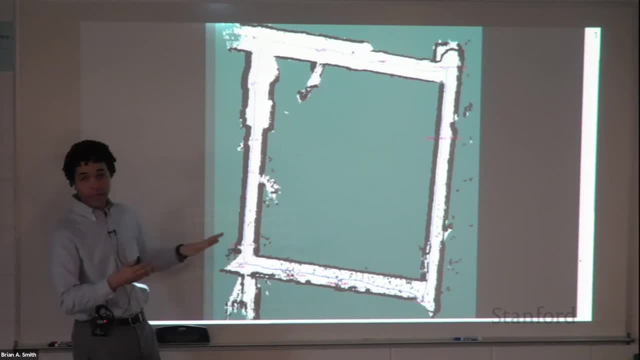 and created these little spots along the way. we're also going to way, we're also going to way, we're also going to. we're looking into this idea going into. we're looking into this idea going into. we're looking into this idea going into social computing of sharing maps. 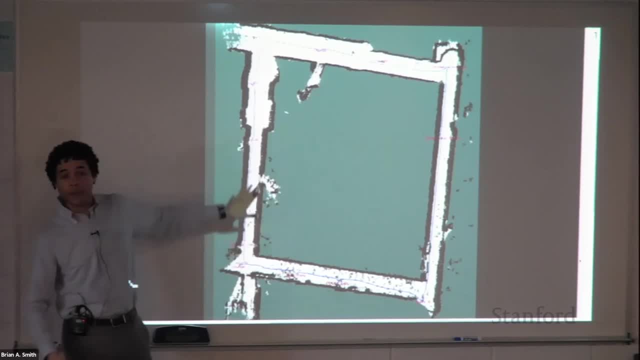 social computing of sharing maps, social computing of sharing maps. so if i, for example, created a map of so, if i, for example, created a map of so, if i, for example, created a map of my office building, and then i have a my office building and then i have a. 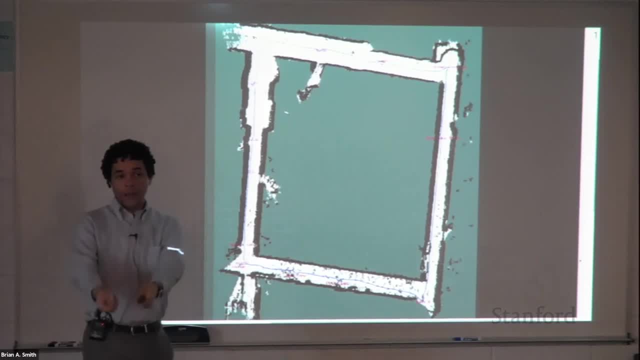 my office building and then i have a visitor, visitor, visitor who's blind. i can say, oh, i have a map who's blind. i can say, oh, i have a map who's blind. i can say, oh, i have a map for that, for that, for that being right, or maybe there's kind of an 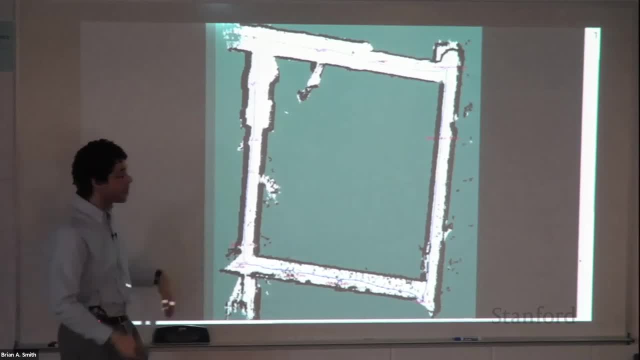 being right, or maybe there's kind of an being right, or maybe there's kind of an open street map, open street map, open street map or a project sidewalk for this sort of, or a project sidewalk for this sort of, or a project sidewalk for this sort of thing. 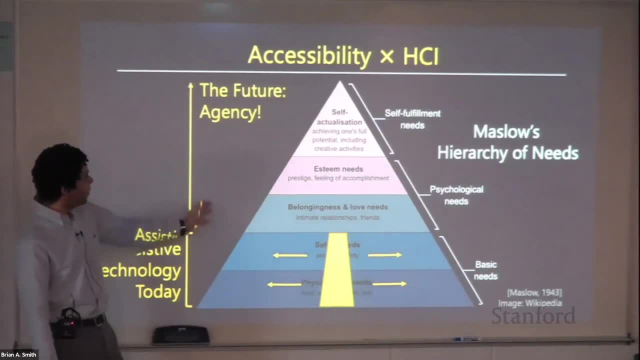 thing thing. okay, and one last word. this is my last. okay, and one last word. this is my last. okay, and one last word. this is my last thing thing thing about this slide, about how about this slide about? how about this slide about how accessibility relates to hci- that i'd. 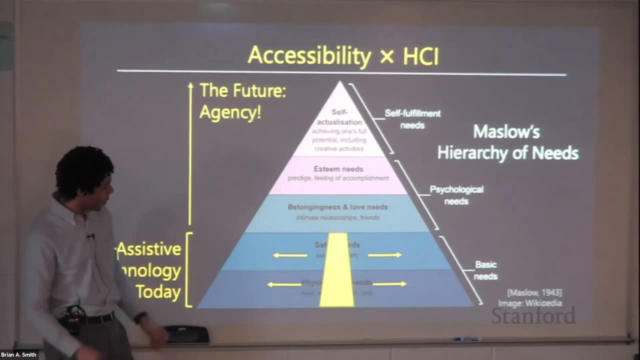 accessibility relates to hci. that i'd accessibility relates to hci that i'd like to say, like to say, like to say um accessibility. i feel is like very, um, um accessibility. i feel is like very, um, um accessibility. i feel is like very, um central to hci, because it forces us to 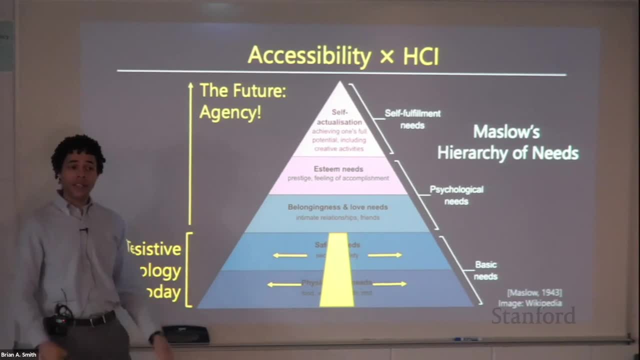 central to hci, because it forces us to central to hci, because it forces us to think, think, think of what's really necessary and what's of what's really necessary and what's of what's really necessary and what's really needed, really needed, really needed um in the systems that we build right. 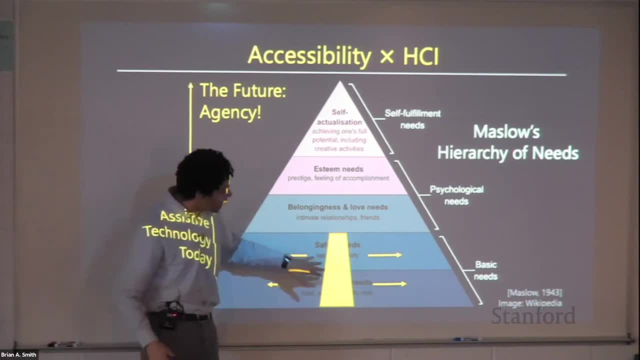 um in the systems that we build right, um, in the systems that we build right, like what is the core, like what is the core, like what is the core? components- um, we, we have to stay components. um, we, we have to stay components. um, we, we have to stay grounded when we think about. 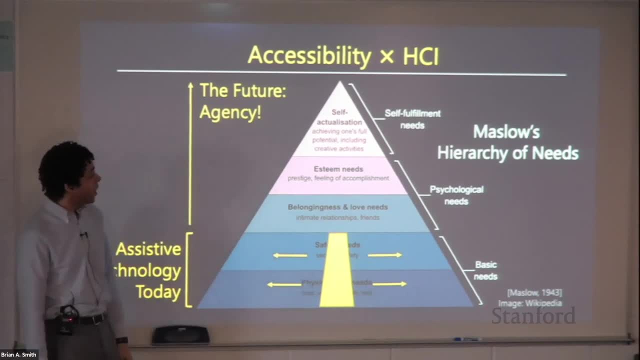 grounded when we think about grounded, when we think about accessibility issues, um, but going accessibility issues, um, but going accessibility issues, um, but going forward, forward forward, uh. i think that, like you know, we should, uh, i think that, like you know, we should, uh, i think that, like you know, we should be thinking in terms of not just 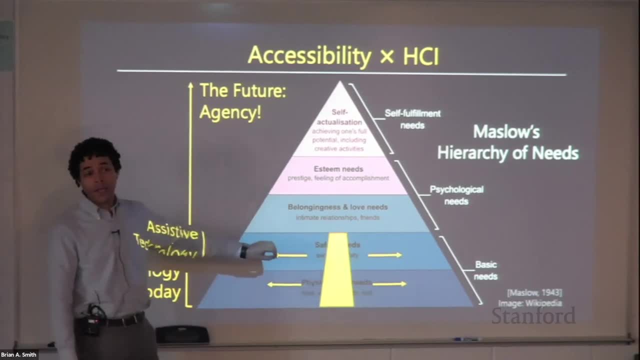 be thinking in terms of- not just be thinking in terms of not just what's really needed, um, but in terms of what's really needed, um, but in terms of what's really needed, um, but in terms of equity, equity, equity, like. how can we like in all of these? like, how can we like in all of these, like, how can we like in all of these great systems that we build great systems, that we build great systems, that we build um, how do we make sure that we're not um, how do we make sure that we're not? 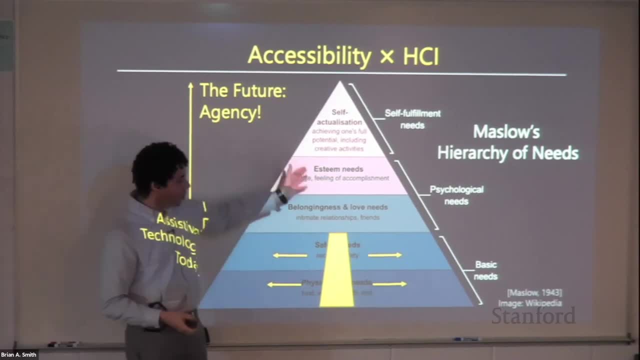 um, how do we make sure that we're not just making life possible for other, just making life possible for other, just making life possible for other people? people, people- um but equitable for other people. um but equitable for other people. um but equitable for other people. okay, so thank you so much um for. 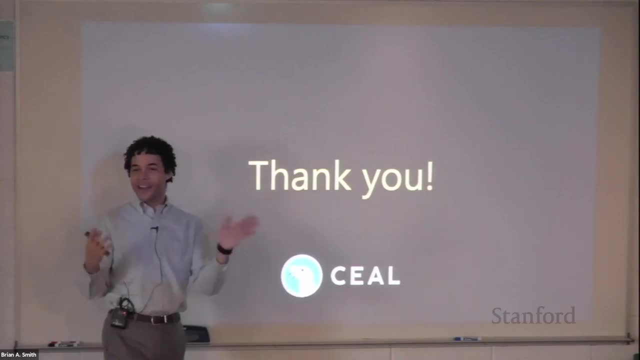 okay. so thank you so much um for okay. so thank you so much um for listening and uh happy to take any listening and uh happy to take any listening and uh happy to take any questions, questions, questions. sorry for the high flex classroom, um. sorry for the high flex classroom, um. 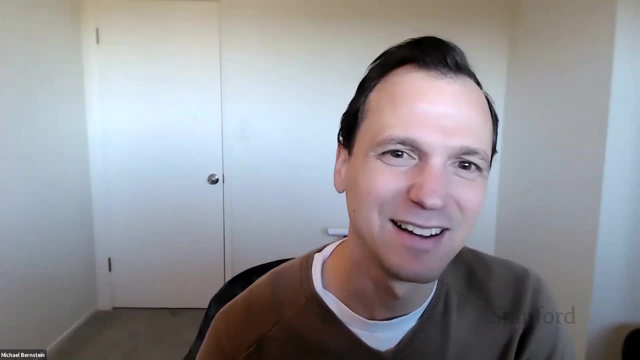 sorry for the high flex classroom. um, you know audio issues. thank you, brian, you know audio issues. thank you, brian, you know audio issues. thank you, brian. no worries, no worries, no worries. the joys of of uh zoom, and yeah, brave. the joys of of uh zoom, and yeah, brave. 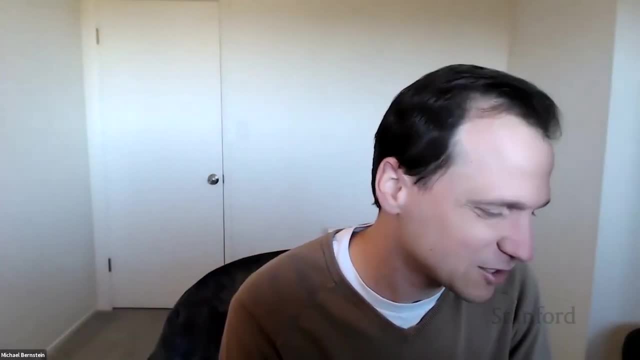 the joys of of uh zoom and yeah, brave new world, new world, new world. uh. thank you, brian. uh the uh. so this is a uh. thank you, brian, uh the uh. so this is a uh. thank you, brian, uh the uh. so this is a good a chance for. 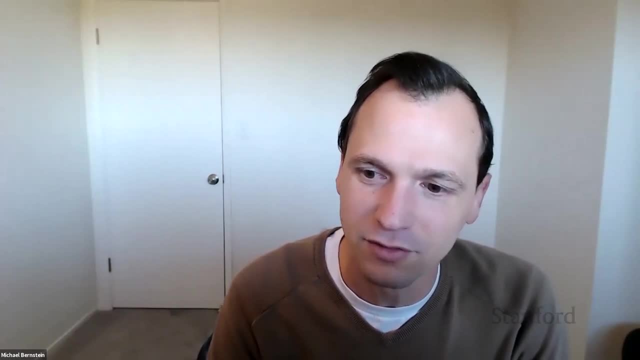 good a chance for. good a chance for for questions: the uh. there's a form for questions: the uh. there's a form for questions: the uh. there's a form that i've linked to in the zoom chat that that i've linked to in the zoom chat that. 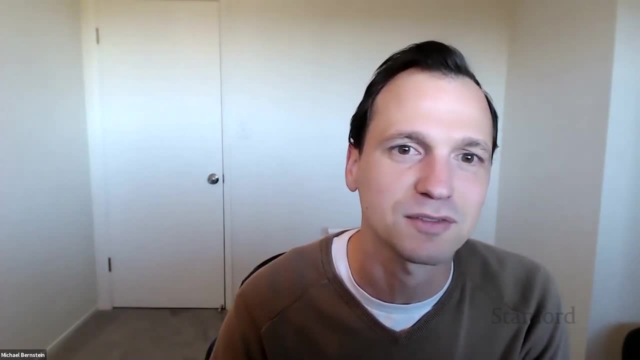 that i've linked to in the zoom chat that you can ask. you can ask, you can ask panelists. feel free to just go ahead, and panelists feel free to just go ahead, and panelists feel free to just go ahead and unmute yourselves. unmute yourselves. 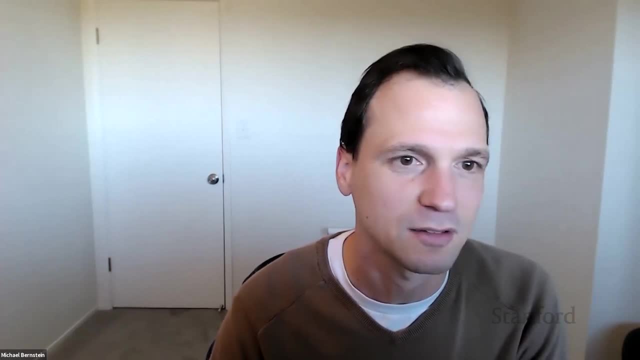 unmute yourselves and and dive in um. did you want to start? and and dive in um. did you want to start? and and dive in um. did you want to start? and then while i curate the questions, and then, while i curate the questions, and then while i curate the questions from the, from the, from the form. sure, if 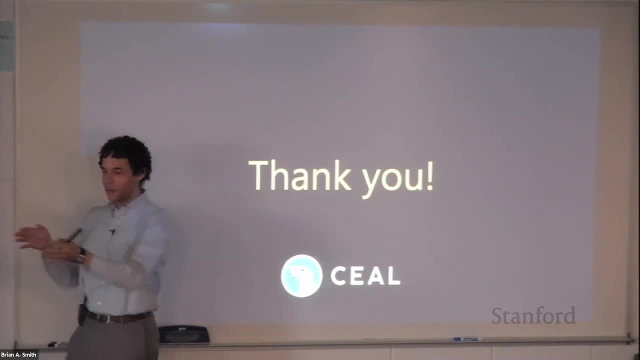 from the from the from the form sure if? from the from the from the form, sure. if i look this way, this is my view of the. i look this way, this is my view of the. i look this way, this is my view of the computer. i can see the gallery here, so 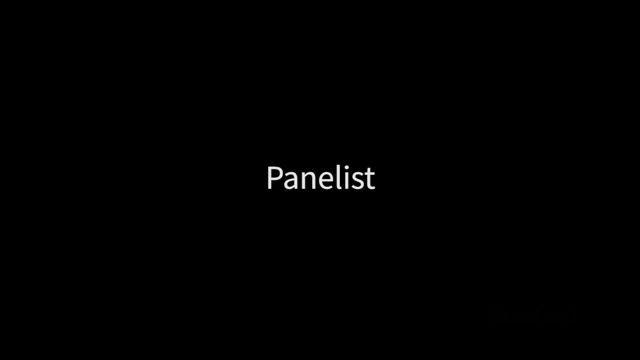 computer, i can see the gallery here. so, computer, i can see the gallery here. so, yeah, yeah, yeah, okay cool um, i was a little curious about okay cool um, i was a little curious about okay cool um, i was a little curious about how you're thinking about play testing. 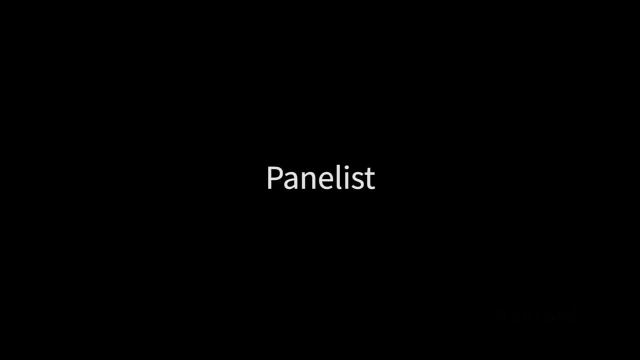 how you're thinking about play testing, how you're thinking about play testing, um so, um so, um so. normally you do many, many, many rounds. normally you do many, many, many rounds. normally you do many, many, many rounds um, but of course it can be difficult to um, but of course it can be difficult to bring in participants. so i was wondering. 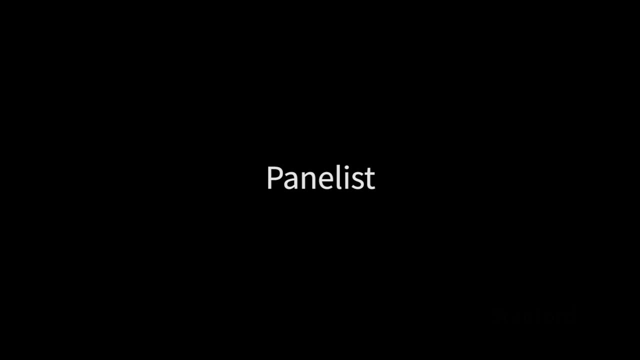 bring in participants. so i was wondering: bring in participants. so i was wondering just sort of, just sort of, just sort of: do you do you? do you do it yourself? do you wear a blindfold? do it yourself, do you wear a blindfold? do it yourself, do you wear a blindfold? you know, because i saw that you used. 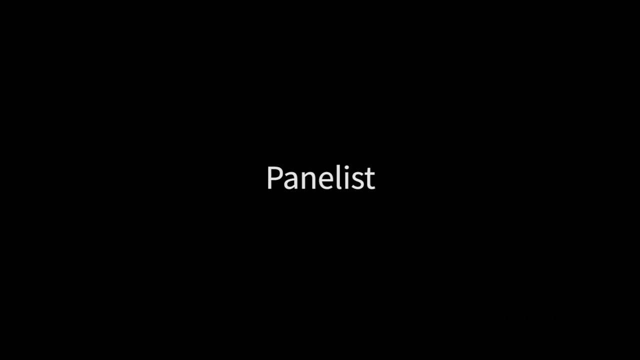 you know, because i saw that you used. you know because i saw that you used them in the last cycle, but that's really them in the last cycle, but that's really them in the last cycle, but that's really kind of late, kind of late, kind of late. yeah, let me, yeah, um, thanks for the. 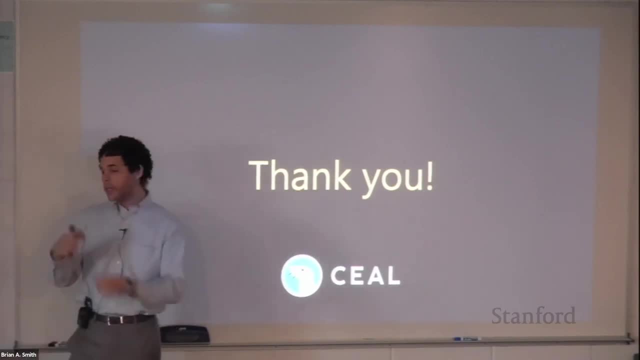 yeah, let me, yeah, um thanks for the. yeah, let me, yeah, um thanks for the question. yeah, let me actually make that question. yeah, let me actually make that question. yeah, let me actually make that clear, so um during development, and like clear, so um during development and like 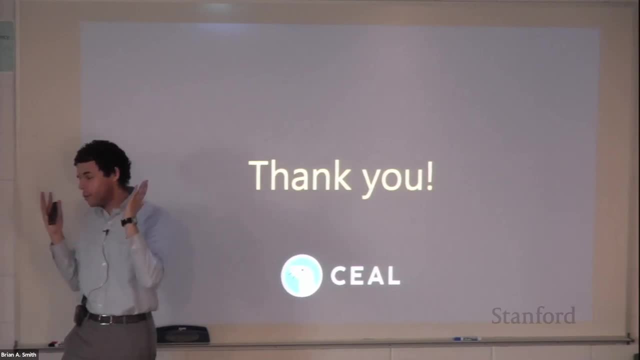 clear. so, um, during development, and like you know we're coding something, does it? you know we're coding something, does it? you know we're coding something? does it work like we do wear blindfolds work like we do wear blindfolds. work like we do wear blindfolds ourselves, just to get a basic feel for. 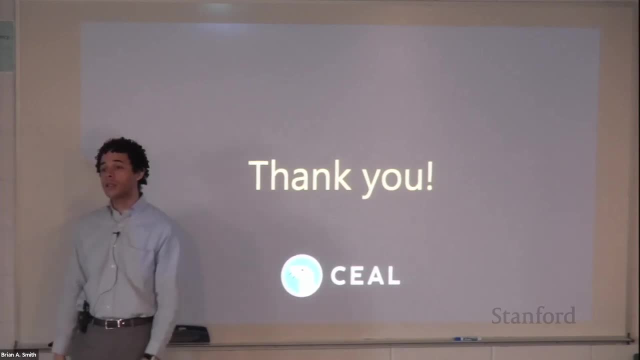 ourselves, just to get a basic feel for ourselves, just to get a basic feel for things. but we also host things. but we also host things. but we also host um uh, students in the lab, uh, um uh. students in the lab, uh um uh. students in the lab uh, particularly people with visual 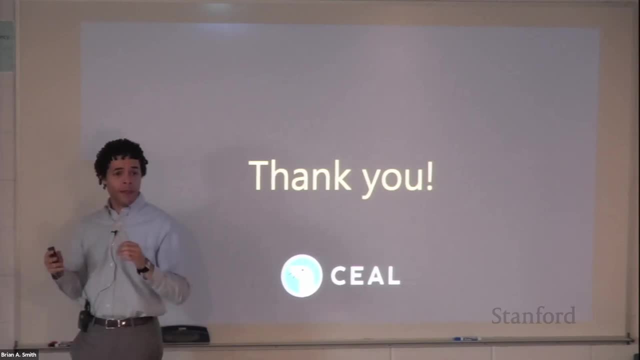 particularly people with visual, particularly people with visual impairments. so i have relationships impairments. so i have relationships impairments. so i have relationships. one of the like, so uh, several different. one of the like, so uh, several different. one of the like, so uh, several different. you know, national organizations for um. 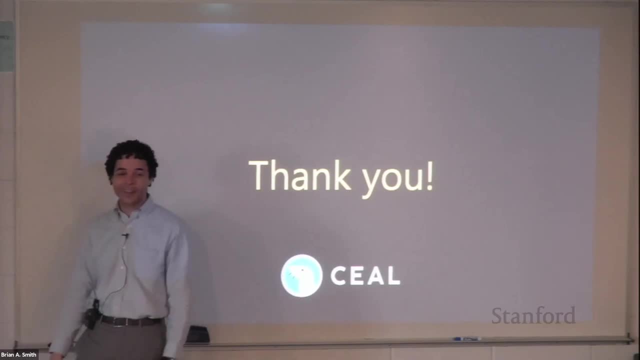 you know national organizations for um you know national organizations for um you know serving blind users. are you know serving blind users? are you know serving blind users? are headquartered here in new york, headquartered here in new york, headquartered here in new york, and so i have relationships with them. 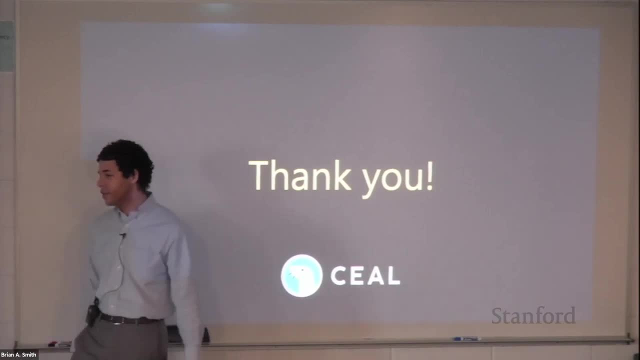 and so i have relationships with them and so i have relationships with them. we have um. you know they sit alongside. we have um. you know they sit alongside. we have um. you know they sit alongside us, us, us. so we co-design with these users. we host, so we co-design with these users, we host. 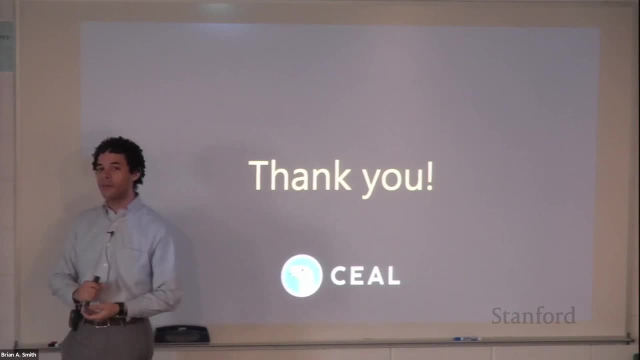 so we co-design with these users, we host over the summer as well, over the summer as well, over the summer as well, and so we've actually learned a lot more, and so we've actually learned a lot more, and so we've actually learned a lot more from them. 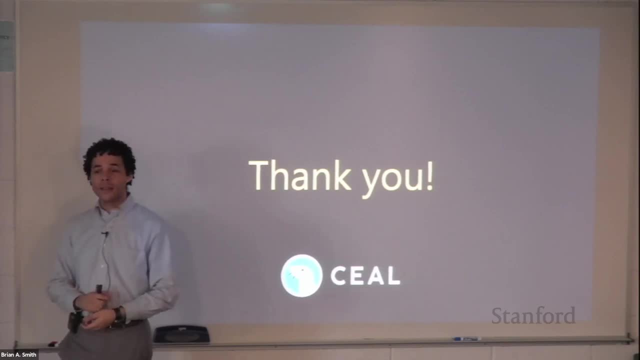 from them, as they've learned from us: um and uh, and, and. so that's how we do things. so, like, when it comes to just like, debugging something, do i think this? you know you're coding, it's night time, um, you know, do i think this is going to work? yeah, we'll wear a blindfold, we'll try it out, and and we've learned. 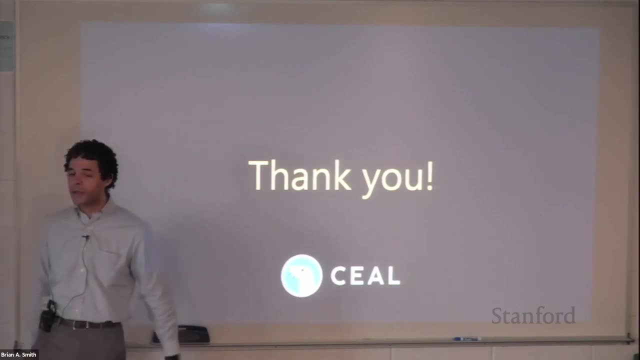 to have some kind of intuition for that, because we've been in this space for a while. um, but ultimately, uh, you know, co-design is what. what does that for us? absolutely, um, and i'm gonna sneak one more in: have you explored echolocation? yes, echolocation, i find it super interesting. um. 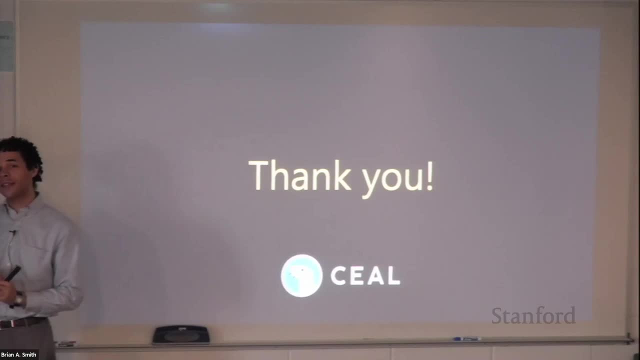 it takes. yeah, like i, i think we um, at least in that that project that i showed about communicating room shape, um, that's actually what we're looking at uh, most and like different and different techniques for, um, generating echolocated sounds. that's actually the space that we're exploring. 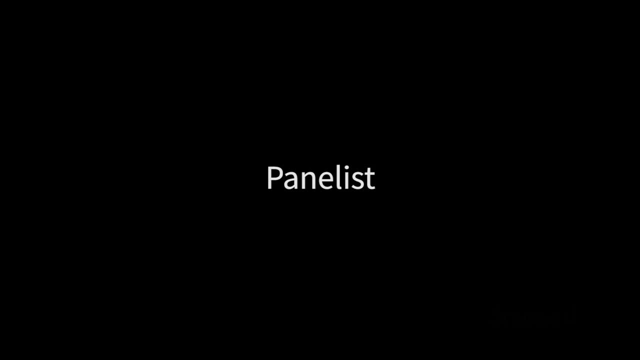 i think, uh, that's really the essex function that we want to tune in to. yeah, i think that's the way that we do um process and uh, and those are the things that we want to do and, um, i think we're going to have to find different ways to do it, um, but but if we can do that, we will. 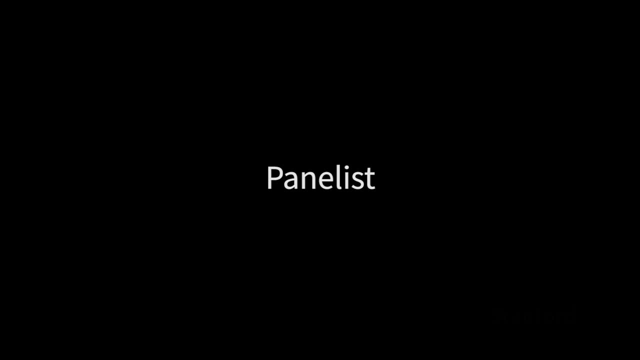 definitely do it, and i think that's the idea that i do, because it's um, it's harder, it's harder to figure out what's going on and um. so i think that's the thing that i think we should be trying to try and, uh, do um, so that's um, and i think it's it's a very good point. i think it's a very good. 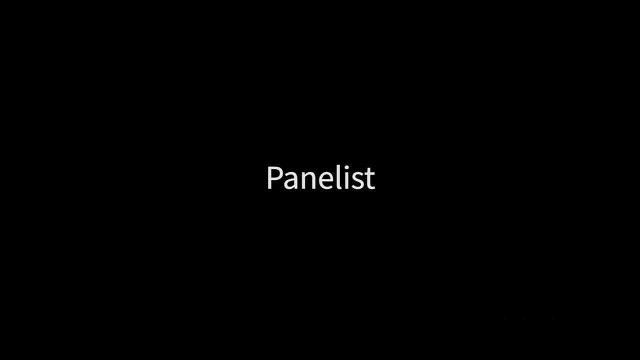 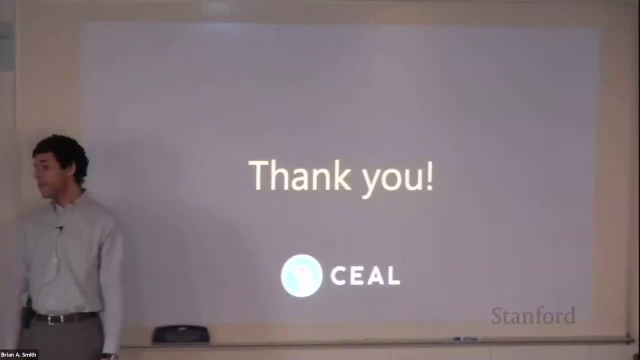 one, um, and i think it's very useful and i think so this is just your time to have your uh uh zoomed and whatnot is also a valuable approach and if you're doing anything with it, yeah, yeah, i'm really interested in touch as well and like, just like you said, a braille sort of thing, um. 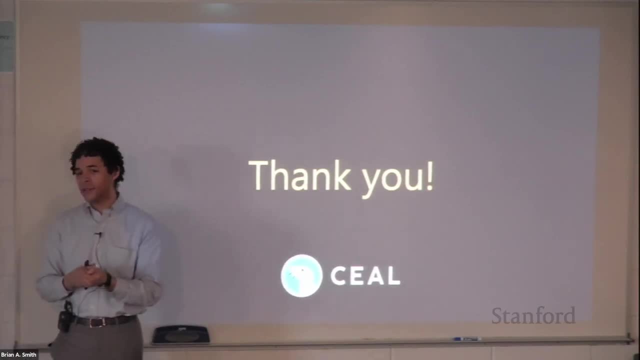 you know, dealing with um limited human sensory resolution. that's a major challenge, um, as well as like speed of of motors, right um actually making the haptics work. i think for general purpose- navigation, real world environments- they'll work just fine for games, especially when the games are very fast. i found that to be a limitation, um in some of the- uh you know. 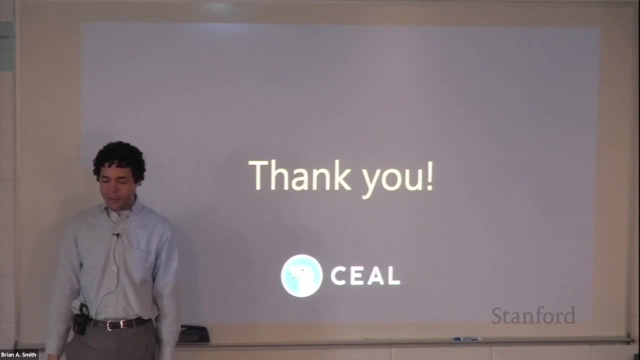 me just like trying things out, um, but i think, um, to be perfectly honest, uh, one of the uh obstacles that we've had is, um, uh, i'm not working with any students, like neither of my phd students and myself, like we, we aren't into hardware ourselves, um, and so that's actually an area that we're. 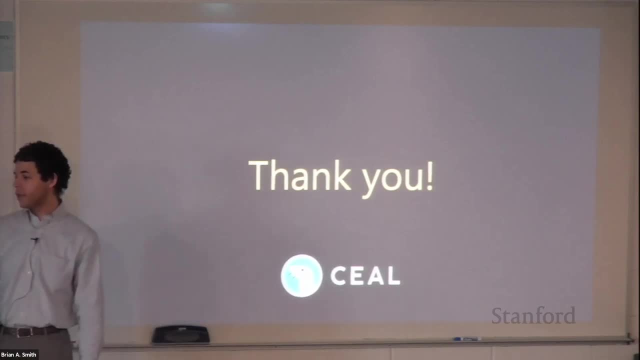 looking to collaborate in um is like, how can we think about haptics, design haptics, uh, and also think about multimodal solutions? um, audio and haptics, um yeah. and then, and especially if there's some general purpose devices that users can buy, like you buy this one thing and it can. 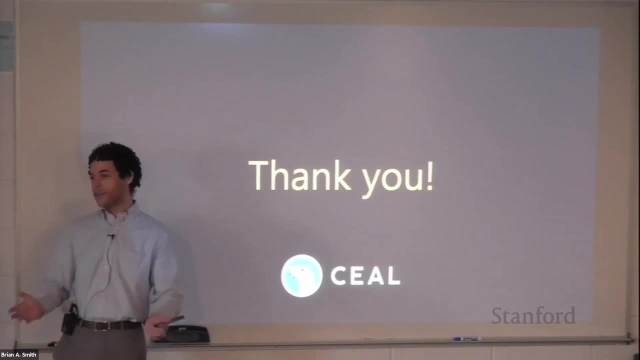 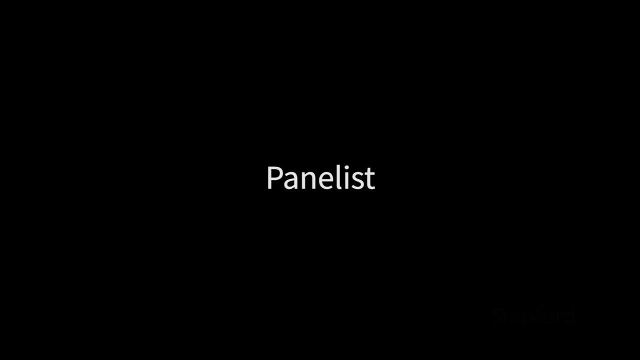 you know, uh, give you a lot in terms of, you know, real world navigation in many contexts. um i i love that idea, cool. um i i have a question. um, in the biofeedback space, um, specifically with the audio path, you decided to complete a new project on a computer screen, when you're creating your own? 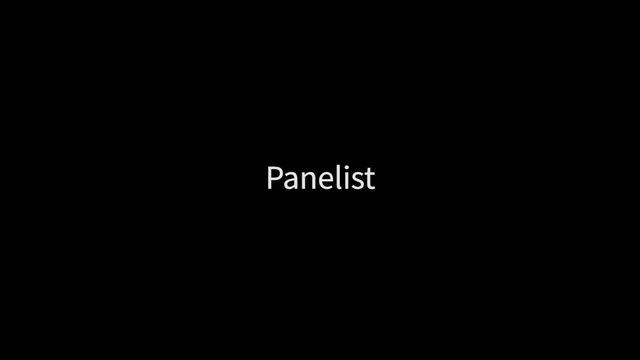 audio-based image it's impossible to create in a virtual environment, right? yeah, um, you're looking at a multi-uniform media solution. um, if you don't have the space to do something like that, you're not going to be able to create a virtual experience. um and um, and then the 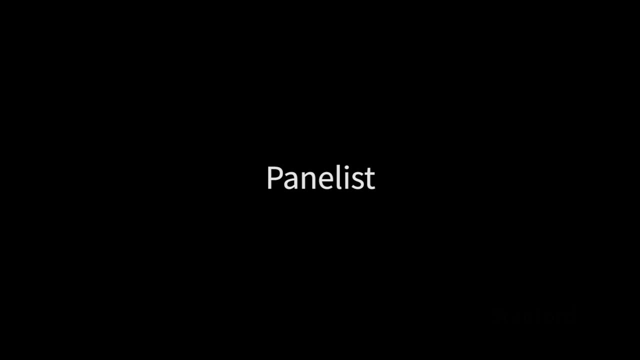 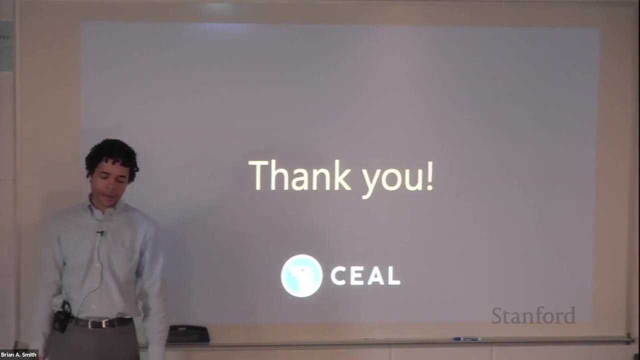 new technology is like i don't know. we're going to be able to do it like a virtual environment. um, you know, some are going to do it that way, but there's a whole range of possibilities and, again, as a person who's growing up in a virtual environment, you're not going to be able to create. 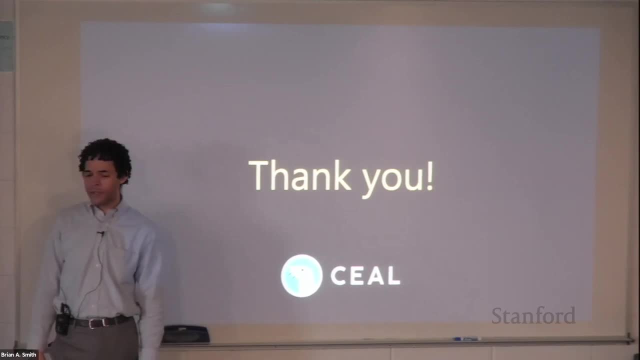 importance of multimodal. I think, like I've found it, just you know a lot of the visually impaired folks that I've worked with and spoken to. some of them are really into sound, Some of them also. many of them actually have hearing impairments, even slight ones that make sound. 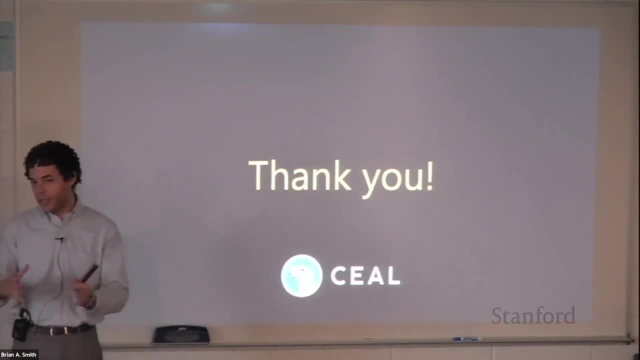 work, you know, much less effectively for them, And they'd really prefer haptics. Some don't like haptics, And so I think that we should be aiming to design solutions in both sound and haptics and allow users to kind of choose and mix and match. Hey, Brian, nice to see you. 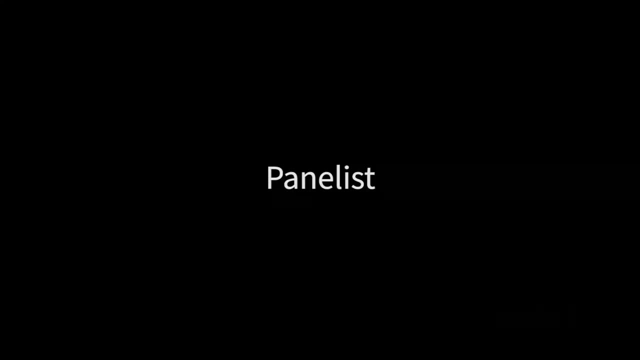 Hi, nice to see you. I had a couple of questions that you know hopefully won't take too much time, so maybe I can do two. The first question I had was whether you've looked at whether these kinds of tools also help sighted people, because it seems to me like having this kind of extra. 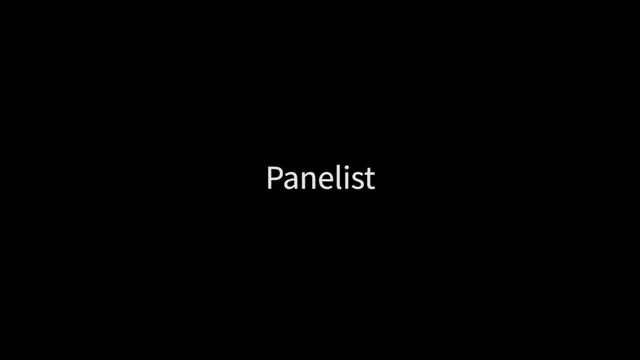 feedback. you know, extra in the case of someone who's sighted would maybe like improve their experience of a game, And I think that's often the case when we design more accessible techniques and tools that actually everyone benefits. So that's just sort of one question, although 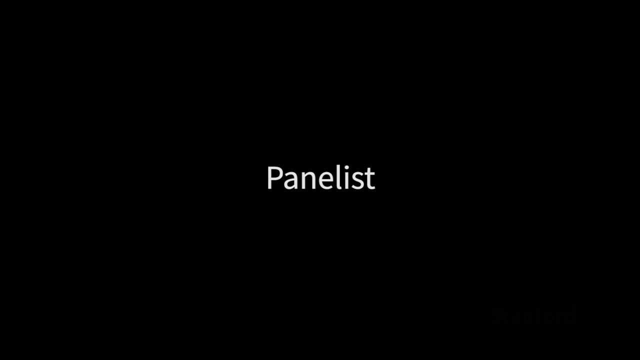 obviously that's not the focus, nor should it be. And the other question I have is how you think about the trade-off or the tension between learning something new that might, you know, provide someone with a skill set that's going to, you know, with the time and 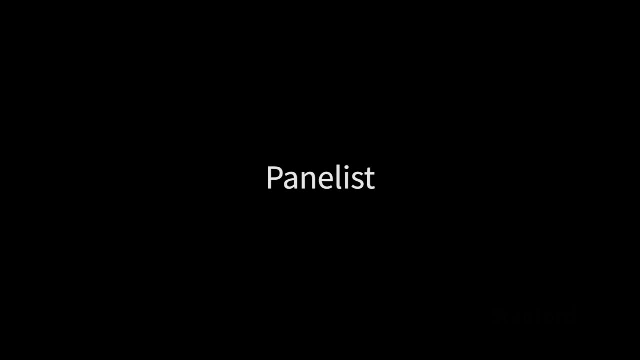 investment to learn is going to provide them a lot of benefit versus sort of speed of adoption, which makes some. you know, in the case of a racing game, it's really cool if someone can, within a few laps, be totally proficient at it, But also, you know, if it's sort of a more advanced 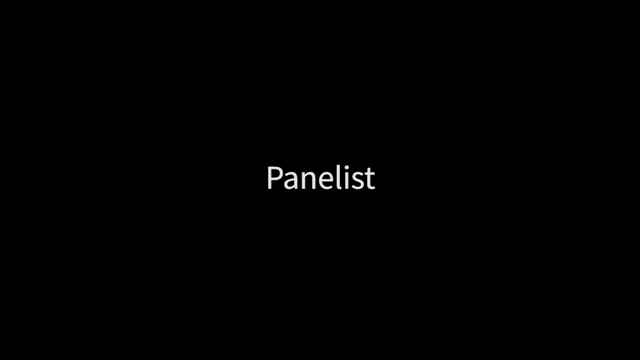 or a more difficult technique. you know, maybe speed of adoption is not really the right metric because it might take longer to pick up but then actually be like more effective in the long term. So I'm just thinking about how you evaluate your tools and think about that trade-off. 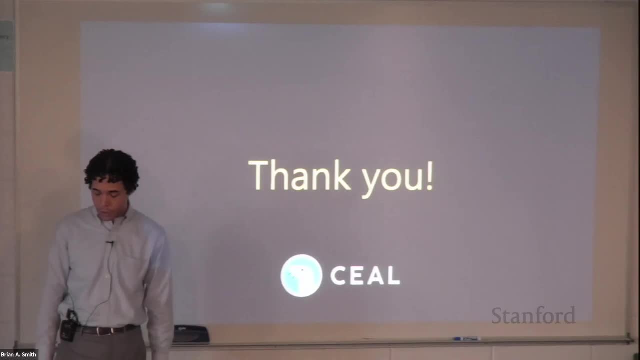 Yeah, so super quick answer to both questions Regarding so. I'll answer the second one. first, about adoption. I think again, that's where personalization is important, right, And that begs for future work, right? So if you have one technique that does more or less, you know well, but you can learn it quickly. 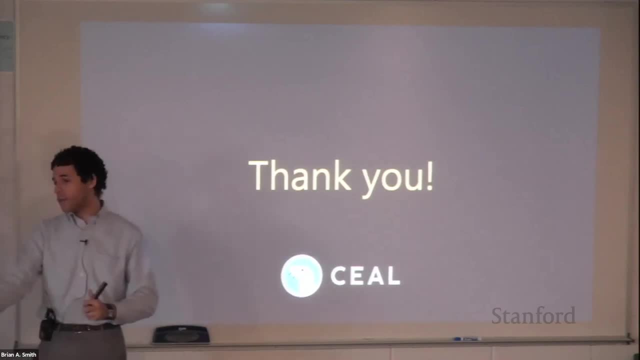 and another one that like works really, really well but it takes a while to learn. is that effort worth the cost? It's kind of like learning a new keyboard layout. That just begs for the research, And so I think that the jury is still out on that. 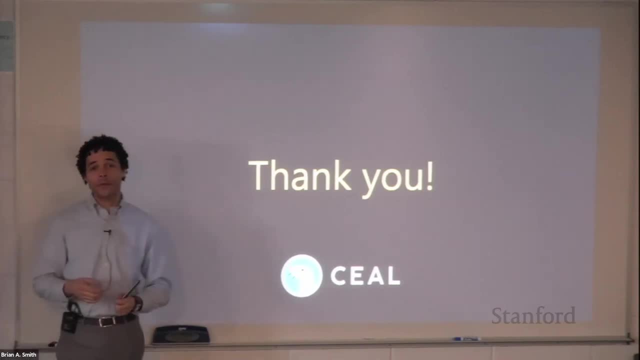 But in terms of your other question, like for you know, people who don't have visual impairments like: how can these systems benefit sighted people? I think about this every time I go to Penn Station downtown and that's actually one of the reasons why I'm really I if I had to choose. 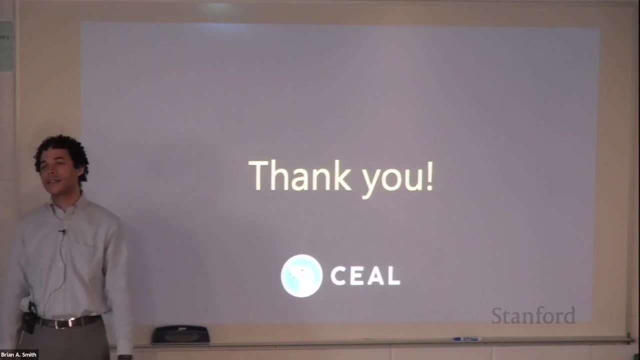 like. I choose audio because it's so easy to incorporate into earbuds And so I think there's a lot of potential to help people who are sighted just with earbuds that they would always like normally have in their ears anyways. 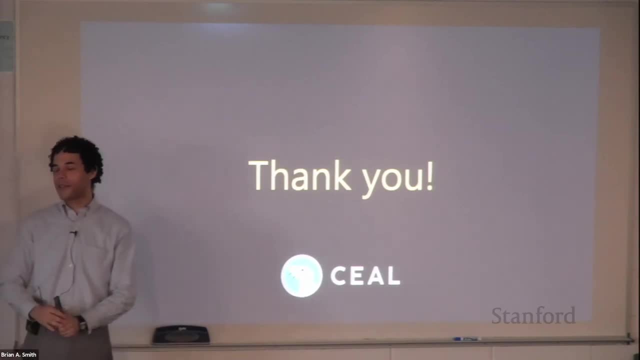 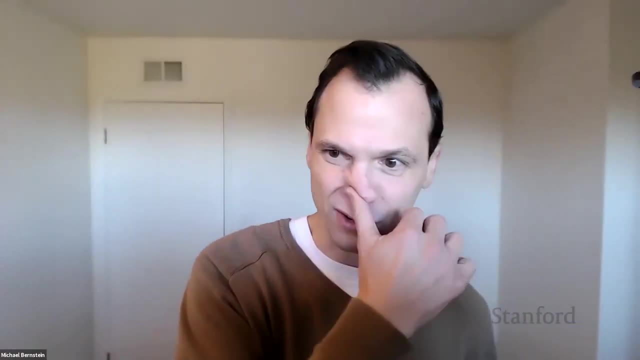 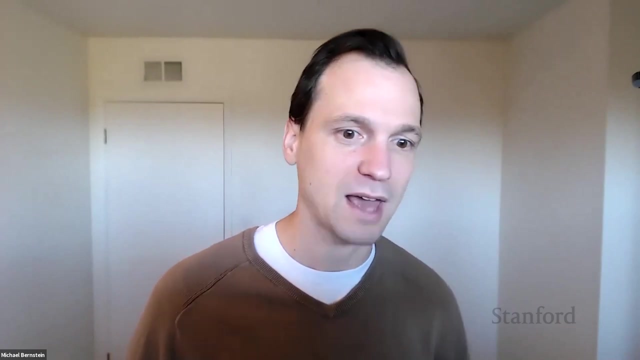 Yeah, Especially grocery stores. That topic comes up all the time as well. All right, And I will be the audience surrogate for the folks who submitted through the form. We definitely had several questions that you've touched on. Most of them had to do with haptic feedback as a channel. 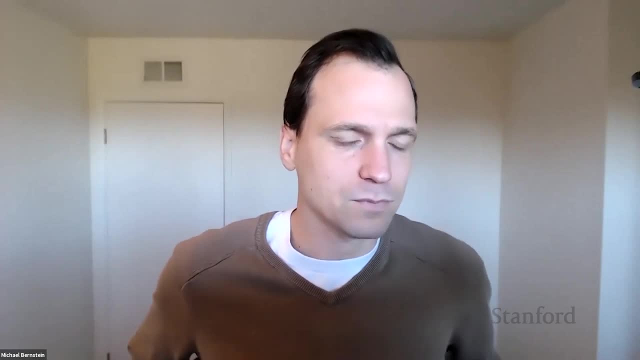 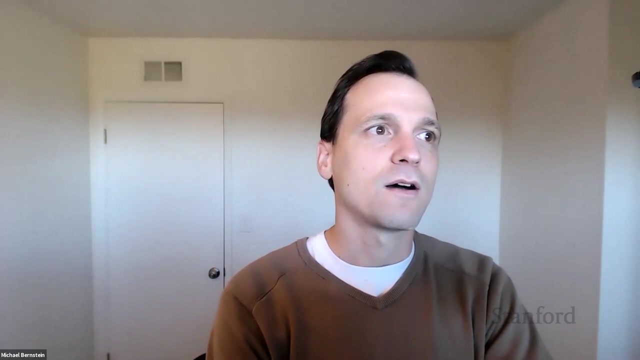 So certainly a lot of excitement around that. Also asked a question about what are the most difficult genres to make accessible? How do you overcome these problems? Maybe a way to conceptualize that question would be to ask you know what seems on the possibility horizon. 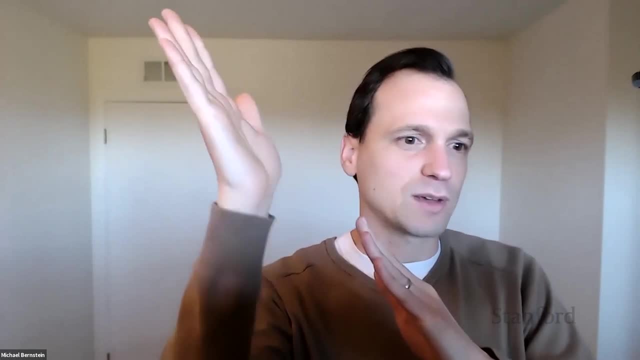 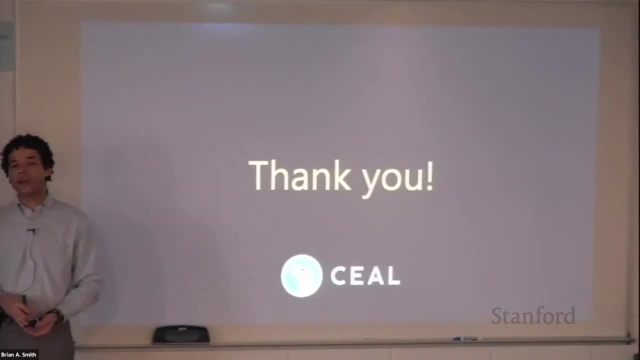 And then what kinds of experiences and fulfillments seem. you know capital H hard that. you know that there are fundamental blockers there, that you see, Yeah, So the regarding the blockers, like I think, if you go, if you look back to that, you know, 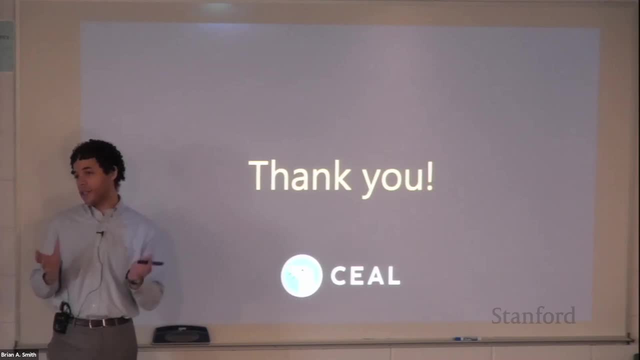 the eight types of fun slide, one type was sensation. games is sense pleasure, Any games that really hinge on sensation, that's capital H hard. And so you know: Color Crush, Candy Crush, all of those variants of the same type of game, right, 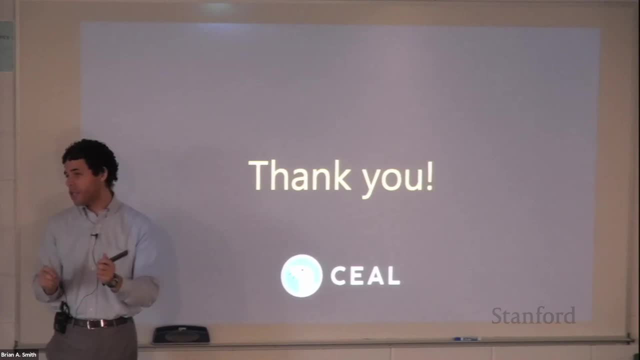 They, those, those are mostly submission, but the mechanic of quickly identifying swappable gems or candies or whatnot is highly, highly highly visualized. Yeah, Yeah, Yeah, And, and so that I would say that's getting closer to capital H hard. 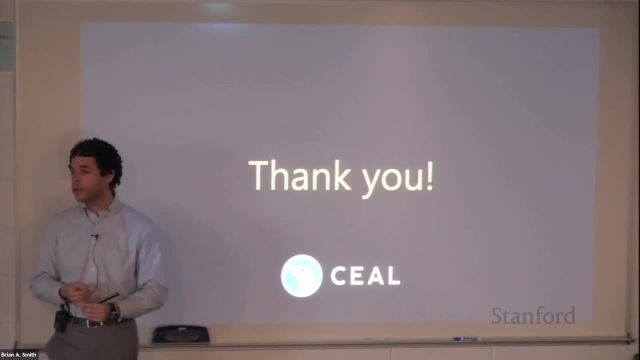 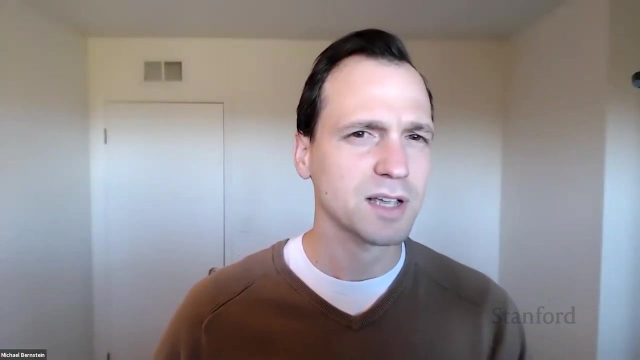 First person shooters- I think very doable- Platforming games- time pressure is so immense. But I think the the real obstacle is the games that that rely on sensation. And does this? some of these examples seem to be because our visual system often operates in parallel.